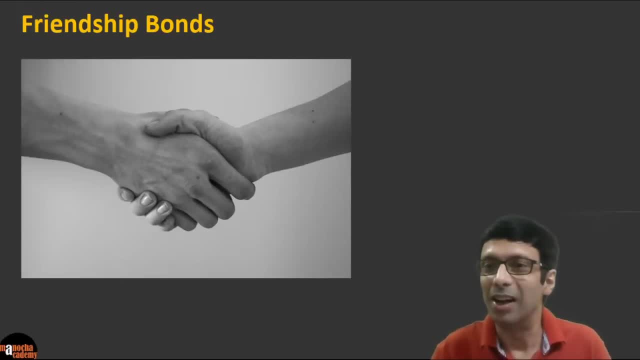 do? we make friends? So that we can have fun, you know, joke around with each other, and these friends help us and support us throughout our lives. So, just like we have friendship bonds, we are going to talk about the friendship bonds of atoms. 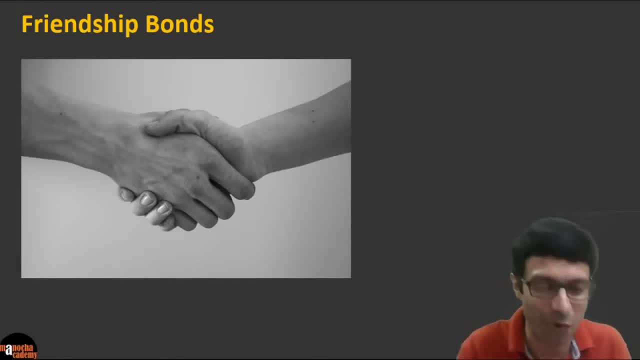 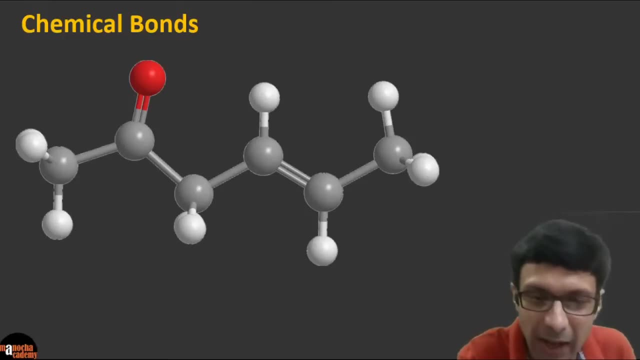 which are chemical bonds. So let's go ahead and dive right into it. So, guys, as you can see in the picture here, can you see there are different types of atoms here, right? And if I go ahead and mark out some of the atoms, so these atoms are representing, the white ones are hydrogen atoms. 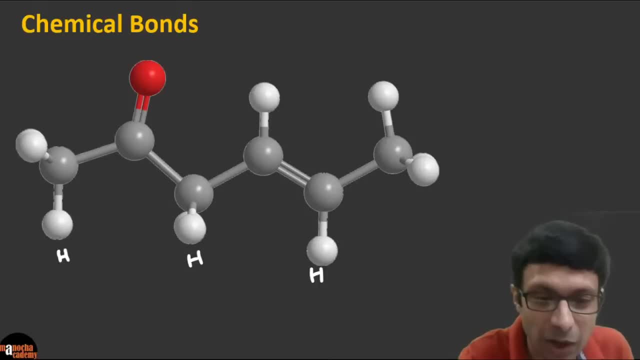 let's say, okay, the white guys, the dark atoms here, right, The grayish ones are the carbon atom, okay, And these, the red one here is the oxygen atom, okay, And can you see that there are these sticks or things that are bonding these atoms? Can you see the bonds here, right? So these 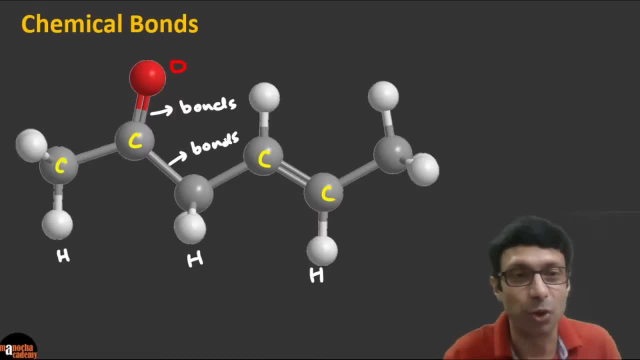 we call as chemical bonds. right, So you know that bonds are holding the atoms together. okay, And these are what are known as chemical bonds. So atoms combine with each other to form molecules. right, So the force of attraction which holds the, which holds the molecule together, is known as. 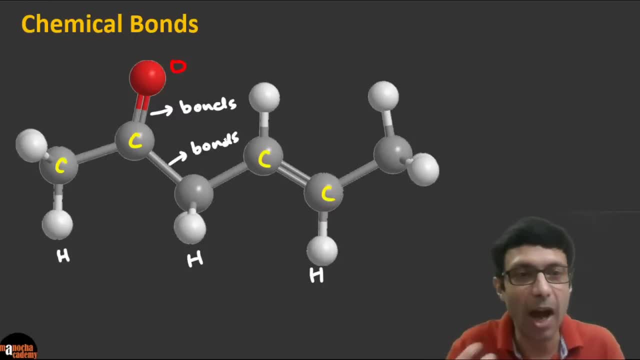 chemical bonds. Now let me ask you: why do atoms form chemical bonds? So we discussed about our friendship bonds, right? So, guys, can you tell me why do atoms form chemical bonds? right? And some of you are asking: what is the difference between an atom and molecule? You know that a 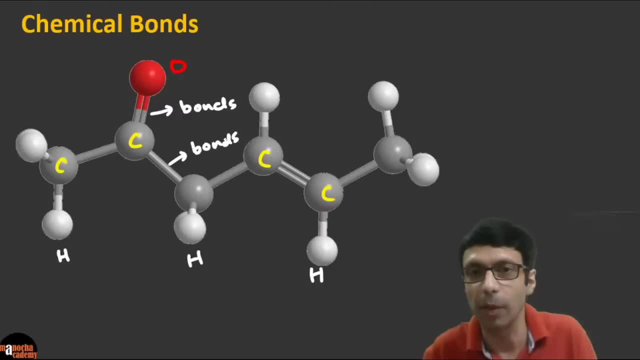 molecule, it can consist of one atom, like monoatomic molecules, right? And some of you are asking: why does a molecule have two or more molecules? Why do atoms form different molecules? But usually a molecule contains two or more atoms It could come for from the same element or it. 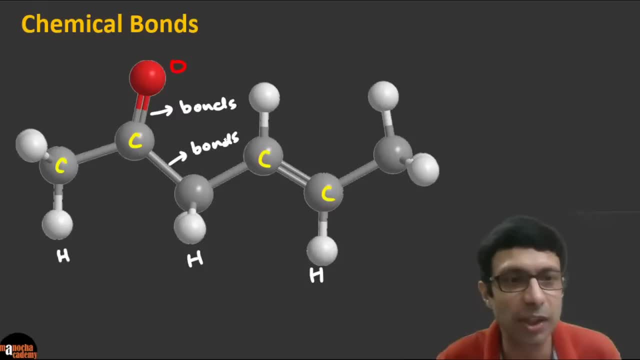 could be from different elements. So very good, I see Suresh has the right answer here, Vinay has the right answer. excellent. Science is like for stability guys: excellent, excellent. So why do atoms combine? very important concept in chemistry. Chemical bonds are formed for stability, okay, So 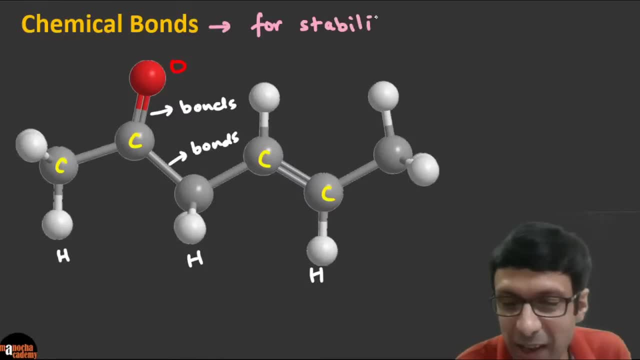 just like everyone wants a stable life. a stable life. so you can see, if you combine atoms, you can job. even atoms want a stable life. they want stability and that is why they form chemical bonds, so that the resultant molecule is stable and each atom in it. 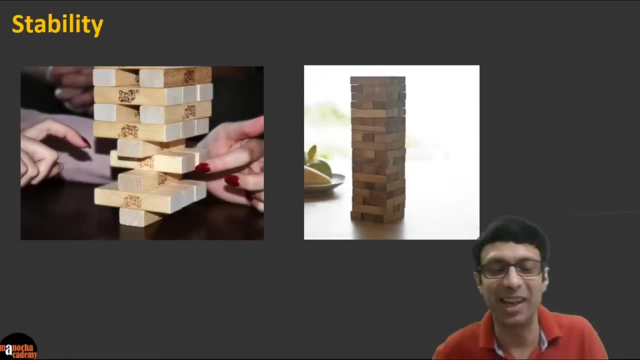 is stable. okay, and guys, have you played this Jenga game before? so how many of you played Jenga? so I'm sure you've seen this right. so can you tell me which Jenga arrangement here is stable and which one is unstable? so can you see. 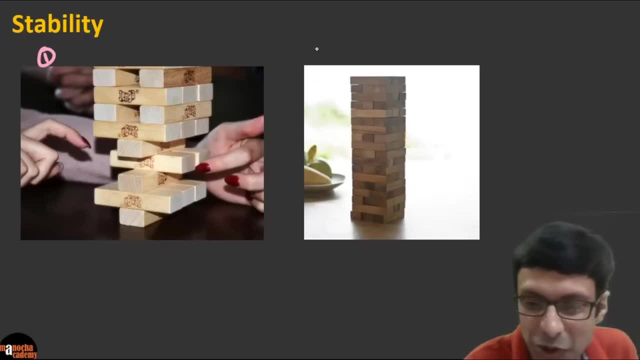 these pictures, guys, right so on your screen. so this is picture number one and picture number two. and if you played the Jenga game, I also enjoy playing Jenga, and so here can you see that this is a very unstable arrangement. can you see that right? because these wooden blocks are going to fall down right and very 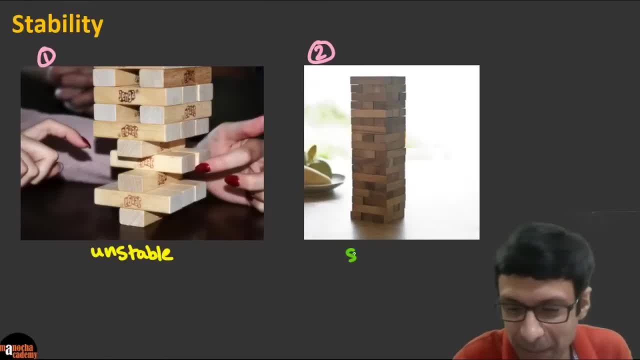 good. so the two is a nice stable arrangement. can you see, right? so this is for Jenga, right? or you know, like a building or a set of bricks, what is stable, what is unstable, what is unstable, what is stable, what is unstable, what is unstable? you have an idea right. or if you take a cone, you put it on its base, it's stable if you. 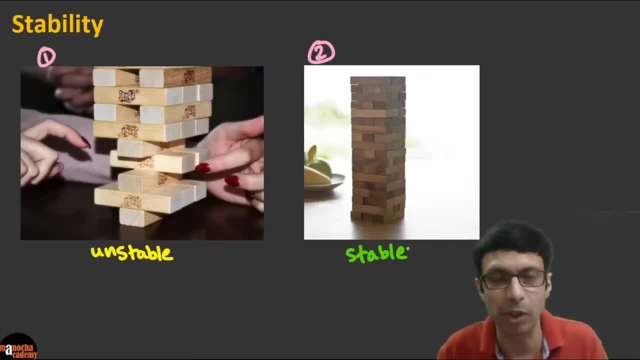 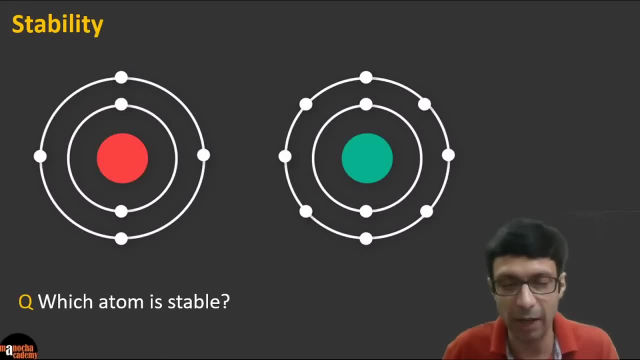 invert it. it's unstable, right. but what is stability in chemistry, right? what is the meaning of stability? it's very important to discuss that. so, guys, i have two pictures of atoms here, right? so i've got. let's again number them. this is, let's say, atom number one, okay, and this is atom number two. so 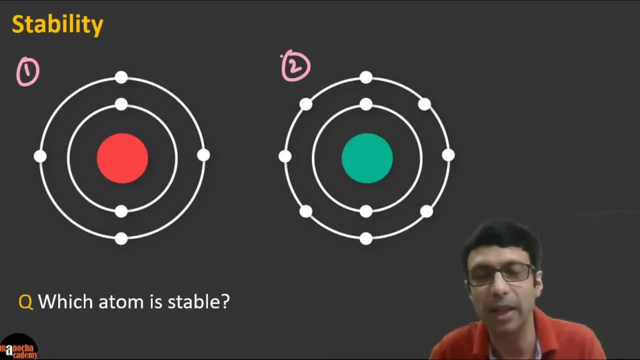 based on your chemistry knowledge, can you tell me which atom is stable? okay, and which atom, or we should say which atom- is more stable than the other? so come on, i want all of you to try here, excellent, excellent guys, and it's great to see the response- and, guys, if you haven't hit the like. 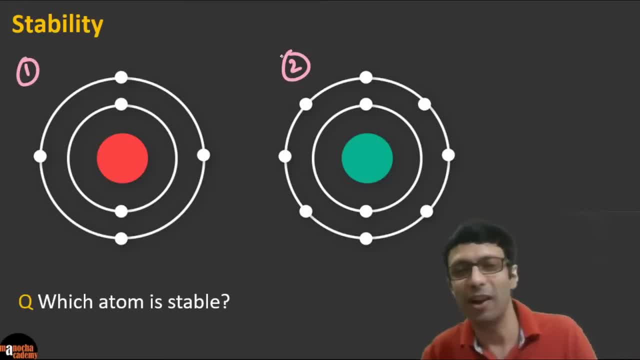 button. please hit the like button right now and do share it with your friends. thanks, guys, for clicking the like button and do share it out with your friends also. great, OK, so lot of you. i'm seeing. very good, you're seeing. the correct answer is the second atom. 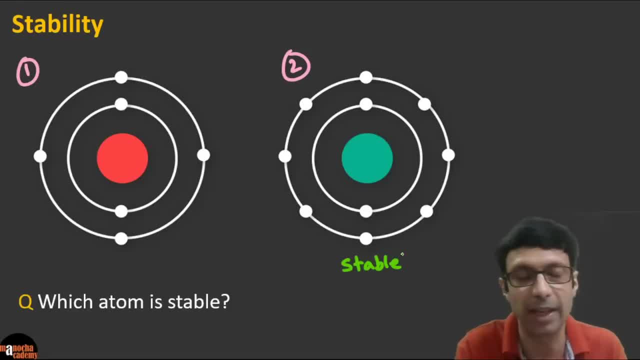 is stable, and the first more stable, we can say, than the first one. now let's discuss why. what is special about the atoms here? so can you see in this picture i've shown electron configurations right, so this is actually a carbon atom here. okay, so the first one is a carbon atom, so that is its. 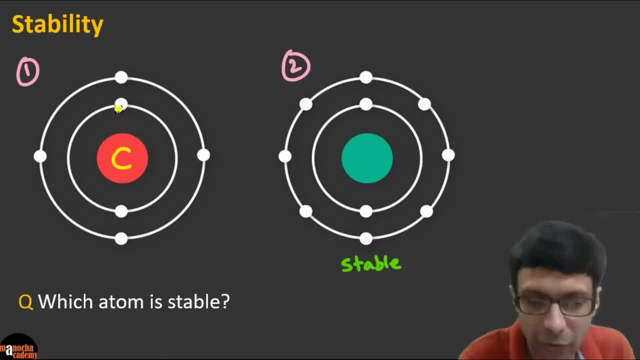 nucleus. and, guys, can you see the carbon, you know, has six electrons, so one, two, three, four, five and six. everybody see that on your screen and this atom, right? so, guys, do you know which atom this one is? and it has eight electrons, one, two, uh sorry, ten. one, two, three, four, five, six, seven. 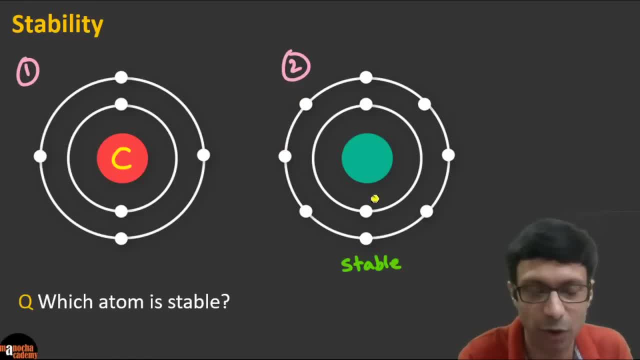 eight, nine, ten. okay, right, it has ten electrons here. carbon it has six electrons. so we can write down: its electronic configuration of carbon is two comma six, okay, and the electron configuration of this guy. let's write it down. okay, the electron configuration of this guy is going to be: 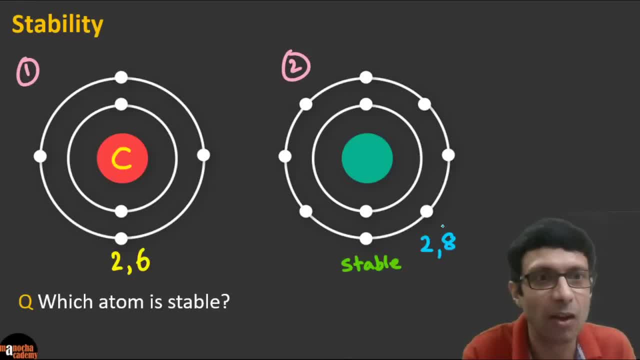 two comma eight. so do you know which atom is this? very good, i see apollo has given the right answer: mayank jadhav. very good, so this is neon okay, excellent. let me write it with a different color here so that it's more visible. so this is neon excellent, and it is more stable. 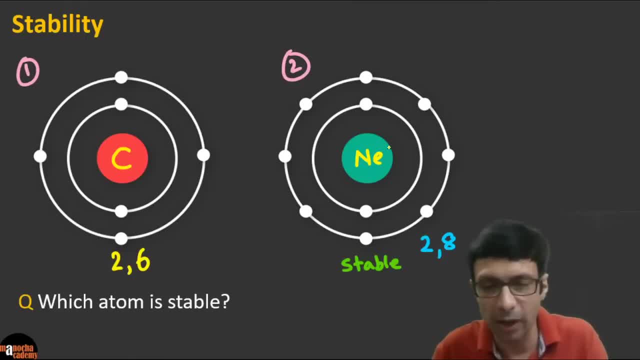 or it is. it is a stable atom because, very good guys, the octet is filled. so the stability of this atom is not kleine, because it is like a たjach and it is not big at all because in chemistry is decided by the electron arrangement. okay, and what is the rule? so the rule is at least. 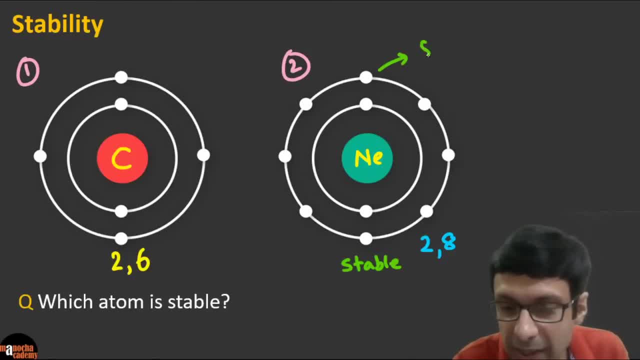 here we can see, an atom is stable because it has eight electrons in its outermost shell. okay, so it has eight electrons in its outermost shell and, as you guys are saying, you guys know it already. awesome guys, this is called the octet rule in chemistry, right? just like if you read the. 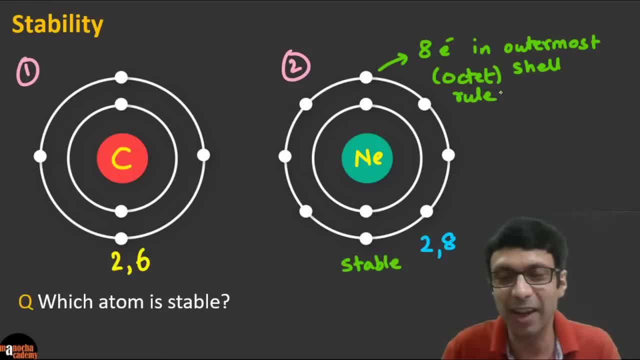 harry potter book. in harry potter, seven is the magic number. right, there are seven books, right, i think seven horcruxes, seven is the magic number here, it's eight. in chemistry, if you have eight electrons in the outermost shell, it is a stable atom. okay, that is its stability. it does not want. 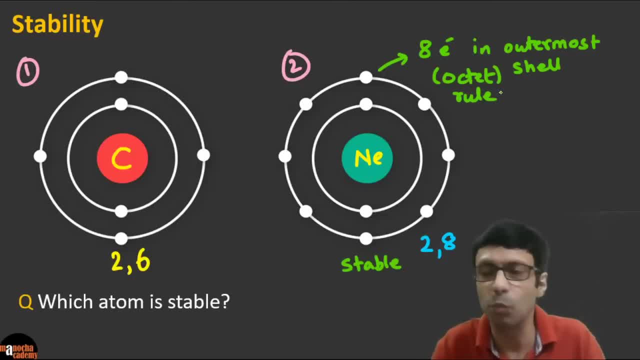 to combine with others. but carbon, it's not that carbon atom we can say completely unstable- right, it is there, but it wants to combine with others to become more stable. okay, so carbon goal is, uh, trying to get to this state, the octet state. so this is the goal of carbon: to try to get. 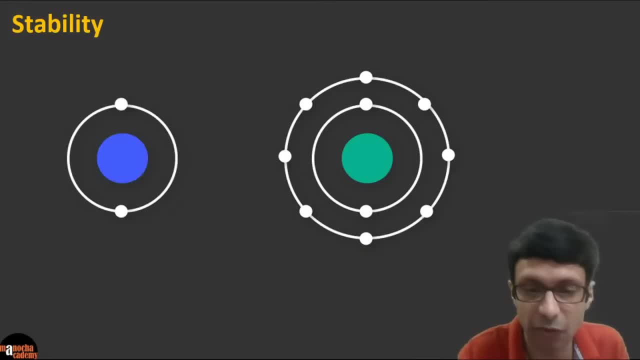 to eight electrons, okay, and it's just not octet, right, so you must be- uh, you must have heard of this. the stability rule is actually twofold. it's either the duplet rule, okay, so let's talk about it. so what is the stability rule, the duplet or the octet? and let's discuss what that means, okay. 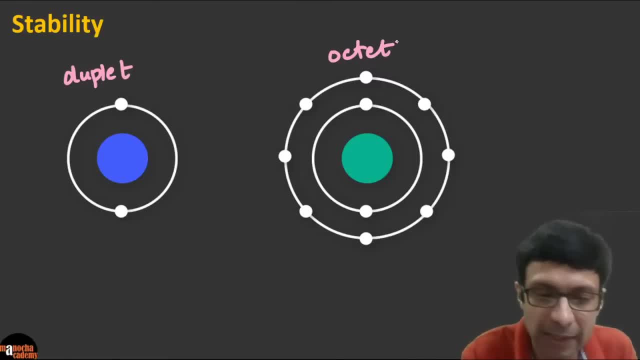 so do in the duplet rule, right? there's basically uh, for an atom to be stable, it should have only one shell. guys, can you see here? there's only one shell here. if it has only one shell, if the atom has only one shell and two electrons, okay, can you. 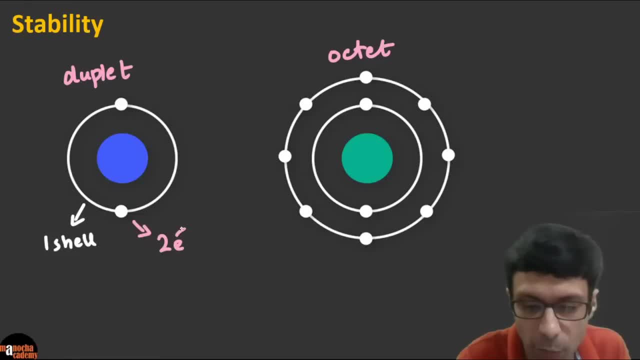 see one, two and two electrons in the outermost shell. so if one shell and two electrons, then also this atom is stable. and, guys, do you know which atom i have shown here on the screen? so what is the atom? uh, the left atom on the screen. come on, guys. 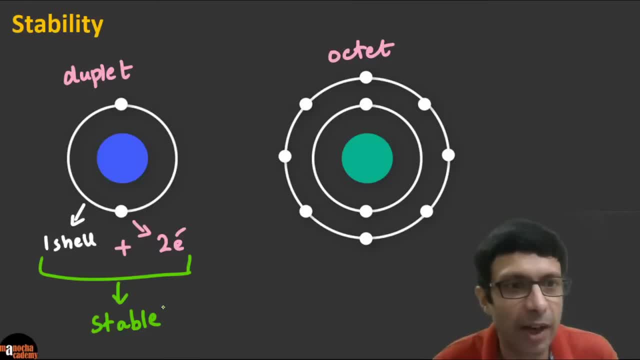 excellent, i see, satya narayan mangal has the right answer, right uh. namita has the right answer: super uh, right uh, saudami, you have the right answer. very good, so this is helium, right, it's following the duplet rule in chemistry, right? so if you have one shell and two electrons, or right? so stability can. 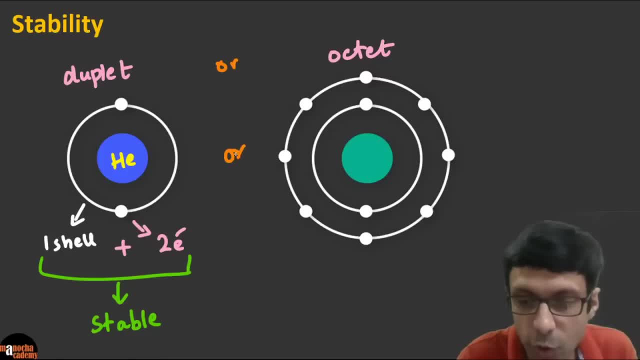 be either this or duplet, right, or you can have a configuration where atoms have eight electrons in the outermost shell. please look carefully here: eight. can you see the last shell? you don't have to look at the inside one. it could have if it has eight electrons in the outermost shell, like we. 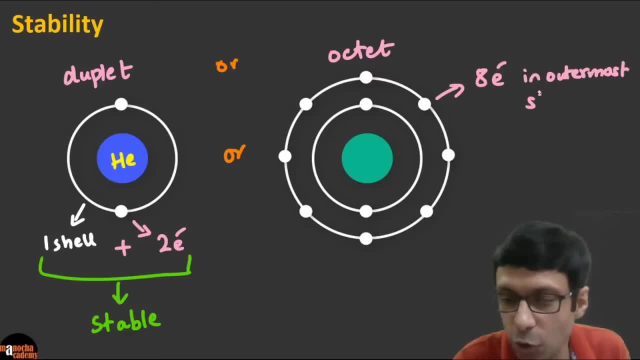 discussed in the outermost shell, then also, it is stable, so it's called either duplet. duplet means two or octet, just like octopus, octet means eight. okay, excellent, excellent, so this, uh, so it's either the duplet or the following the octet rule and you. 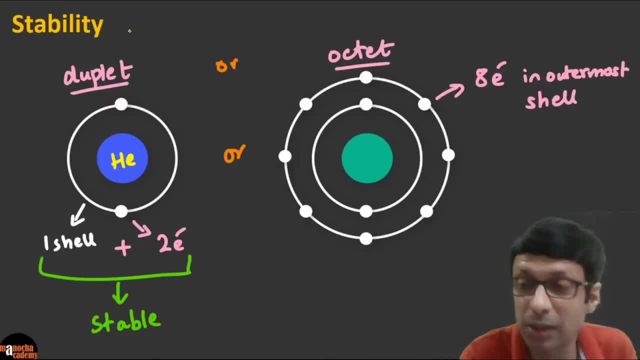 know who who follows these rules? so who, uh, who's the- what type of atoms- follows the rules? uh, these rules, it's the noble gases, right? or we say inert gases. you know they have the, uh, the stable configuration. so, noble gases or inert gases, they either follow duplet or octet, like helium, neon. 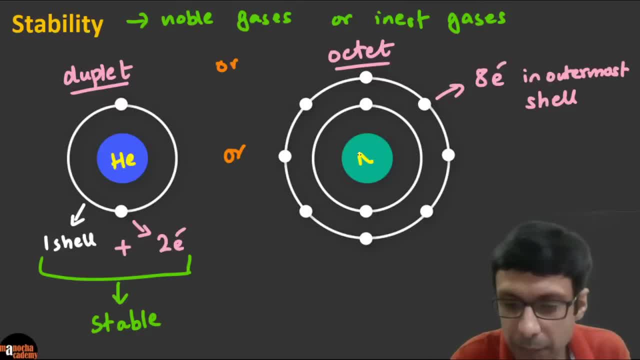 right, so this guy was neon. let's write it down here, right? similarly, argon, xenon, right? so these gases, they have eight electrons in the outermost shell, right? so this guy was neon. let's write it down here, right? similarly, argon, xenon, right, so this guy was neon. let's write it down here, right? so these? 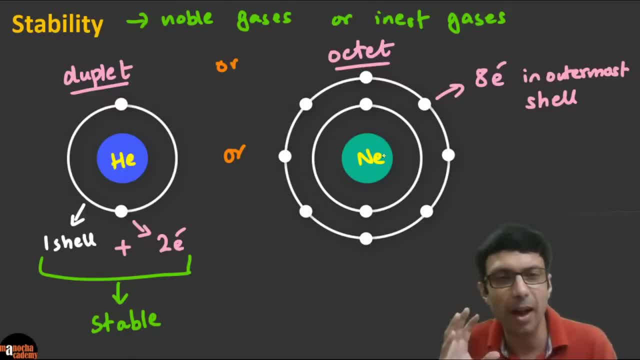 gases. they have eight electrons in the outermost shell. so all the atoms are trying to become a noble gas or an inert gas. they want to get stability right and that is why they form chemical bonds. so this is the key concept in chemistry: why an atom forms chemical bonds to get to this stable. 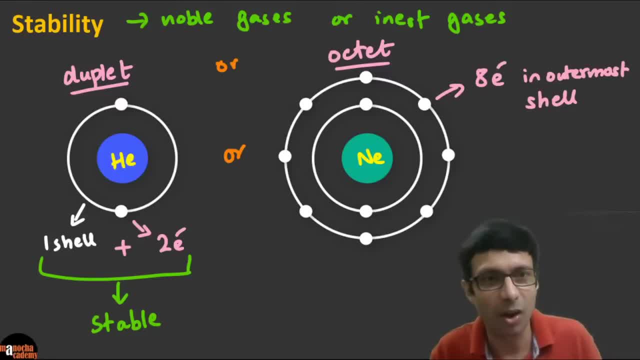 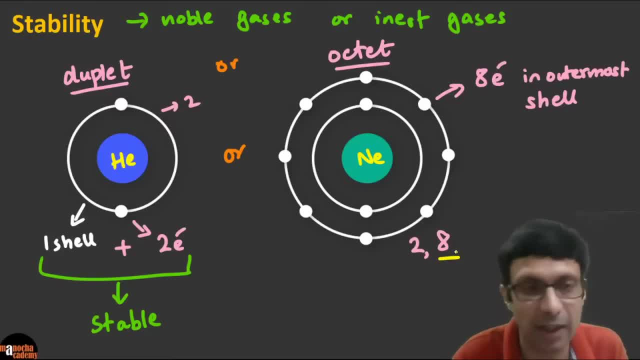 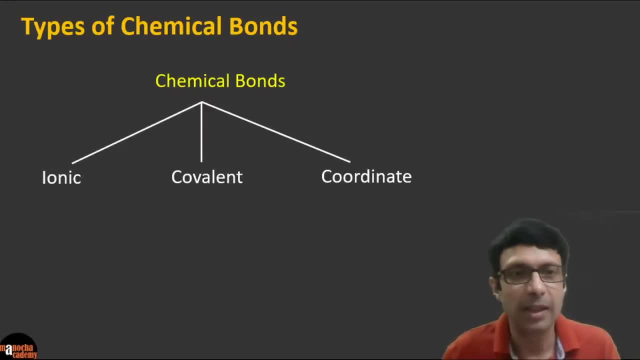 this one is 2,8, so the last shell is the key shell, right in the outermost shell. okay, right, that's what we have here. So now let's talk about the types of chemical bonds. right, so we've understood what is a chemical bond: the force of attraction between the atoms, right, that holds them in the 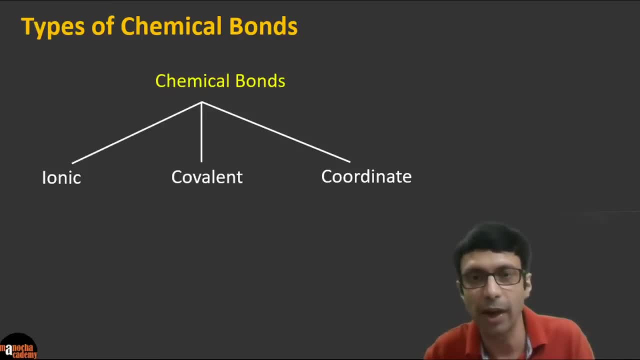 molecule and they do that for stability. so they can be classified into ionic bond right, covalent and or coordinate. so these are the three important types of covalent, of chemical bonds: right, so for ionic bonds we can also write: they are known as ionic or another word is, so you might have heard. 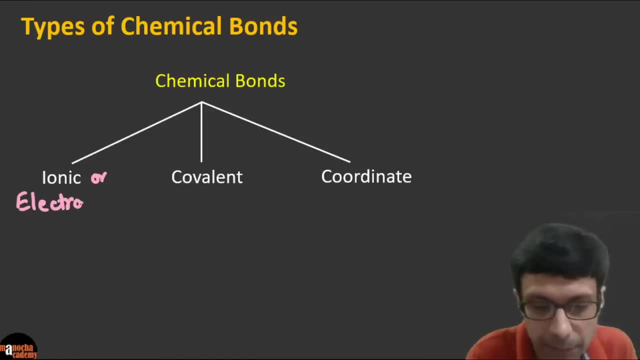 of this, or electrovalent- okay, so that's another name. it means the same thing. ionic or electrovalent covalents are also known as: or molecular- okay, so that's another name for covalent bonds and we are going to discuss them. right, and the last. 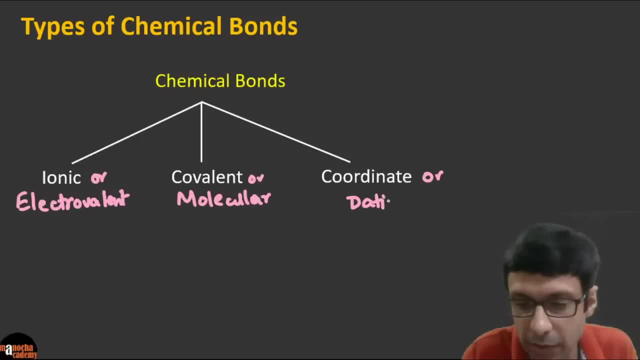 one coordinate. they are also called dative bonds. okay, so what is the difference? right, why these different types of bonds? okay, so what is? uh, because the key thing, as you can see, they're trying to get to stability, which means they're trying to get to the correct stable electron. 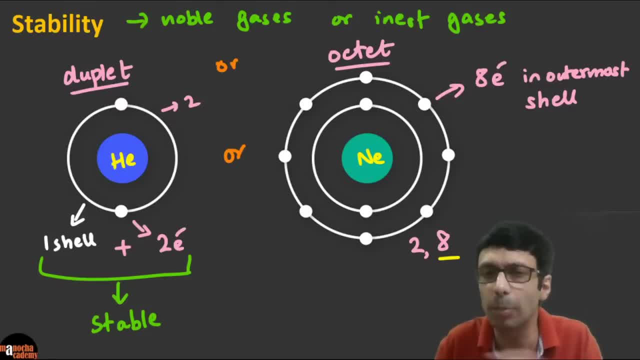 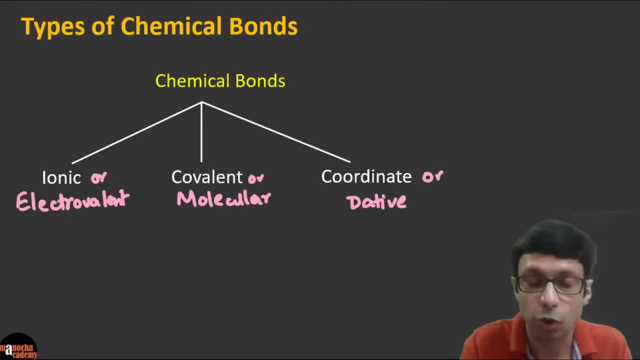 configuration. right, so electrons are the key here, not the protons, not the neutrons. they're getting to the key: electronic configuration right, okay, so to get to that. how do they do that? right? okay, so to get to that. how do they do that? right, so to get to that. how do they do that? 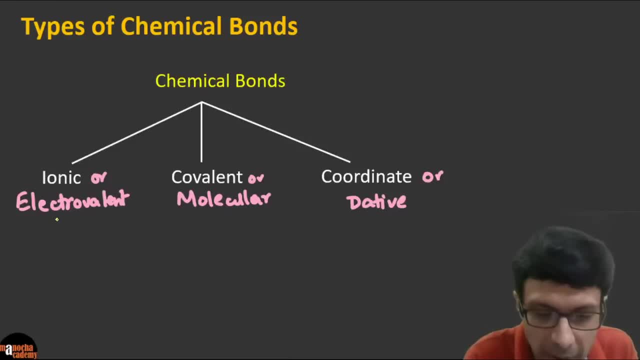 okay, so to get to that, how do they do that right? okay, so to get to that, how do they do that right? So for for ionic or electrovalent bond, they basically do the atoms do a transfer of electrons for stability. So the key point is transfer of electrons. OK, so that's when an ionic bond is formed. 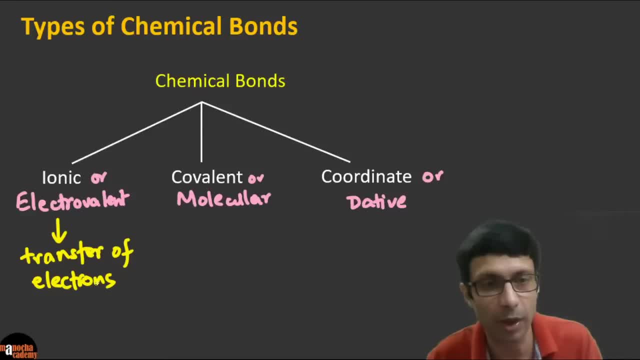 And, guys, do you know what happens for covalent or molecular bonds? OK, so what happens is it's basically done through sharing, sharing of electrons, Right, So that is done through sharing of electrons. OK, And the coordinate, or dative, is special. 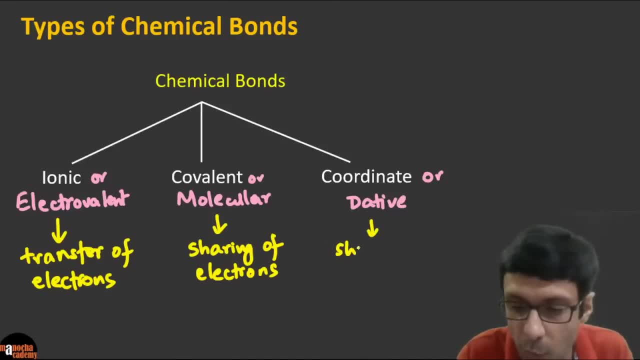 It's also sharing of electrons, But the shared pair comes from one atom only. OK, So the shared pair of electrons comes from one atom. in the covalent or molecular, Both the atoms are sharing. The electrons comes from one atom, OK. 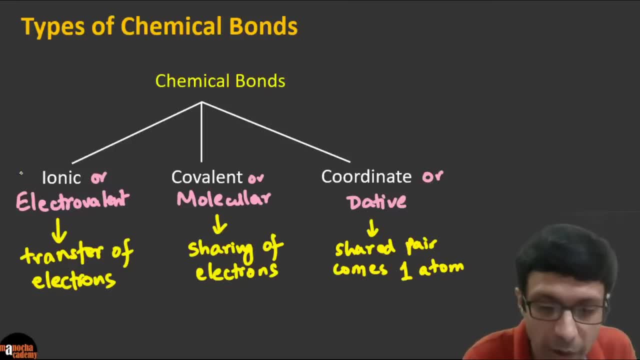 And guys. in this class our focus is going to be on ionic or electrovalent bonds and covalent. I won't be going into the details of coordinate or dative bonds in this class because the key chemical bonds are ionic and covalent. 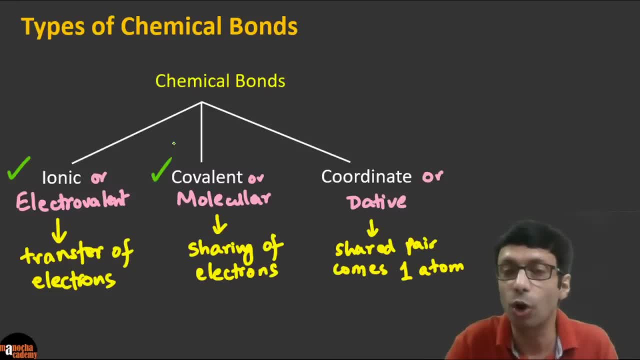 And I'm going to make the concepts crystal clear and show you how to draw the electron electron diagrams, Right. So the electron dot structures. I'm going to show you that, Right. OK, let's go ahead and discuss the details of ionic or electrovalent bonds. 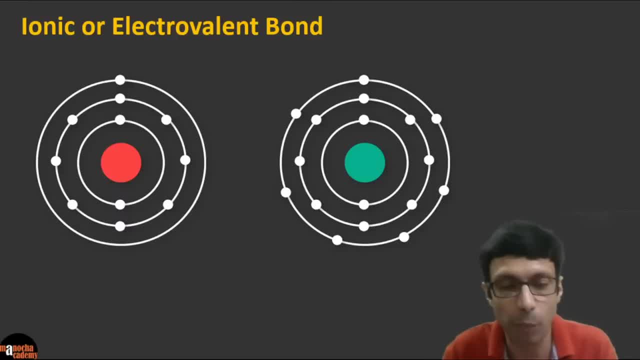 OK, very important. So ionic or electrovalent bond, The key point is they are formed by the transfer, as we said Right, Formed by the transfer of electrons. So let's take a look. What is the transfer going on here and why it happens. 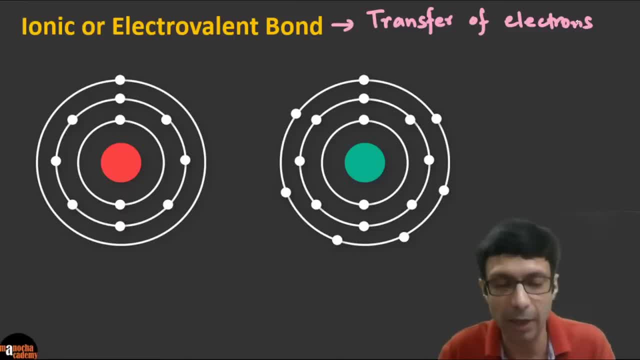 OK. So if you take a look at these atoms here, I've got these two atoms on the screen for you And let's take a look at their electron configuration really carefully. OK, guys, So, and you can try to identify which atom these are Right. 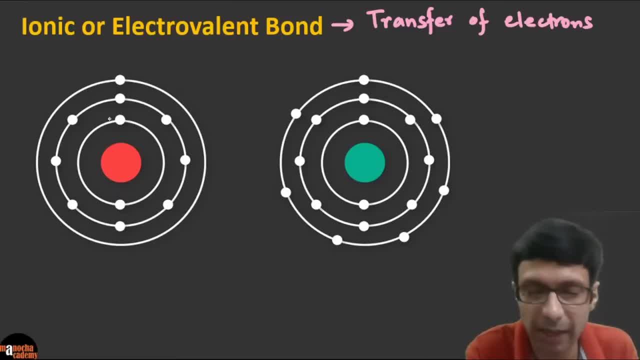 So how do you look at the electron configuration? So we start from the center, So in a, in a shell, Right, And so basically we have- you can see that- two electrons, then one, two, three, four, five, six, seven, eight and then one. 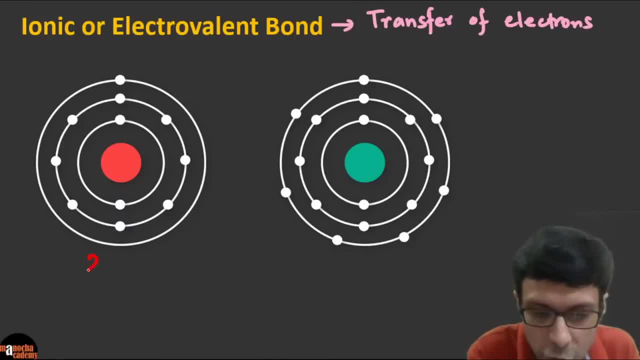 So this, this guy has a configuration of two comma eight comma one. Do you guys see that Right? So two comma eight comma one. Guys, can you tell me which atom is this? So come on, Can you tell me which atom is the first one which has two comma eight comma one? 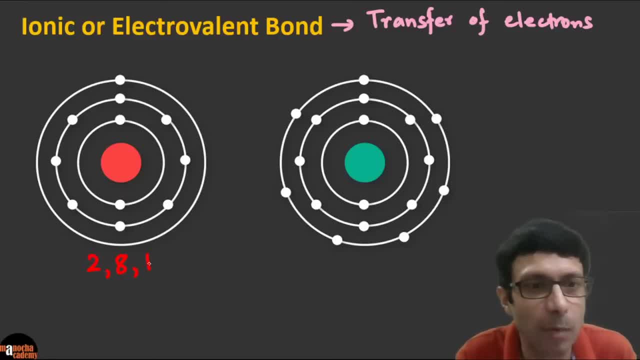 That means it has 11 electrons. Excellent guys. I see Gotham Right. The right answer, Srinivas. Very good, So this is basically the sodium atom, Right? Can you see the sodium atom And what is this atom on the right side? 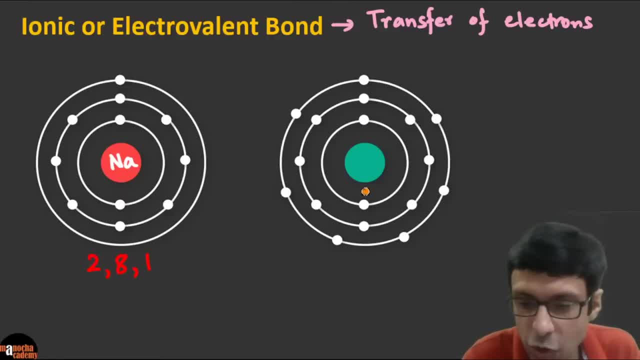 Let's take a look at its electron configuration. So if you take a look, it has two, eight and one, two, three, four, five, six, seven. So the electron configuration of this guy is two comma eight comma seven Guys. do you see that? 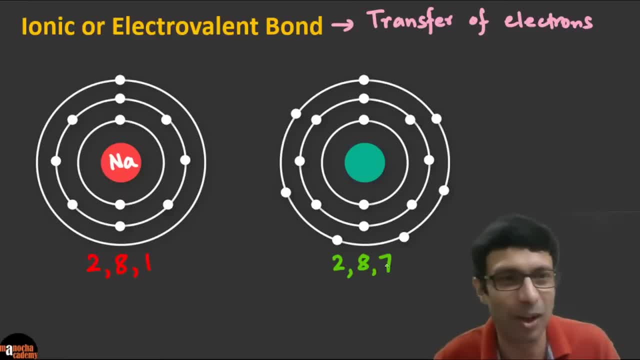 So can you tell me which atom is the one on the right? Come on, guys. OK, so very good. Srinivas says chlorine- Right, What do you guys think? Come on, OK. so Vinay says chlorine, Jaya Reddy, Excellent, guys, A lot of you are giving the right answer. 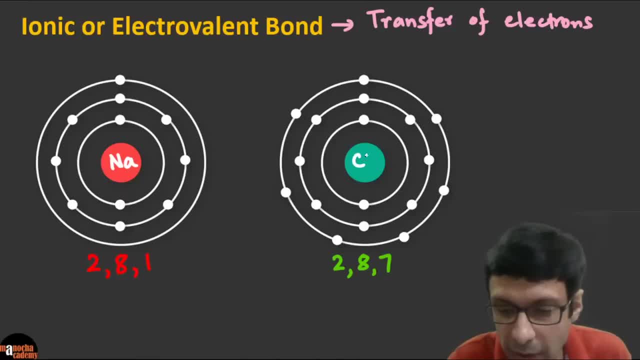 Sorry if I'm not able to take everybody's name, but it's great to see the interaction here. So chlorine, OK, And now let's see how they are going to combine these atoms. and why do they combine? So first thing that you can see here is that they don't have a stable state. Why? 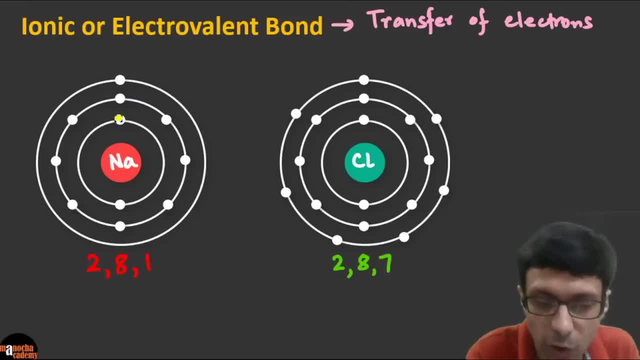 Because if you look at sodium, it has only one Electron in the outermost shell. Can you see It's comma one For stability it needs to get to eight. Same way, if you look at chlorine, it has seven. For stability it needs the outermost shell Right. 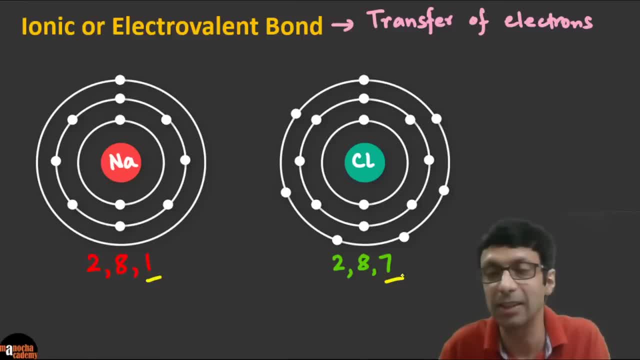 Not, not the one inside that you'll say: there's two comma eight. is there Eight is there? No, the outermost, which is called the valence shell, or the outermost shell, needs to have eight electrons. OK, so what are the options here? What can sodium do to get to a stable state? 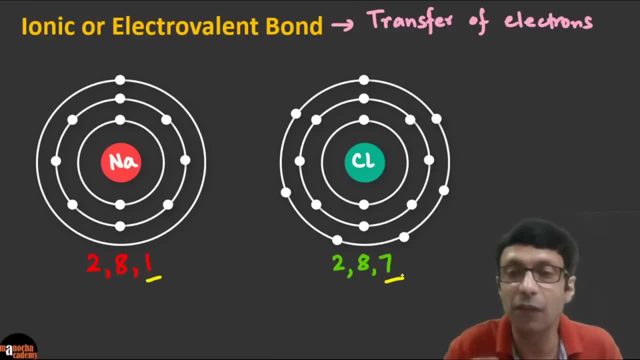 Either it can lose that last electron, Right, Give it away, or it needs seven more. Do you guys agree? So sodium has two options: Either give away that last electron, So this guy I'm talking about. So either it needs to give away this electron here, Right, Which I marked with the yellow color, Right? 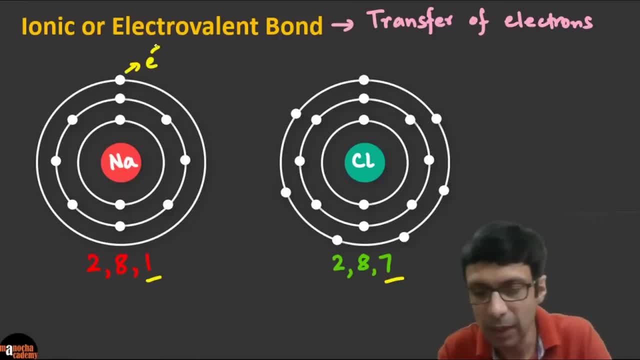 Either it needs to give that away or it needs seven more. Now let's take a look at chlorine. What is the chlorine's option? Either it has to give away all the seven, Right, Or it has to gain one, because it has seven there and its goal is to get to eight. OK, 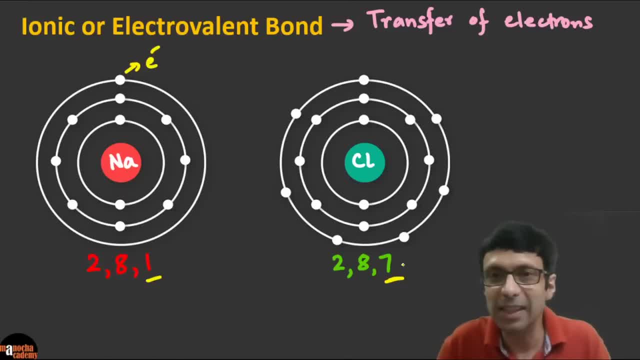 So what is the best solution, The best option here: Right. So for sodium it's easier to lose one electron Right, Then gain seven more. That's a more difficult task, Needs more energy. Right So sodium will want to lose this electron or transfer this electron. 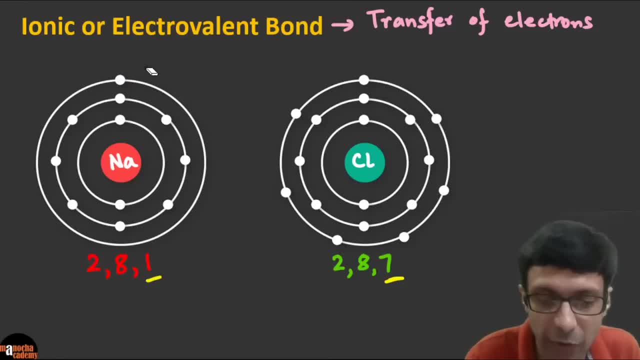 So he needs a friend who is ready to accept an electron. So sodium is ready to give away or transfer its electron. So there's going to be a transfer of electron Right- Very important- And this electron we are talking about, which I'm going to color in the yellow there. 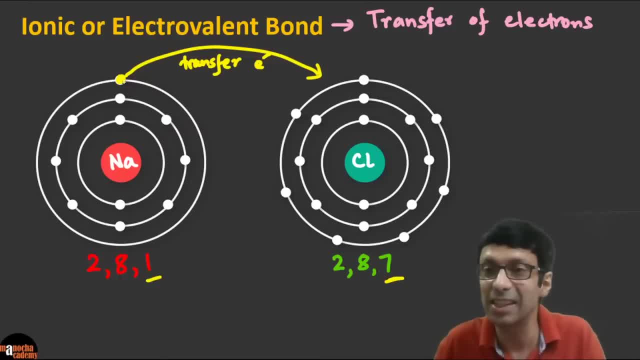 OK, And chlorine is ready to accept one, because it's easier to gain one than lose seven Right guys. So if he's ready to accept this electron, So this will. what will happen here? Can you see? sodium is going to basically become the configuration will become two. 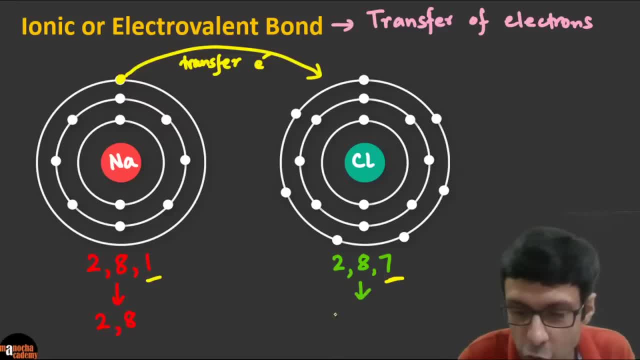 comma eight when it loses that, and chlorine will become two comma eight comma eight If it gains one. Excellent guys. So Mitra says sodium will lose the electron and chlorine will gain one electron Superb. So there's basically a transfer of electron. 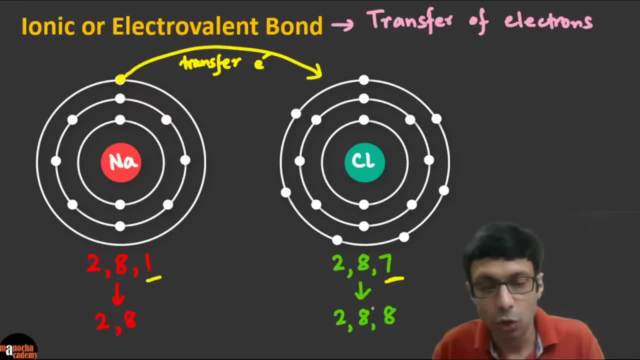 And now let's see why is an ionic bond formed. OK, so if you take a look, if sodium loses one electron, So if I represent this by sodium Right, So two comma eight, comma one is basically sodium Right, This is sodium. But what is two comma eight? 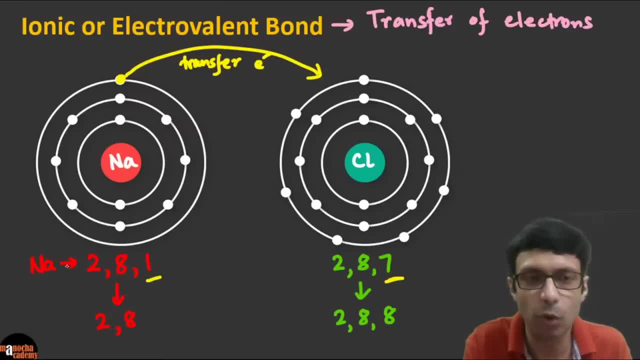 Since it's lost an electron, is it an atom anymore? No, because it's lost the electron, It's basically going to become the sodium ion. Can you see that? Because now it has one less electron, So it's going to become a cation, Can you see? 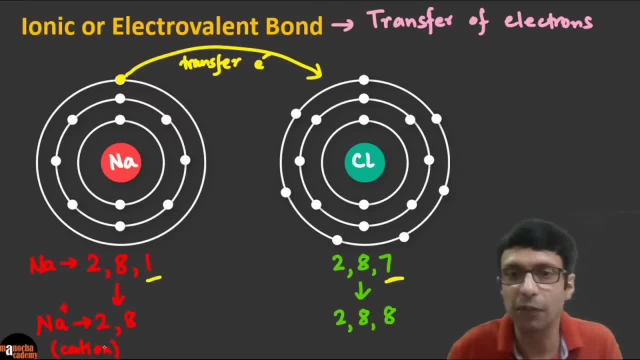 So it forms a positive ion, or what you know is called an electropositive ion or a cation, Right? So sodium is going to become a cation. And what about chlorine? Chlorine is going to gain that and it's going to become two comma. 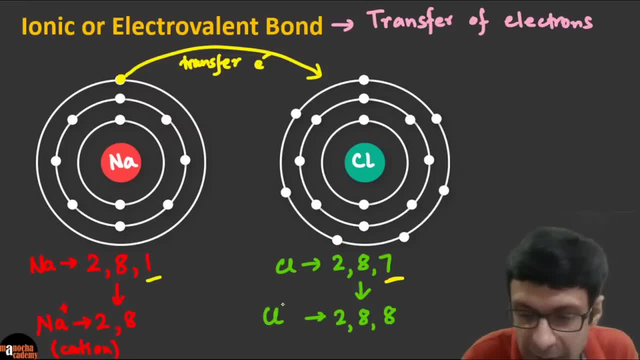 So if this is chlorine, this is basically representing CL minus the chloride ion and this is basically the anion. So can you see what happens after the transfer of electron? this guy? So let's say this transfer happened Right, So this electron goes from here. OK, 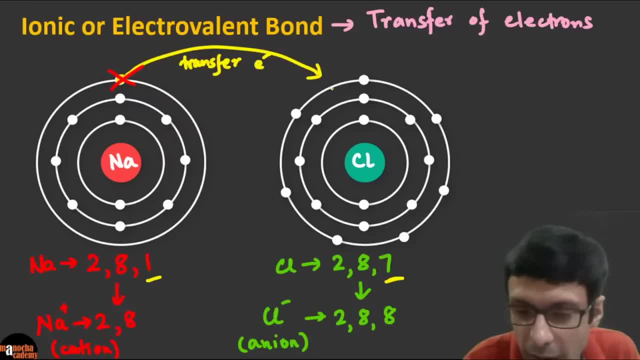 So it's no longer here. So I'm going to put a cross here and it's gone and transferred over here. So let's go ahead and place it here, Right? So can you see, this whole sodium thing is basically going to become positively charged. 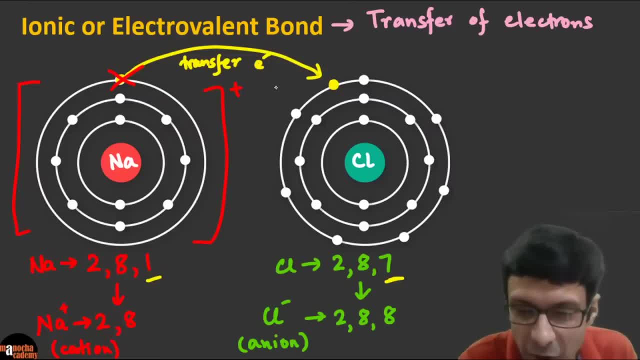 Do you guys agree? And what is going to happen to the chlorine guys? Chlorine atom is going to become an chloride ion, not chlorine ion. We say chloride ion in chemistry And it's going to have a negative charge. OK, And that is why it's called an ionic bond. 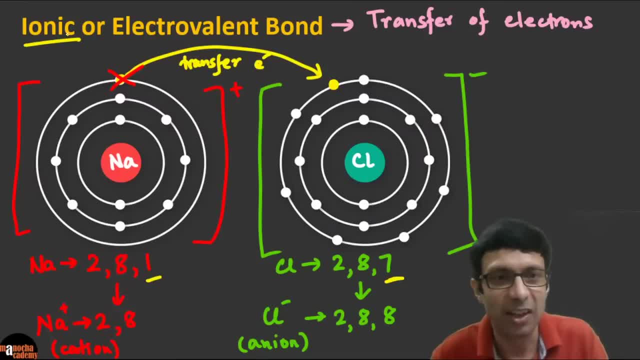 Look at the name guys. Ionic Because you have ions, the sodium ion here, any plus the cation, And can you see on the right the negative ion and positive negative, They attract each other. So that is why we have an ionic, or also known as electrovalent bond form. 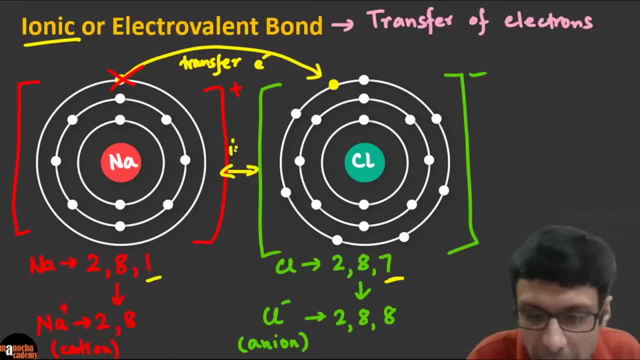 Got it guys. So is that making sense? We are having an ionic bond here between these friends, And our friends are sodium and chlorine, So they are forming an ionic bond because the one is positively charged, the other is negatively charged. 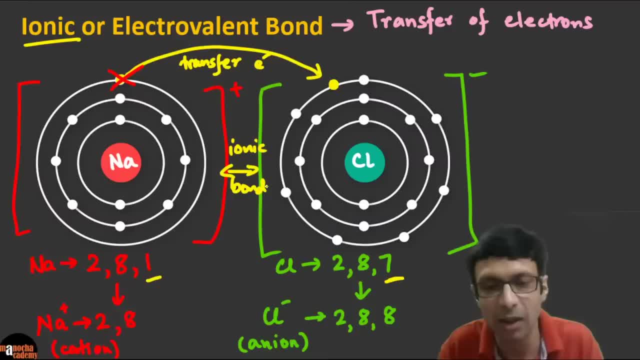 You know from science, right, positive, negative attract each other And this is why it is called an ionic or electrovalent bond, because we have ions formed as the result of this Right. It's no longer atoms, They are ions now. 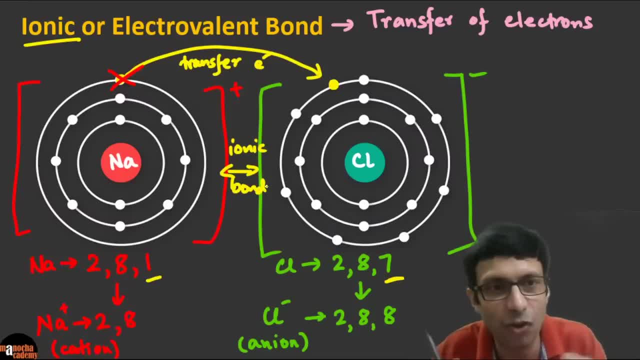 And it's a very strong bond because the plus minus, they attract each other Very good. Shreyas Hosu says: with a strong electrostatic force. Excellent Right, So there is a very strong electrostatic force here. Let's write that electrostatic force. 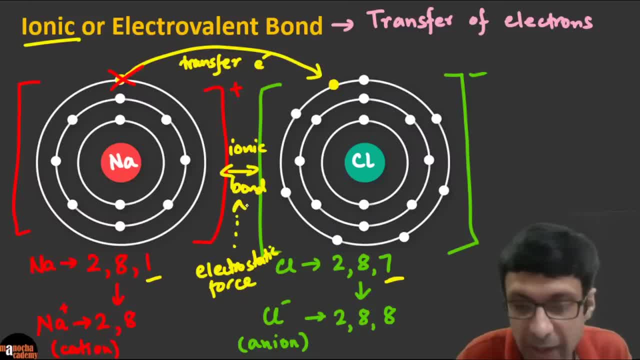 Right, And that is attracting these guys, Clear guys. So this is called an ionic or electrovalent bond. And who forms an ionic or electrovalent bond? Can you see, it is usually formed right. It is formed between a metal, Right. 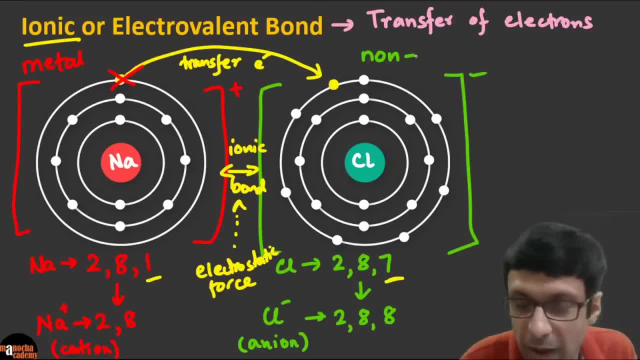 We have a metal here and a nonmetal, So ionic or covalent or electrovalent bonds are formed between a metal and a nonmetal. Why? Because metals they have a tendency to lose electrons. They have one, two or three electrons in the outermost of valence shell. 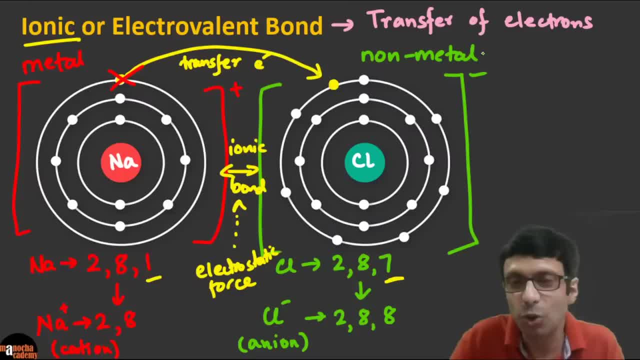 And nonmetals. they have four, five, six or seven. So they have a tendency to gain an electron And that is why, very important to know ionic bonds are formed between metals and nonmetals. Clear Right, Because one has a tendency to lose an electron. 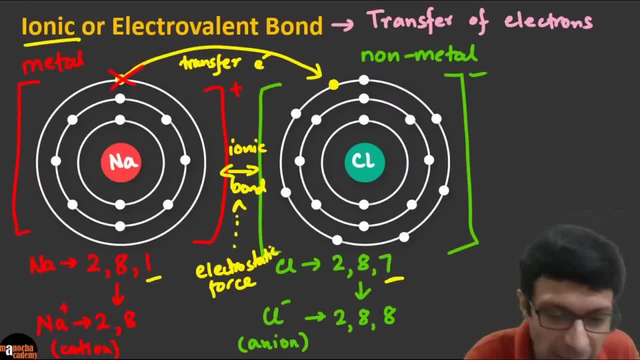 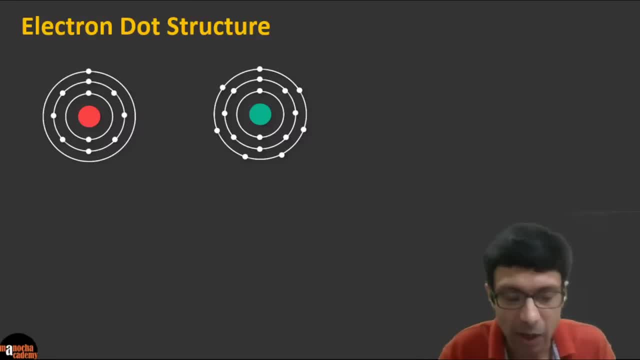 The other guy has a tendency to gain, So they like doing the transfer of electrons. Excellent guys. So this was the complicated, the full diagram that we discussed. Now let's see how we can express or show it in a simple electron dot structure diagram. 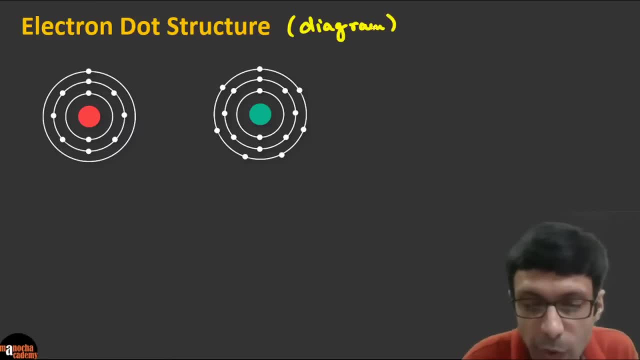 So we are going to discuss this diagram. It's very important because we don't want to draw all these complicated structures each time, Right? So, as we discussed, this was the sodium atom here, Right? So, guys, this was sodium and this was chlorine. 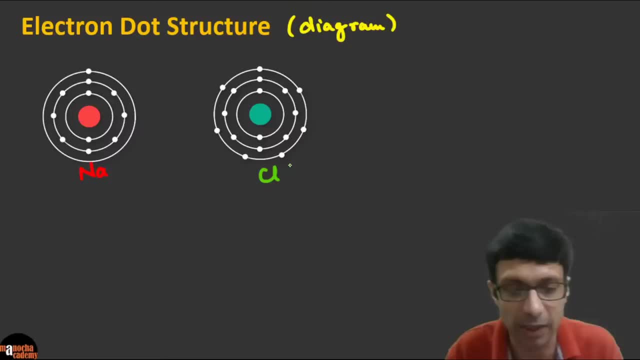 So let's take a look how to draw the electron dot structure for this. So guys carefully follow me and I'm going to make it really easy On how to show it Right. So first we look at sodium, Right, So I'm going to use the red color, just the matching color for sodium. 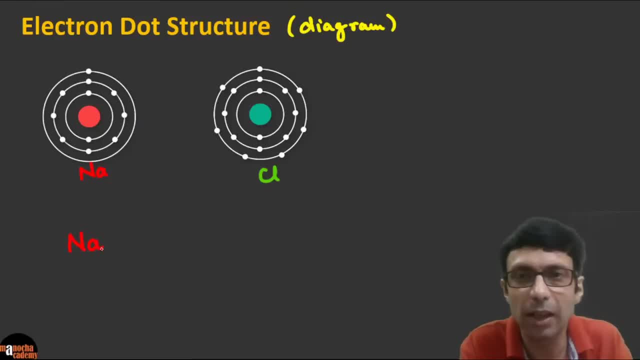 So we have sodium here, Right, And you need to draw. rather than drawing all the two comma eight comma one, You should only be showing the valence electrons, because the valence electrons, you know, are the key. So how many valence electrons does sodium have, guys? 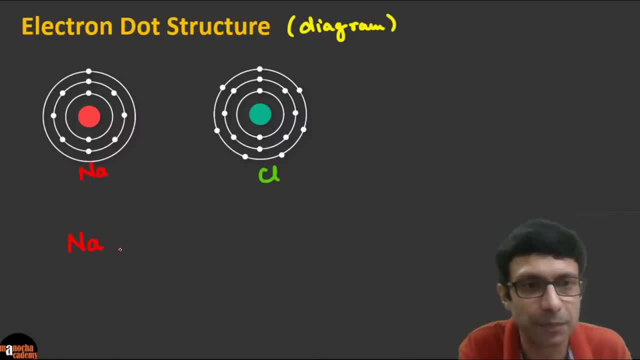 So can you tell me how many valence electrons does sodium have? OK, so who can tell me how many valence electrons in sodium? And, guys, if you Haven't hit the like button, please hit it right now and do share it out. 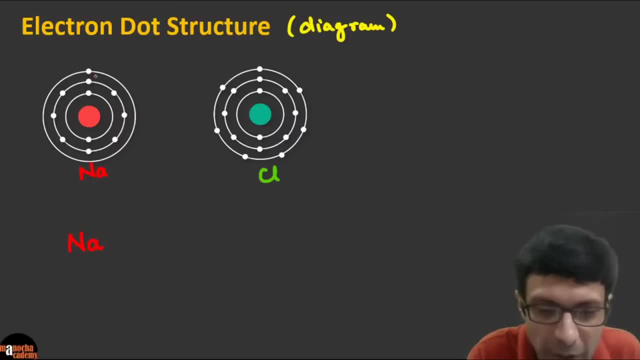 with your friends. Excellent, guys, I see the right answer here. So sodium, can you see? it has only one valence, electron, So we are going to represent it here. So let's represent it with a dot, OK, And what about chlorine? 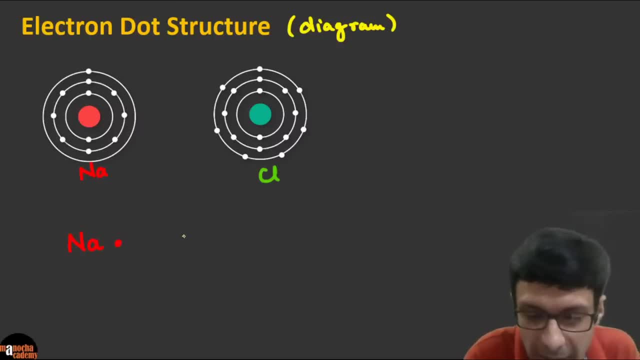 So we are not showing the whole configuration, We're just representing the dot And let's write the chlorine atom. So chlorine atom, Excellent, It has one Right, So very good. And guys, chlorine has how many valence electrons? we are going to show that. 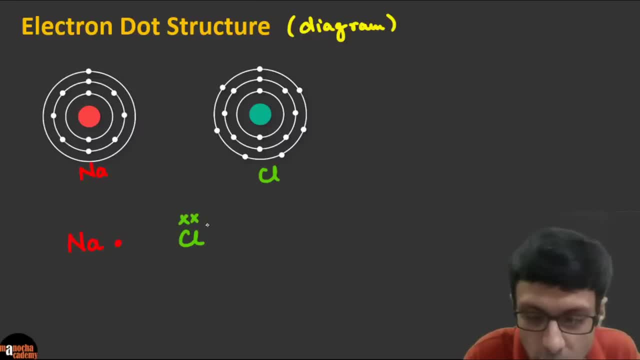 Seven Right, So let's go ahead and show that here. So one, two, three, four, And usually the electrons. you know they're drawn in pairs And I'm drawing it with a cross here. Some, some of you in school, you might be drawing all of these with a dot. 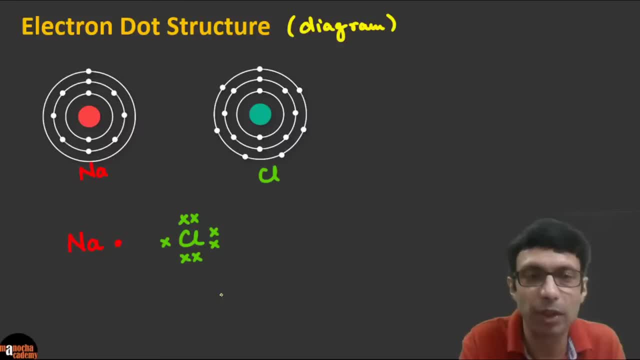 That's fine, But usually you know it's good to show one element with a dot and the other one with the cross. Excellent guys. Seven electrons for chlorine, OK. so that's how we've shown it, And now we need to show the transfer. 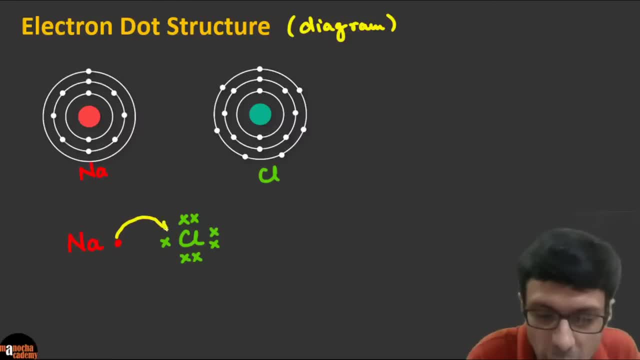 OK. so when these guys are going to combine this valence, electron is going to go and get transferred here, Clear guys, And you can put a plus here to show that you know these guys are trying to combine. So this is our simple electron dot structure, also known as right dot, and 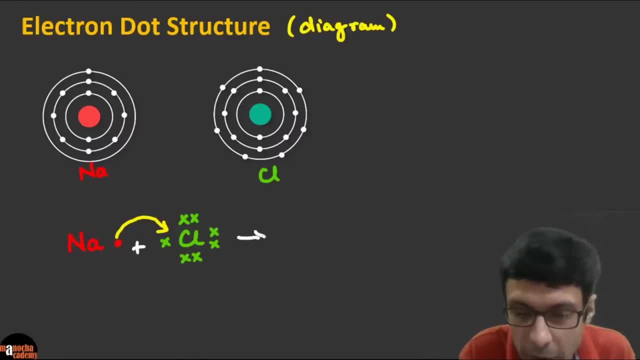 cross structure, because we're using dot and cross here. OK, And so what is going to happen as a result of this? Sodium loses the electron, So we don't have to show any electrons for it, because the valence electron is gone. 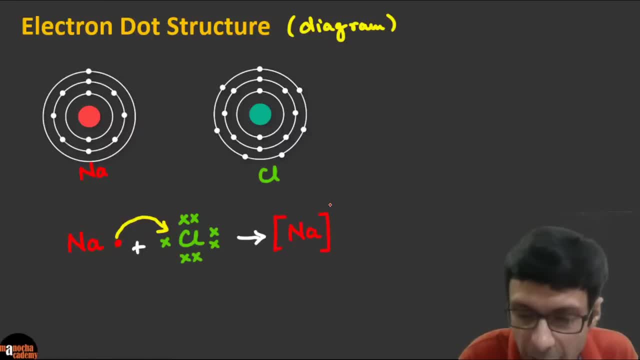 And you need to show these box brackets to show that there's an ion. now, OK, And I'm going to mark it with a positive charge, Clear. And now let's draw. What is the scenario for chlorine? So chlorine is basically here and we're going to draw CL. 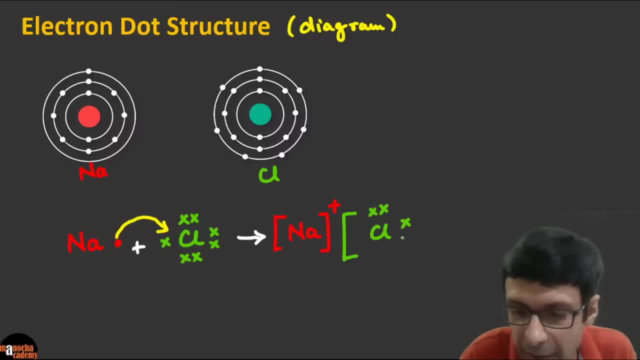 Right, And we'll mark all these crosses to show the valence electrons, chlorine and seven of them, And it accepted, Right. It accepted the electron from sodium Right. So we're going to show that here And, as I said, the electrons are shown in pairs, you know. 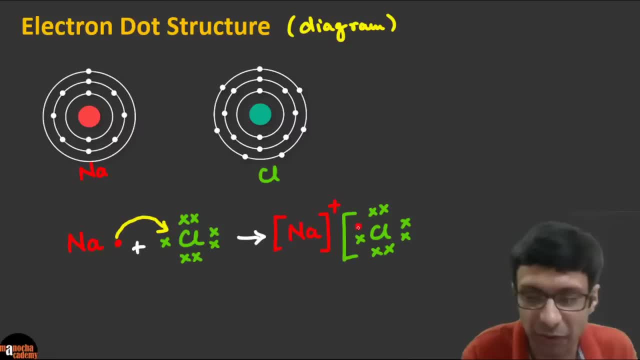 Right. So we put the sodium electron here, Excellent, Right. And we are going to show this also with this box bracket ring, because it's an ion and you need to write the charge: It is a minus one. had it be minus two. 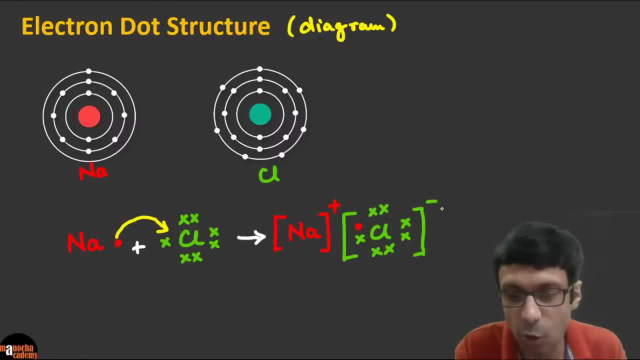 You have to write two minus Clear guys. So can you see that? So this is how we show the ionic bond, the electron dot structure of how the ionic bond is formed. And, guys, if you want to write the further steps, sometimes school ask you to write the formula. so you can write that. 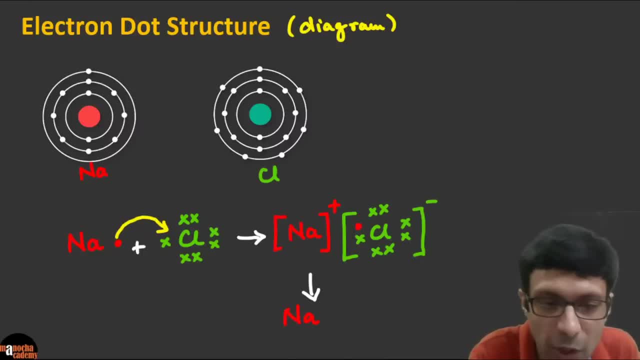 So, basically, what do we have here? NaCl? OK, Of course I'm using all these colors so that you know it's more colorful and easier for you, But you'll be doing it with a single color. But dot and cross helps to differentiate here. 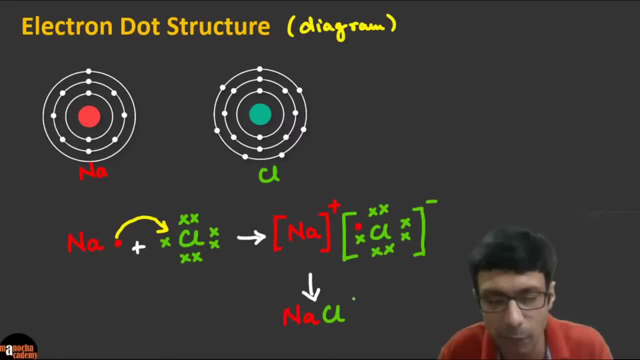 So, guys, please take a look at my diagram. Any mistakes that you see, anything I might have missed Clearly, can you see the transfer of the electron here, Right, And that's how the ions are being formed. Please mark the ions. 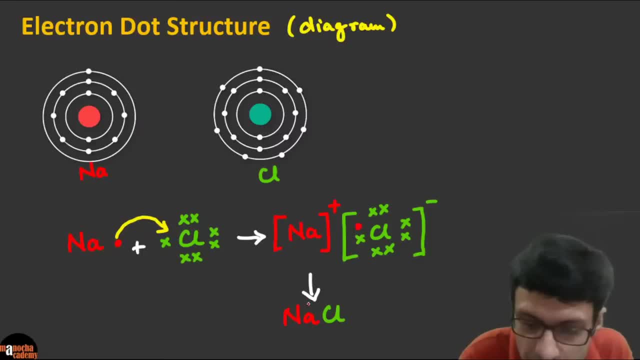 Don't forget to write the sign, And that is why we have NaCl. Sometimes, you know, the school might want you to write Na plus, Cl minus in the last step, also just to show that they are ions. OK, Or you can write NaCl whichever way they like, you know, or simply NaCl. 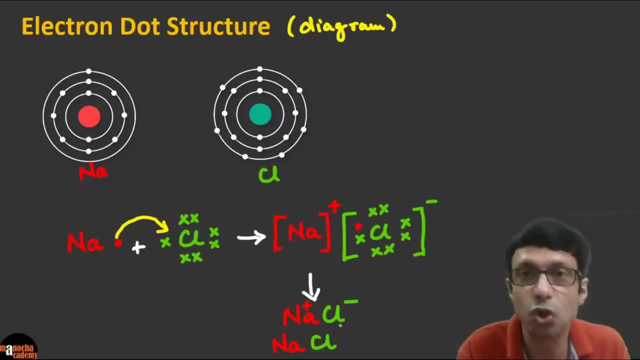 Right. So here we've shown the formation of the compound: sodium chloride, Right. What is our compound formed here? Sodium chloride, And it is an electrovalent bond because it is formed, Very important to know. Electrovalent or ionic are formed between a metal and a non-metal. 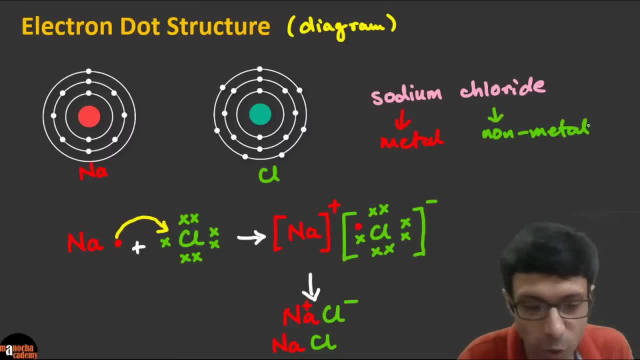 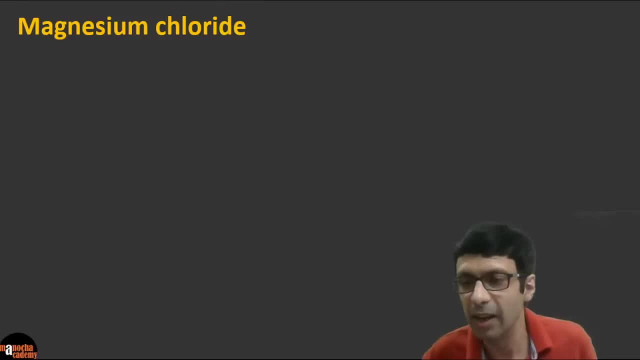 Do you guys see that Very, very important? OK, And I've shown you how to draw the electron dot structure. Guys, let's practice one more electron dot structure for magnesium chloride, And I know it's hard for you to show me. 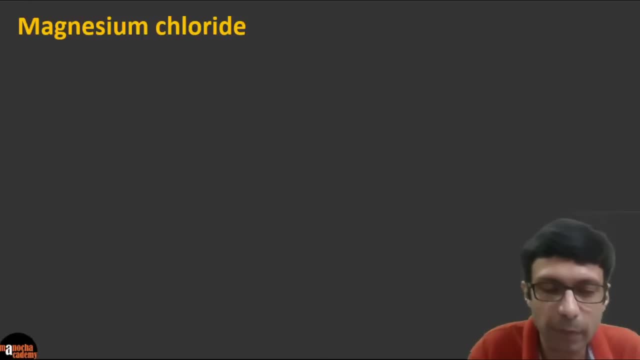 in the chat, but guys sit with a pen and paper and go ahead and try this. So let me show you the tips and tricks of how to draw the structure First, before you jump into the structure, the first thing is to ask yourself: what is the type of bond? 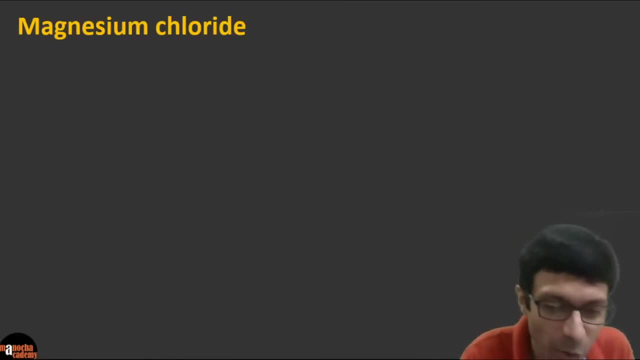 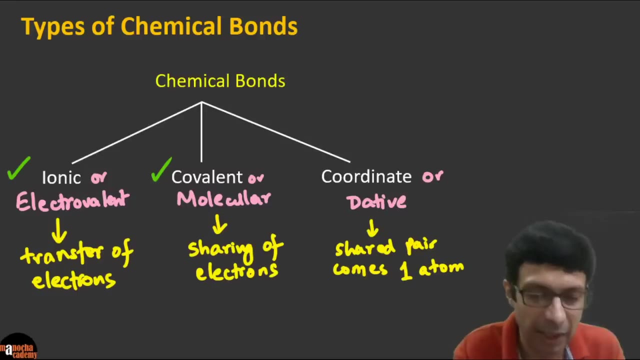 So you need to be, you know, like James Bond and try to identify which type of bond. Is it ionic or covalent? Because we are not talking about coordinate right now. So our main options are: is magnesium chloride an ionic bond or covalent bond? 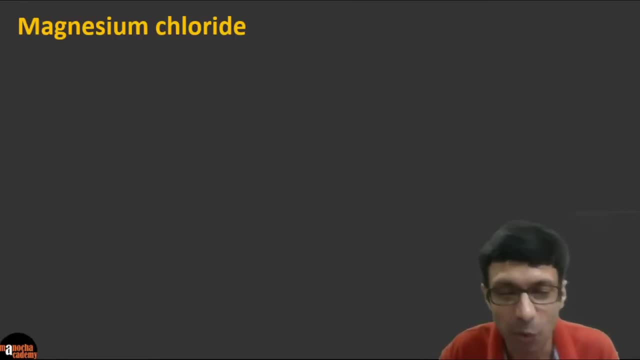 And, guys, can you tell me? So you need to be the James Bond and tell me which type of bond. So before you jump into the drawing: excellent, It is an ionic bond. Why, guys? Why is it an ionic bond? 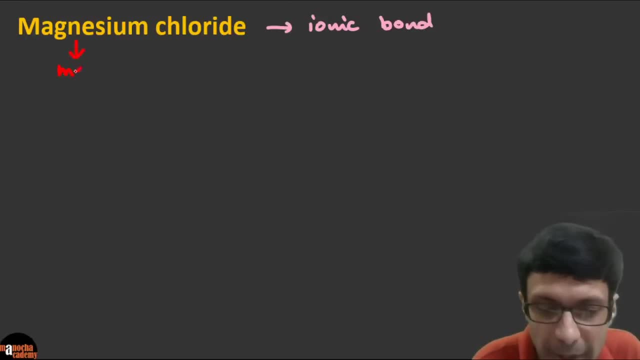 Because you know that magnesium is a metal, right? So magnesium is a metal and, guys, chlorine is a non-metal, And you know that the bond formed between a metal and a non-metal is an ionic bond. So first think of that. 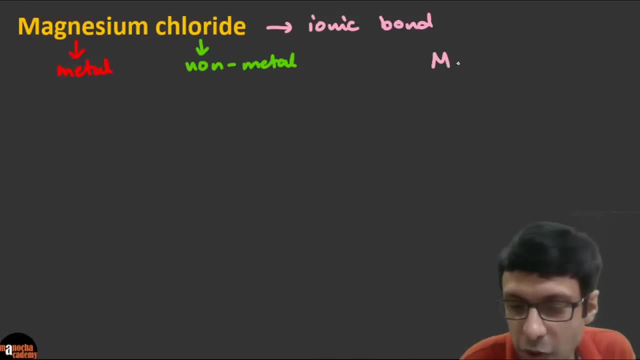 Next thing, important to think: what is the formula of magnesium chloride? So magnesium has valency two, chlorine has valency one. So if you do a criss cross in your rough, you're going to get MgCl2, very, very important. 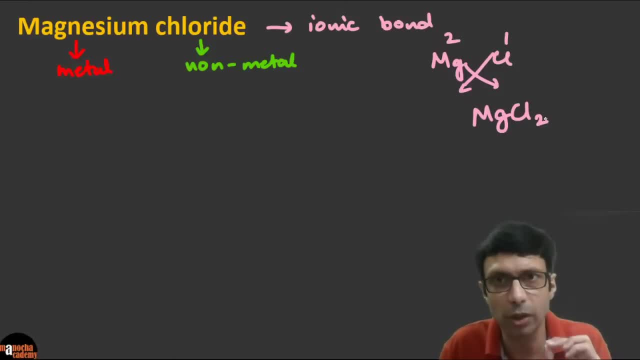 Before you jump into the diagram, guys, make sure you know the formula, you know the type of bond. OK, now let's go ahead and do that. Let's go ahead and draw electron dot structure. Excellent, guys. I hope you enjoyed this video. 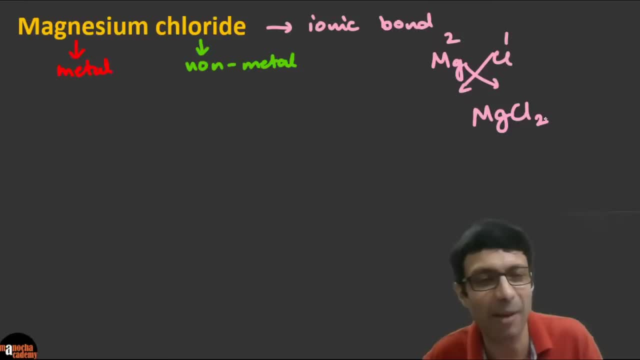 And guys, great to see so many likes out there, And please hit the like button if you haven't hit it already. I'm going to make chemical bonding super easy for all of you. OK, so let's go ahead and draw magnesium chloride. 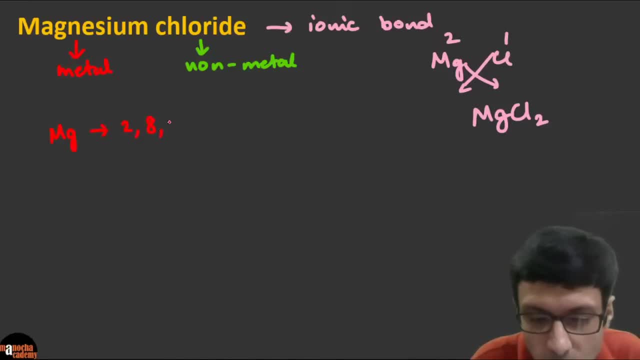 So magnesium, you know right, It has two comma eight comma two. that is its electron configuration. I'm not drawing all of that right. And chlorine, we saw, is two comma eight comma seven. So let's draw the diagram, guys. 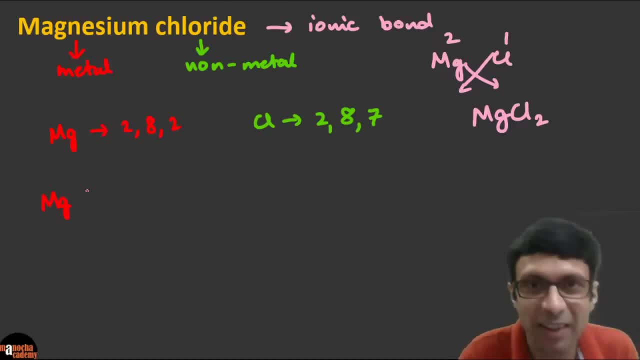 So magnesium is going to have two electrons in its valence shell. Thank you guys. Thanks for the likes. So we are only going to show the two valence electrons and usually be show it as a pair, OK, or, if you like, some of you you know. 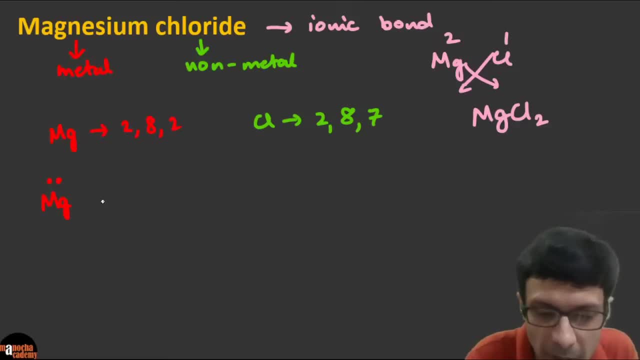 you like to draw the pair on top, you can draw it anywhere you want, That's no problem. Plus chlorine: OK, so there'll be a chlorine here and that's going to have, you know, two the seven electrons. right, because two comma eight comma seven. 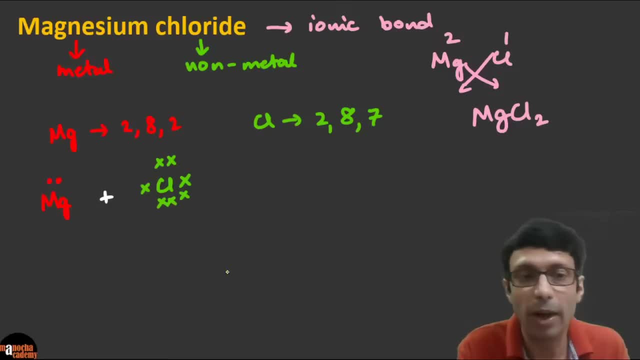 But we will only mark the valence electrons. Now, one interesting thing is: can you see? we are looking for MgCl2? MgCl2 is our goal. We have only one chlorine atom. OK, so one electron from magnesium can be transferred to chlorine and you can see. 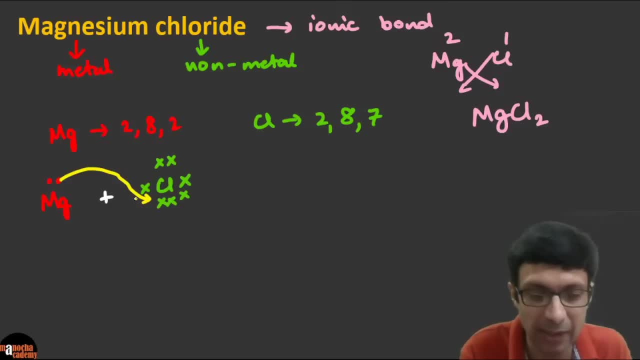 that it's going to get its octet state. OK, it's going to get eight electrons. Oh yeah, I think I forgot to mention that. guys, If you see here, can you see that chlorine has its octet state? 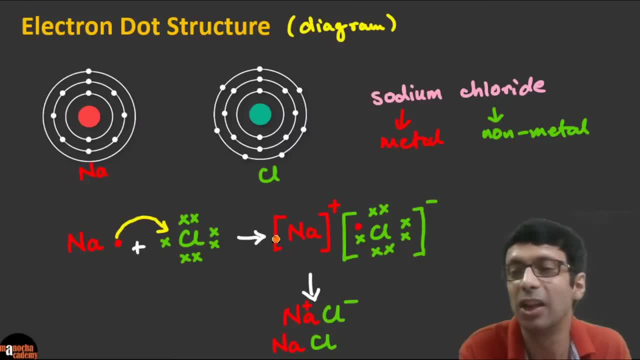 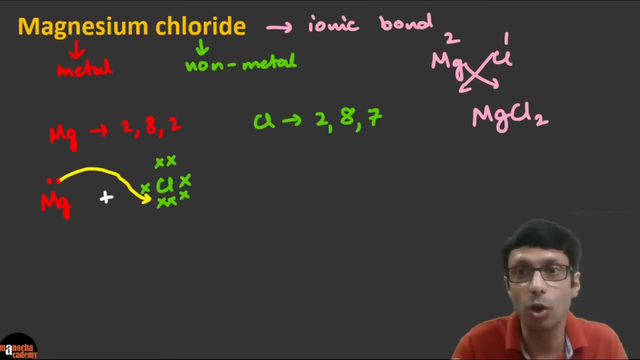 Eight. electrons right And sodium also lost it, So it's two comma eight, which again it got its stability right. Octet state: So same thing here. Chlorine will want to accept one, but it doesn't want to because it wants eight. 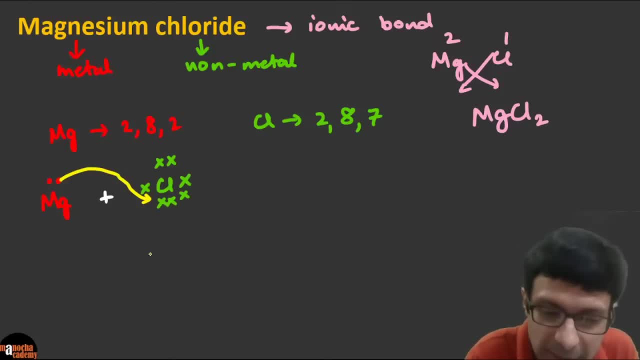 Right, So it's got it. So it's actually this: there's going to be a second atom of chlorine who's going to be accepting the other one? right guys, Do you agree? Because it's MgCl2, right, So there's another atom of chlorine which will accept magnesium second electron. 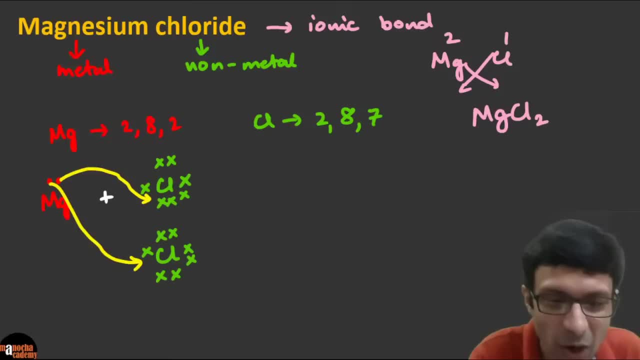 So that's why you need to draw two of them. clear guys, Awesome. And now we go ahead and draw this. So again the same thing. we're going to show magnesium in the bracket because it's an ion, and what is the charge I need to write for magnesium? because it's losing. 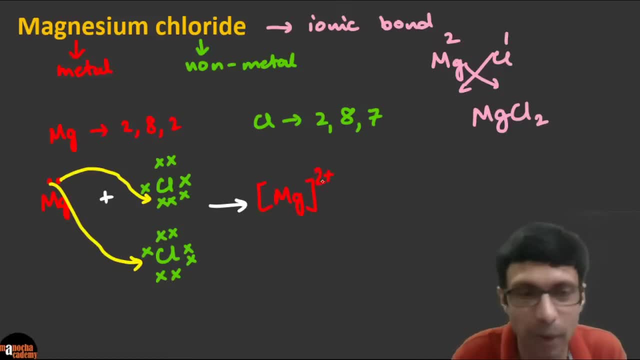 two electrons, what will its charge be? of course positive, but two plus Right, guys. Excellent. Raja says Raja Mukherjee says two plus Absolutely right. And guys, what about chlorine? OK, so what do you think? chlorine will be written here. 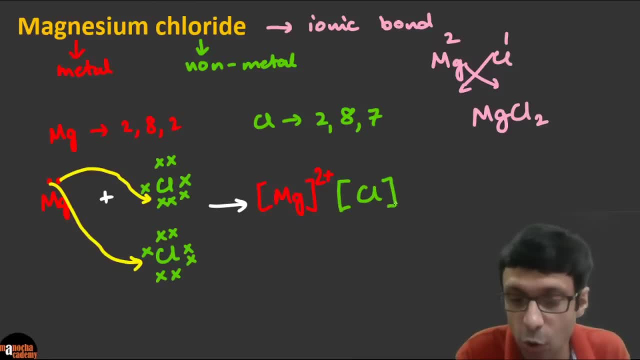 It will become chloride, right, And will chloride be two minus No Chlorine it has got. So here let's draw its original seven electrons, shown with the crosses. and then it got magnesium's electron, which I'm going to show with the red dot here. 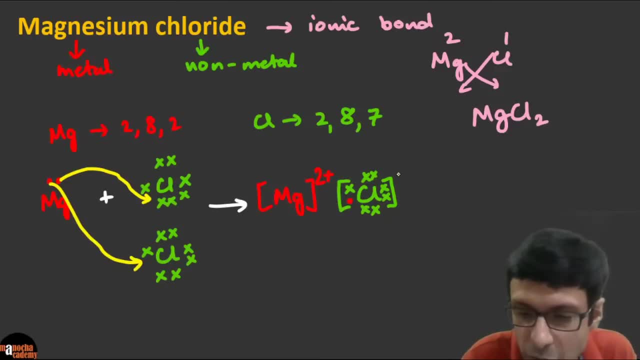 OK, but each chloride is going to be basically one minus right or simply minus, OK, but we need to represent two chlorides, So usually we write it two here, OK. so, guys, one important thing to note, very important. 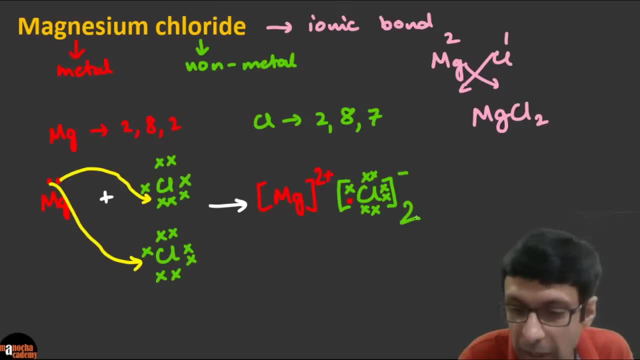 Let me raise that to. it's a lot of you might want to think: let's write the two here, but that is not the convention. OK, you may ask me why. it's just a convention, guys. Not that this is not wrong, but this is not the way to show it. 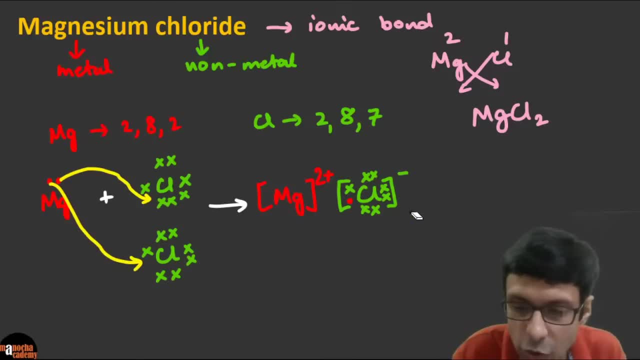 So in by convention it is wrong. So I'm going to cancel this too. And we need to put the two here right in front of, because it's two chlorides, OK, so please remember, this is how you represent the, the dot and cross structure for ionic bonding. 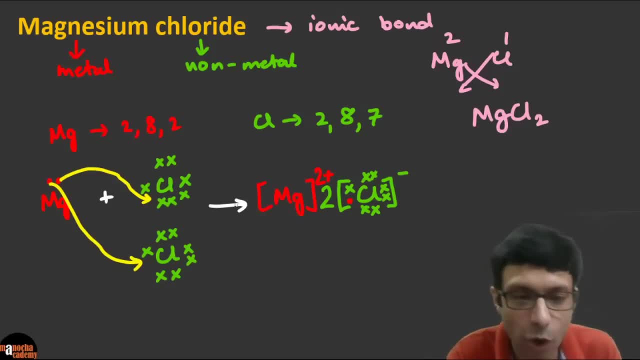 OK, don't forget that, guys. Can you see that? And look here, Magnesium has lost that final electron to two electrons. So it's now. can you see? magnesium is now. if it loses this, it's going to be two comma eight, right? so it's got its octet state, stable state and each chlorine atom. 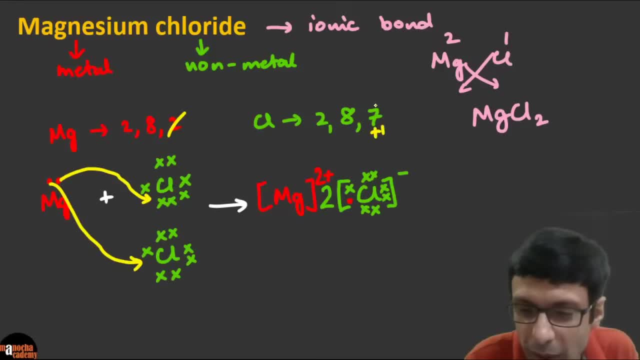 has gained one. OK, so here it's seven plus one over here. So can you see that it's going to be eight here, as you can see in the diagram, And so basically, what we have over here is MgCl2, our ionic compound, or electrovalent compound. 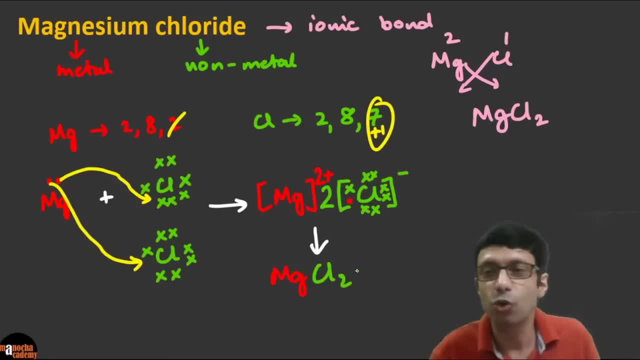 Excellent, guys, Excellent. So is this crystal clear to you: how to draw the, the electron dot structure, And so all of you can now be James Bond. you know. Main question: what to ask? Is it ionic or covalent? 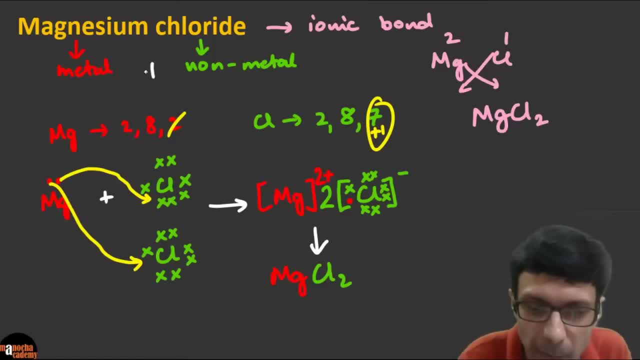 Think carefully: metal and nonmetal. metal and nonmetal were combining, So it's definitely going to be an ionic bond. OK, because metal tends to lose electron, nonmetal wants to gain. So there is a transfer. Can you see in the yellow arrow? 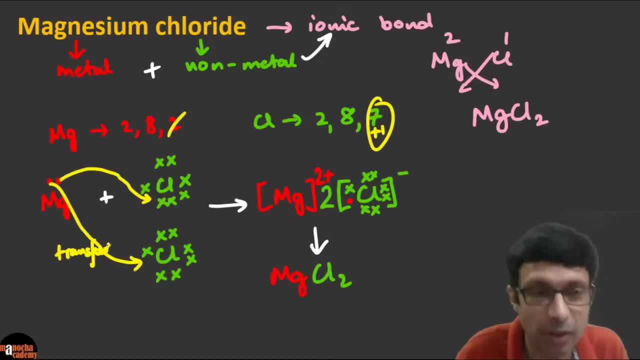 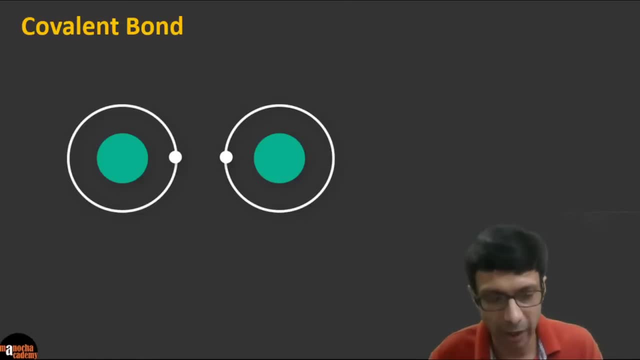 There's clearly a transfer of electrons. Excellent, guys. So is everyone clear? Awesome, Let's go ahead and move on to the next type of chemical bond, which is covalent bond. OK, covalent bond. And what is the key thing in the difference between ionic and covalent? 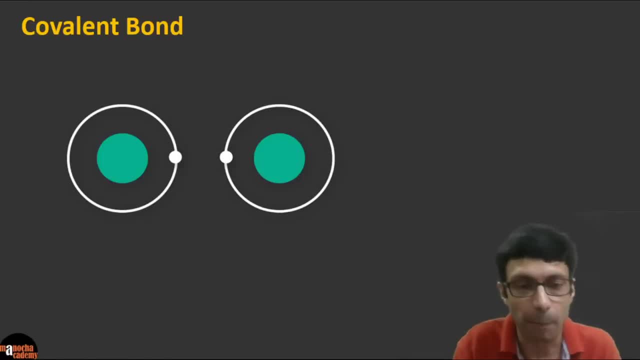 Ionic was, remember, transfer of electrons, But covalent. covalent is sharing of electrons, OK, so sharing of one or more pairs of electrons. So that's the key difference: there It was transfer, Here it is sharing. 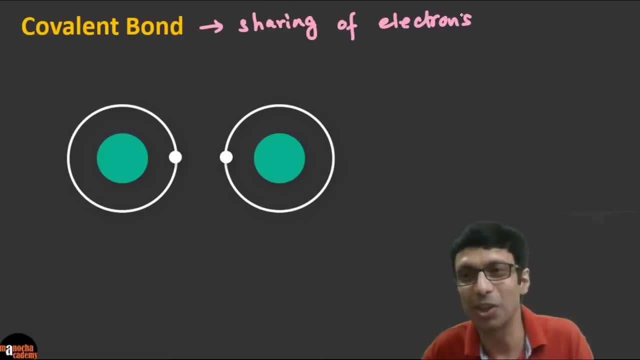 And, guys, you know, sharing is caring, Right, And these atoms are really caring atoms because they want stability. OK, so let's take a look. Why are they doing sharing and why not transfer? So, guys, can you tell me which? 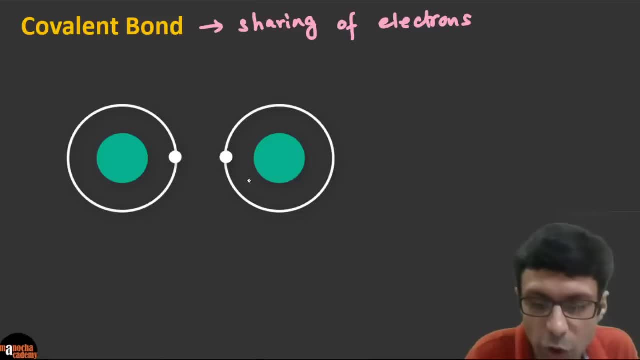 So here there are these two atoms, Right, Can you see? So you've got two atoms on our screen here. These are separate atoms. Can you tell me which atom are these? OK, can you see? each of these atoms have only one electrons. 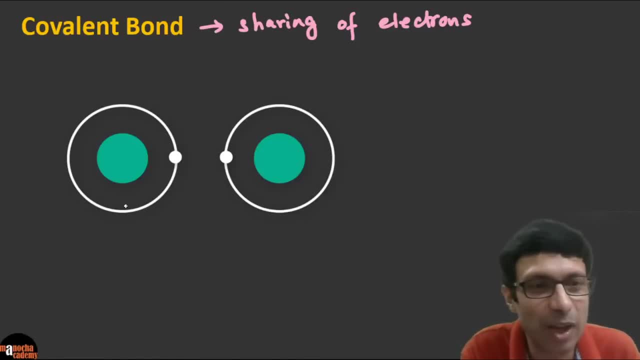 Right, I agree, Sharing is caring, Right. So, guys, can you tell me Very good. So guys go ahead and say: I see a guy says hydrogen, Right, Srinivas says hydrogen. What do you guys think? Come on. 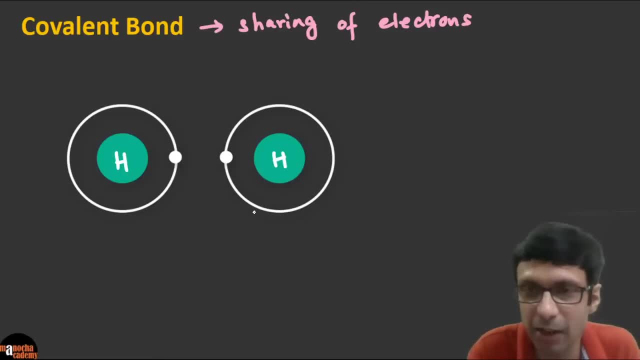 So this atom is clearly hydrogen, right? Because you know, hydrogen is the simplest atom. It has only one electron, as you can see here, Only one electron in its valence shell. OK, And guys, can you tell me, is hydrogen a metal or a non metal? 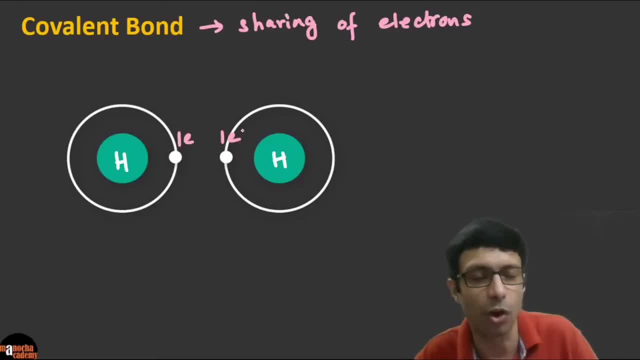 So, come on, who can tell me what is hydrogen? a metal or a non metal? Right? So I want all of you to tell me. So this is clearly hydrogen. Is it a metal Or a non metal? And we have these two hydrogen atoms trying to combine here. 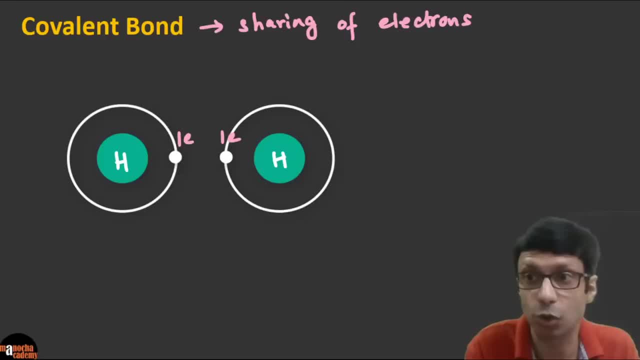 OK, great, I see some of you are saying metal. So, guys, this is very important thing. You guys should be very clear. What is hydrogen? Of course it's in, you know, group one of the periodic table. 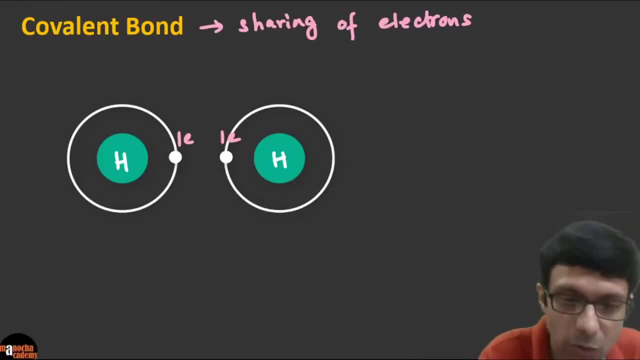 It's there with the alkali metals, But hydrogen is a gas, OK, and clearly we don't have any metals which are gases. So you can remember that way. Hydrogen is clearly a non metal. Please remember that. OK, So I've been writing non metal in green, so I'll write that you know. 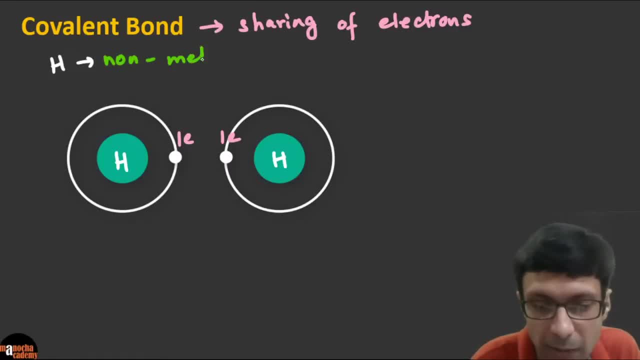 So hydrogen is clearly a non metal, It's a gas, right, OK. And non metals, OK. very important to know metal and non metal atoms. They have ionic bond, but non metal, non metal, they form covalent bonds. 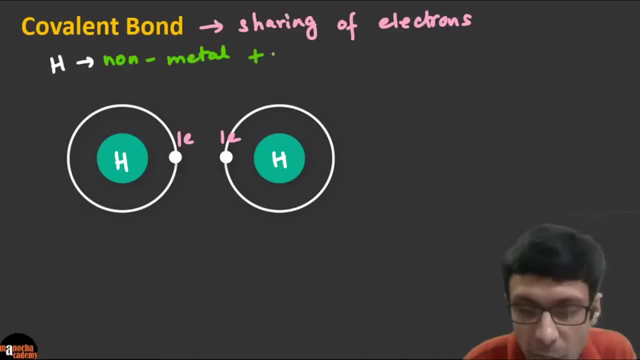 So a non metal and plus a non metal atom will give us a covalent bond. And let's take a look why. OK, so this gives us a covalent bond, Because let's see why they will be. So how will they get the stability? 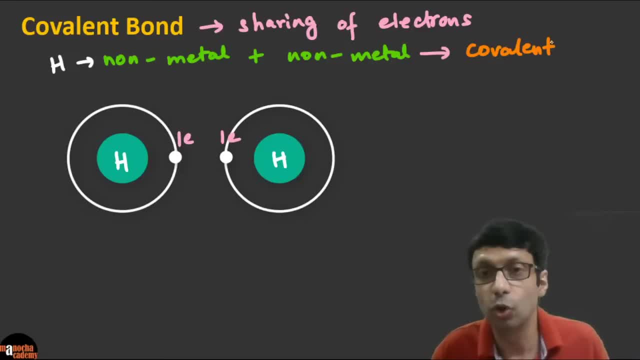 So you can see that first, hydrogen atom says to to gain stability. It wants to get to the duplicate state, Right. So that's an option here, either to get to the duplicate state by gaining the electron, or maybe it says, I want to lose it and just become an ion, Right, Same for the other one. 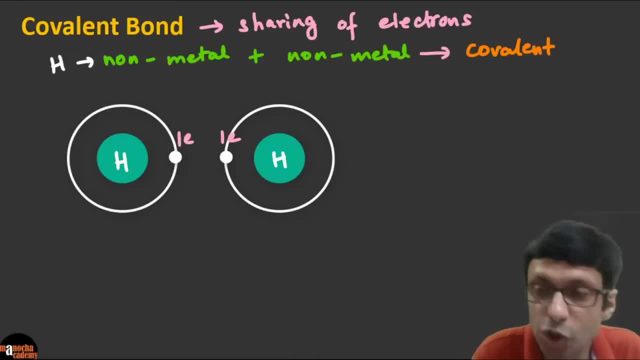 So what these guys end up doing is they end up sharing the electron because the non metals they don't want to lose the, they want to gain electron. OK, Right, Can you see that? OK, so great to hear that you guys are enjoying the class. 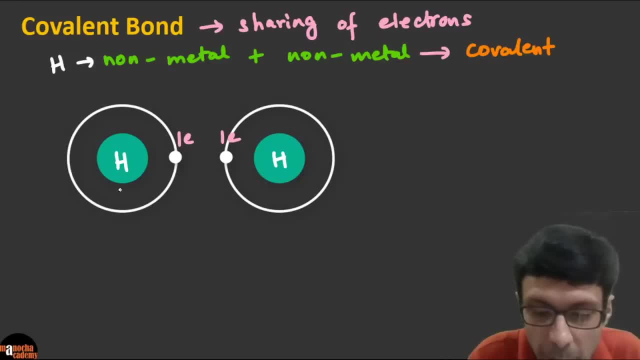 Thanks a lot, guys. So here can you see that the both these are non metal atoms and they want to. they don't want to lose the electron, right? You know, non metals want to gain an electron and here both are non metals. 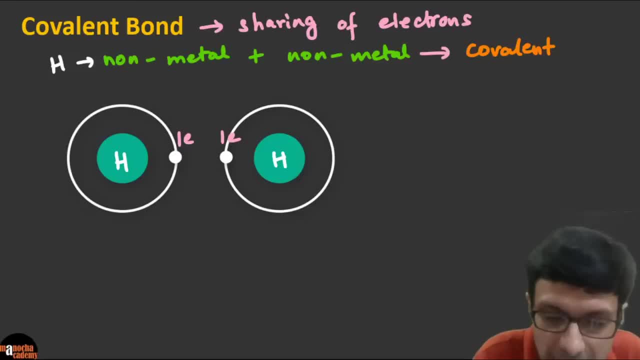 So they end up sharing the electron. and if they share this electron, Right, Right, So let's say I'll just remove the one electron here, the name. So if these electrons end up getting shared with each other, OK, so what is the meaning of sharing that? this electron is going to be present. 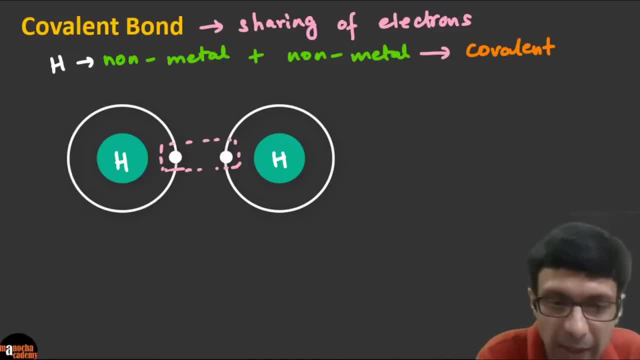 for this atom and for the other. OK, so we can represent this thing like this, you know. so the sharing of the electrons can be shown like this: So here we have the hydrogen, So let's draw that hydrogen. here the nucleus. 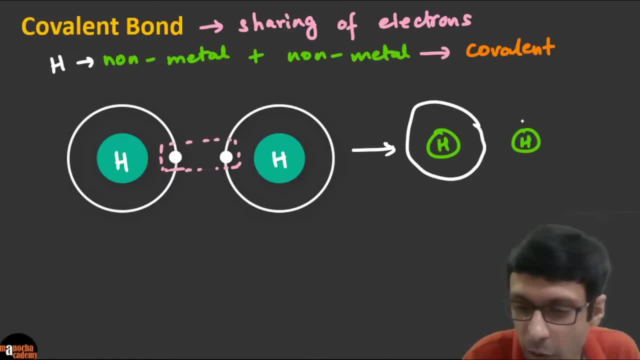 OK, and let's go ahead and draw the electron shell. OK, that's not a very nice circle, Let me try to draw a better one. OK, so here, and we can say: another one is here. So there can you see, and I'm going to show the electrons in pink color here. 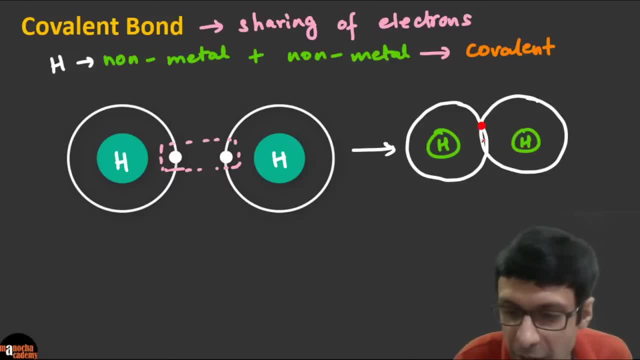 Let me use another color, let's say red here. OK, and so they end up sharing the electron, So it forms a shared pair of electron, And now these two electrons are sort of present in both. They're revolving around both the atoms. 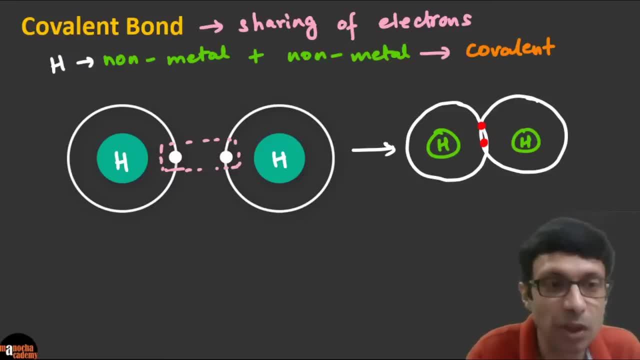 So what is hydrogen? Now, if you look at each of the atoms, how many electrons does each atom have? now? Can you tell me? So now, if you look at this sharing right, how many electrons does each atom have after sharing? So come on, guys, can you see that? 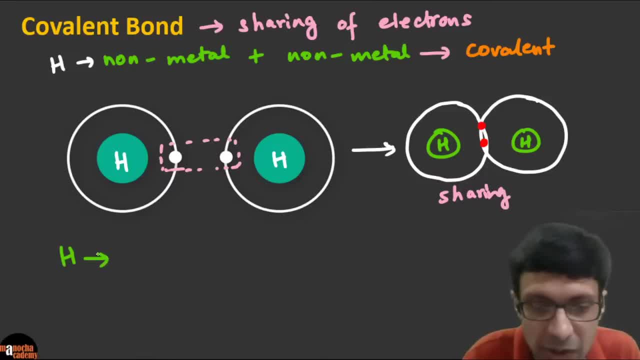 So each hydrogen atom, after sharing it, has two electrons. Do you guys agree with me? Very good, Right. I see Mary says two Right, Excellent guys, OK, So both of them end up having two electrons, Right, And this is so. they are getting to the 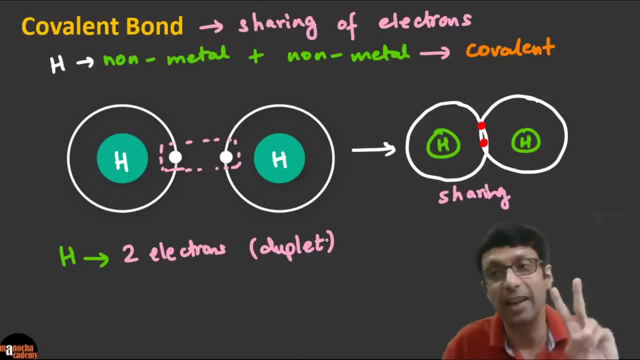 duplicate rule, because you know, if there's only one shell and it has two electrons, it is the duplicate rule which helium has Right. So they've got to The helium configuration of the duplicate configuration, And so it's very stable. 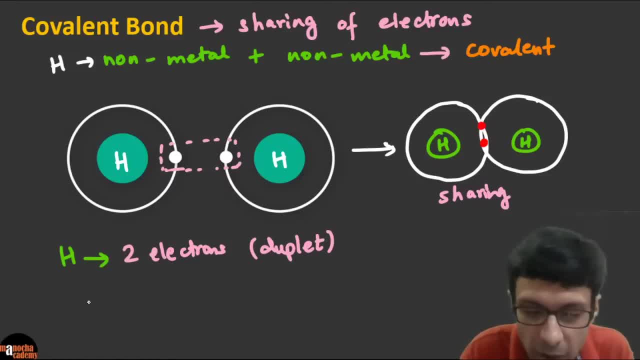 And there you can see. that is why the hydrogen molecule is basically H2.. Can you see? So what is formed is? we show the covalent bond using this line right, or what we call in chemistry as the stick Right. So the chemical bond is shown with this line. 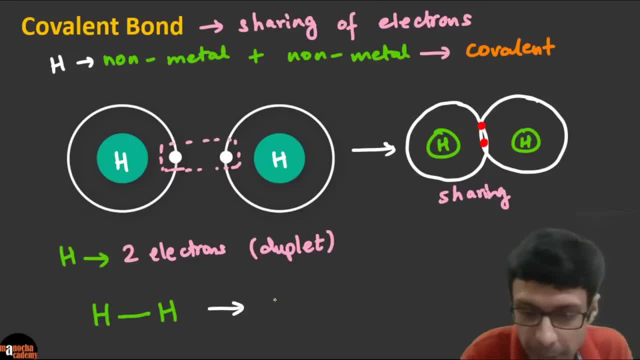 And so, basically, what we have is the hydrogen molecule. Right, Guys? can you see? this is the bond which I've shown with the green line here. Right? So this is the bond between the hydrogen atoms. OK, And this bond contains one pair of shared electrons. 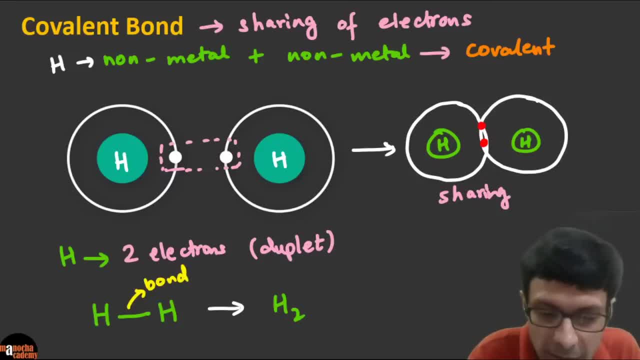 OK, So very important to know. That is why this is known as a single covalent bond. Let's write that down: Single covalent- OK, Why single covalent? There are two electrons, So that doesn't make it a double covalent. 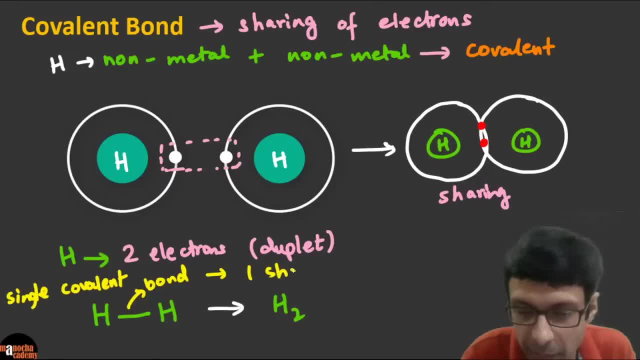 It's a single covalent because one shared pair of electrons- Right. So one shared pair of electrons Here, guys, can you see that? So this is how the hydrogen molecule Right. So do you know the H2? I think all of you know. the hydrogen molecule is represented with the H2.. 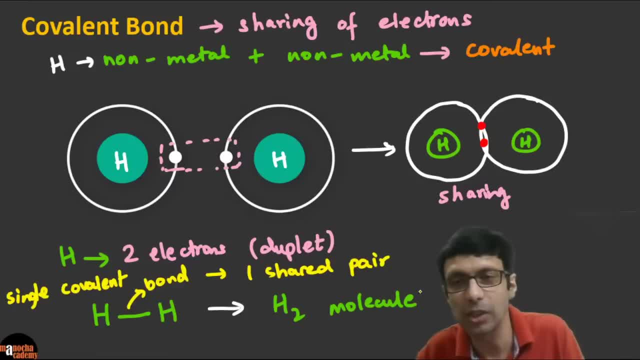 And now you know why it is H2? Because each hydrogen atom is not so stable, It has only one electron, But when two hydrogen, when these two hydrogen friends get together, they end up sharing that electron, Right. So both of them, it's like you know. 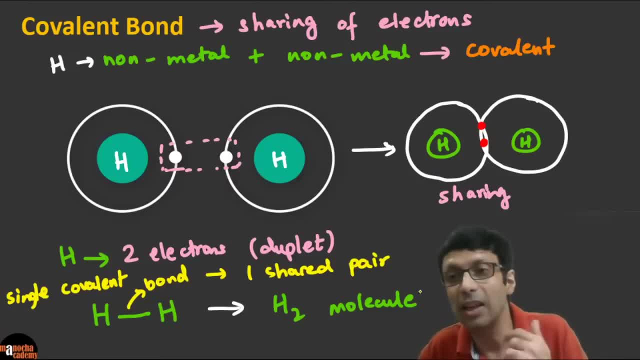 you are sharing chocolates with your friend. Sharing is caring. So here, each hydrogen atom is not holding this electron, It allows the other one also to have it, And so it's a win- win situation. Both get two electrons, and that is how we get H2.. 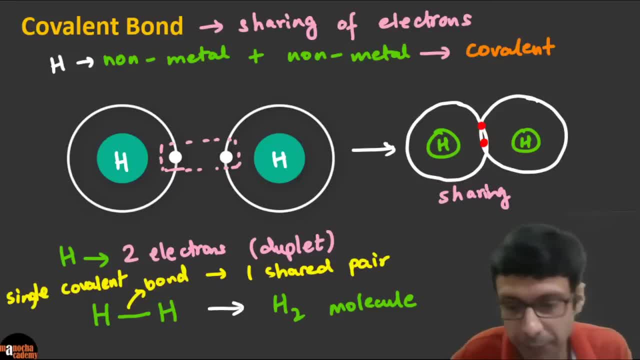 OK, super clear. And that is how you have the, the H2 molecule, Right. And now how we let's go ahead and try to draw it in its electron dot structure. So here we shown the simple way Right. So how do we draw the electron dot structure of this? 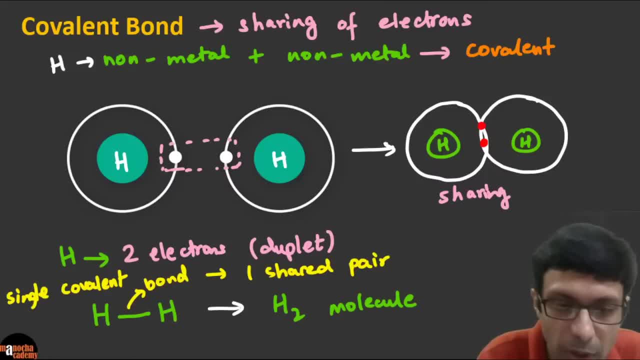 Very simple. Let's go ahead and do that here, Right guys. So let's say: this: is: we draw hydrogen. It has only one electron, So it's going to be H, and the other atom is also hydrogen. This time I'm not going to use cross, Right? 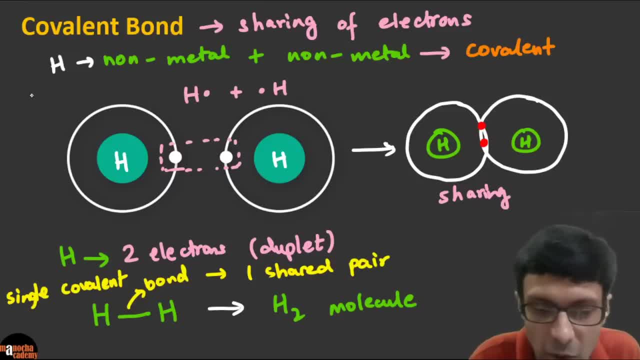 Because it's the same atom, Right? So I'm using dots here, Can you see? So I'm drawing the dot structure here for you guys. So dot structure, OK, so H dot and H dot, And so then when you, when they basically combine, 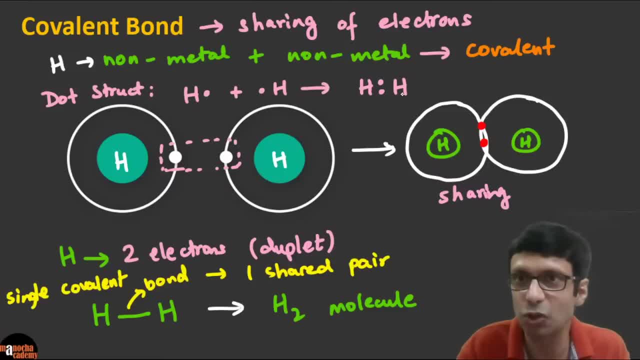 Right, You're basically going to get a situation like this. Right, It's going to share, So we write it close to each other, We write it in the center, And now you guys can even draw the circles to check the duplet rule is getting. 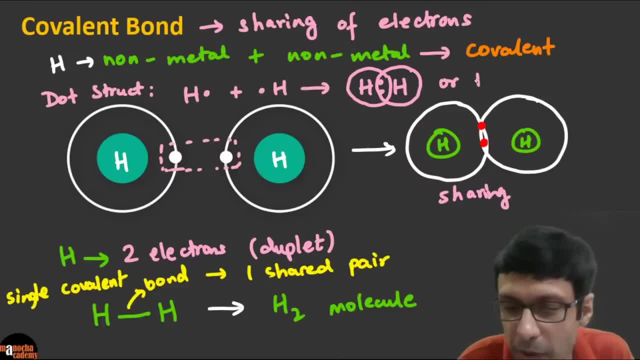 followed Right. So some teachers ask you to draw that, Or you can simply represent it, like we saw, as this: So this is basically our hydrogen covalent bond with a single covalent bond, Clear guys. So this is how you do the dot structure. 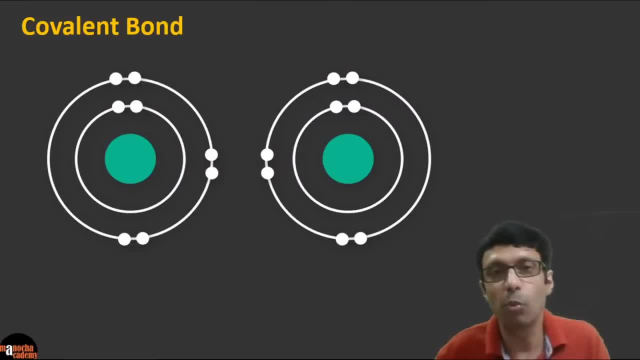 And let's go ahead and practice it for other atoms also. OK, so here, what do we have here? Can you see what do you have? Which atom do you have on your screen? And one interesting thing to note: I'm now starting to show the 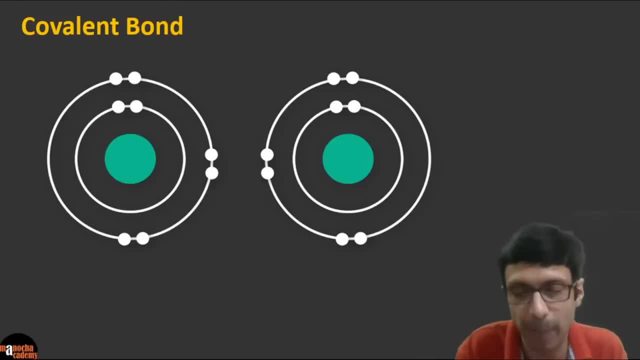 electron dots in the electrons in pairs. Can you see, guys, They are shown usually because the electrons they exist in pairs. So can you see that? And you know which atom is this? It has basically a configuration of two comma, Can you see that? 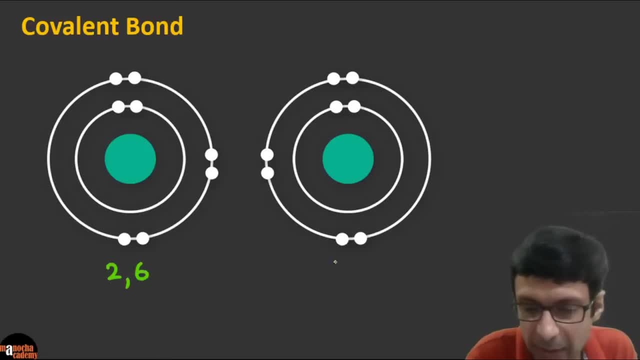 It's basically two electrons in the partial comma six, Right Two comma six. So, guys, can you tell me which atom is this? Very good, Varun says oxygen, Above says oxygen. Excellent, guys, Shomen Mukherjee. 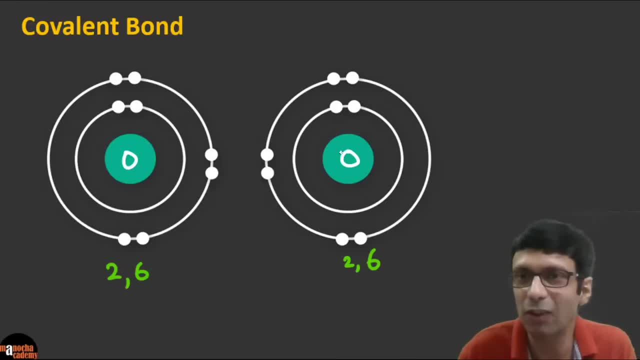 Very good guys. So this is clearly oxygen. So you should know your electron configuration or atomic numbers. It has eight electrons right. And now oxygen guys. What is oxygen? Metal, nonmetal- Please think that That's very important. What is oxygen? 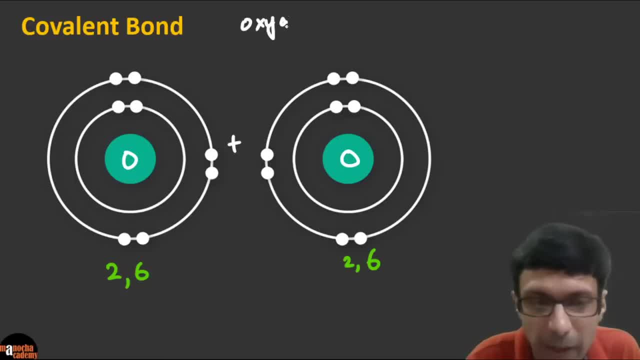 Oxygen, guys, you know, is a. what is oxygen? Can you tell me? Is it a metal or a nonmetal? Very important to think in your mind. So oxygen, Very good, It's a nonmetal, right, Oxygen is a gas and nonmetals. 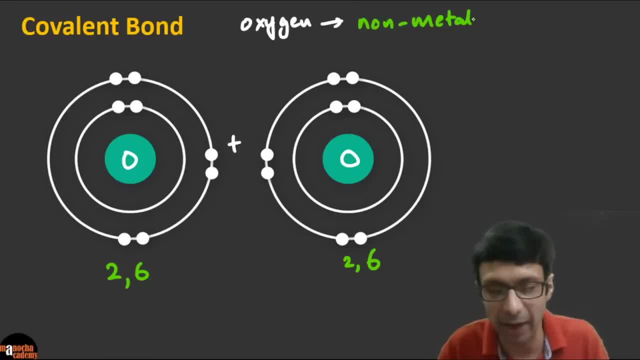 They form covalent bond. Excellent. They end up sharing the electron. OK, And which electron they will end up sharing. So can you see, oxygen needs two more electrons, right? It needs plus two here, plus two here to get to the octet, right? 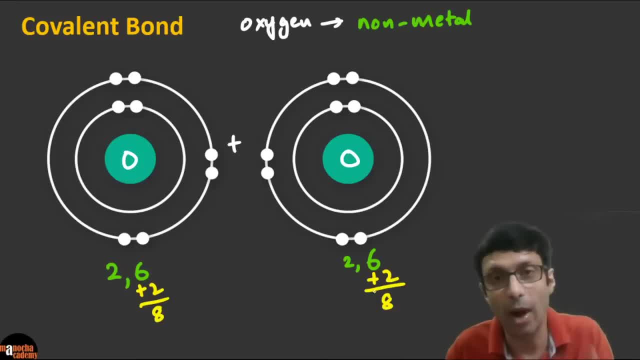 To get to eight in the outermost shell. So it will not end up sharing one electron each, It'll end up sharing two each, right. So we'll have these guys being shared. So let's remove that plus And basically oxygen will end up sharing these pairs, right? 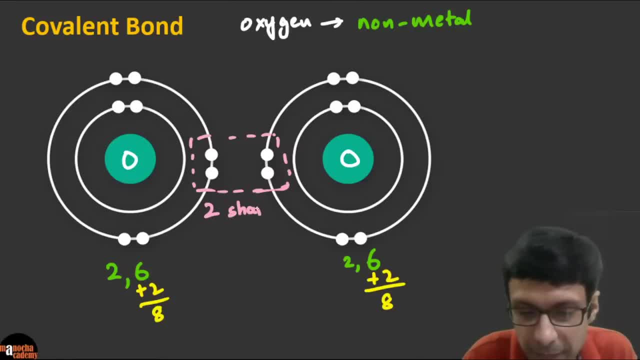 So there will be two shared pairs of electrons From each atom. Can you guys see that Right? So that is how. And can you see after sharing? So let's draw its electron dot structure. Very simple, So we're going to look right. 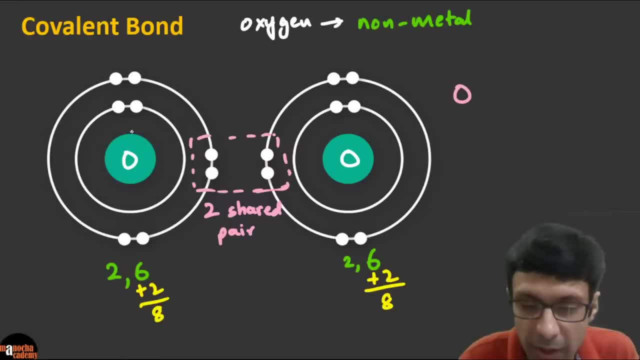 Oxygen first. So oxygen, Right. And so again, we'll draw only the valence electrons. Don't draw all of them, because electron dot structure is a simplification. So we'll do one, two, three, four, five, six. 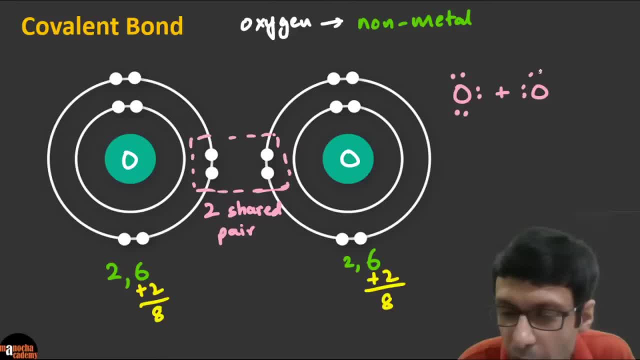 OK, And plus here one, two, three, four, five, six. And notice we are writing this two together Because we're writing them close by so that they're ready for sharing, rather than writing them on the other side. So that's why they're written close to each other, these two shared pairs. 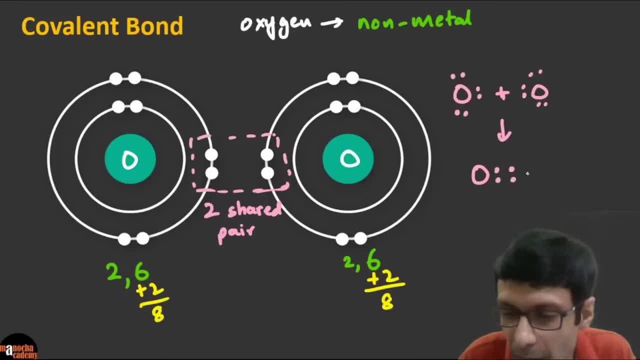 So if you draw it again, it's going to look something like this- right, And I'm using only dots because it's the same atom. OK, so it's a bond between the similar atoms And if you like, guys, you can also show. it's the entire octet rule. 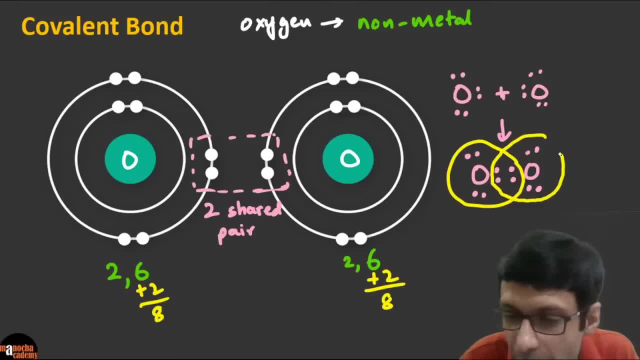 So you can draw that also. I'm showing it in yellow here. So can you see now after sharing, if you look at each of those yellow circles, how many electrons for each atom? Eight, OK, so it's going to become two comma eight. 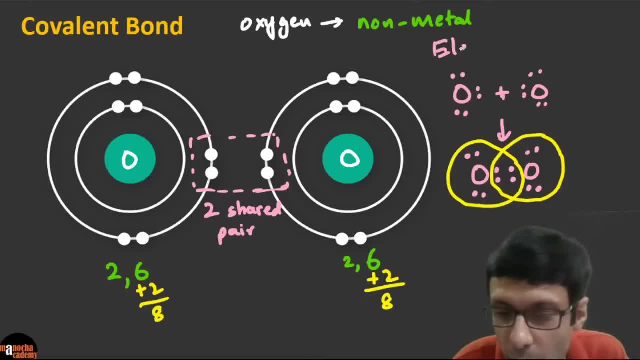 This is how you show the electron dot structure for covalent bonds: Right Electron dot structure. Can you see that, guys? Very simple, I've shown you, And so the next step will be to show it with the stick bonds. 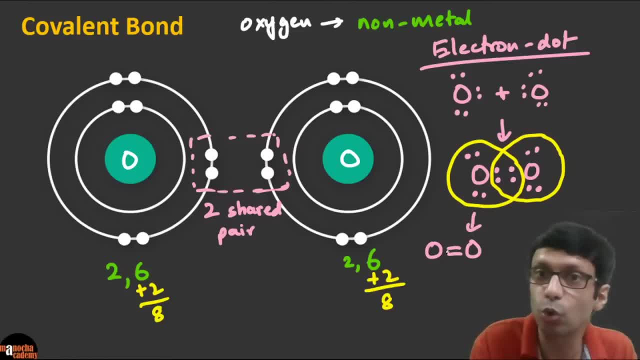 So oxygen will have two sticks right, Because there are two shared pairs. Can you see that? And this is what forms our oxygen molecule, O2.. So, guys, do you see it? And so, therefore, oxygen is basically having a double covalent bond. 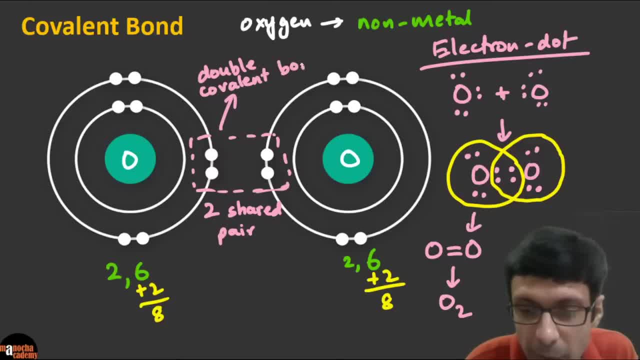 Double covalent bond. Why double covalent? Because oxygen and oxygen when they combine, right? I'll just erase these for now, right? So after sharing, it's basically of this form, right? Oxygen and oxygen is having two sticks right. 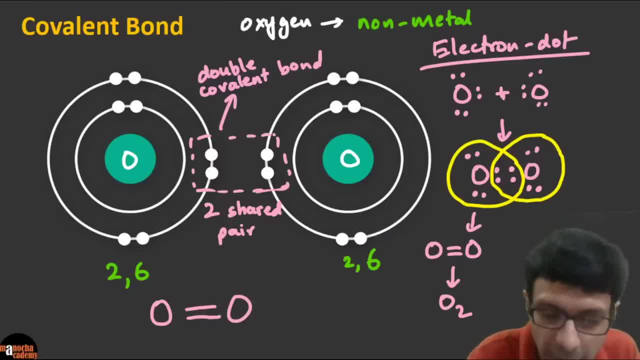 So there are two covalent bonds between the atoms. Guys, can you see that? Very important. This is our double covalent bond, Right? So very good. So covalent bonds can be of different types: Single covalent, double covalent. 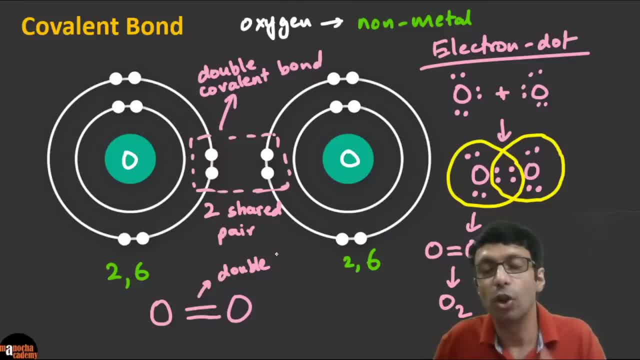 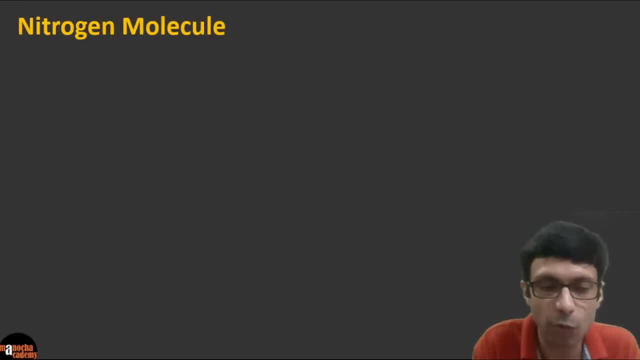 They can be also triple covalent, Right? So can you see that? Because you are having a two shared pair of electrons. Excellent, guys. So simple. And let's take a look at a nitrogen molecule. So, guys, are you familiar with the nitrogen molecule? 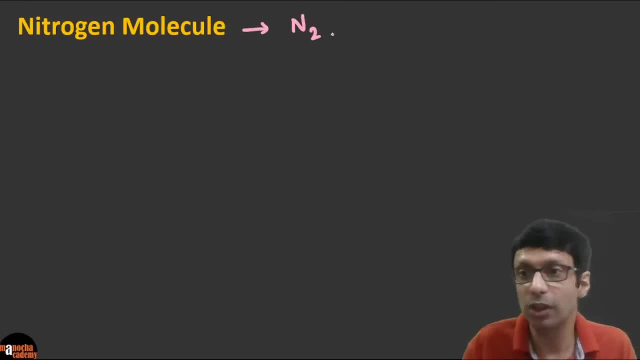 Again. first thing: nitrogen is N2, right, And nitrogen is a non-metal, right? You guys know, nitrogen is a non-metal, So it's between two non-metal atoms, right- N2, right. So definitely nitrogen is forming a covalent bond. 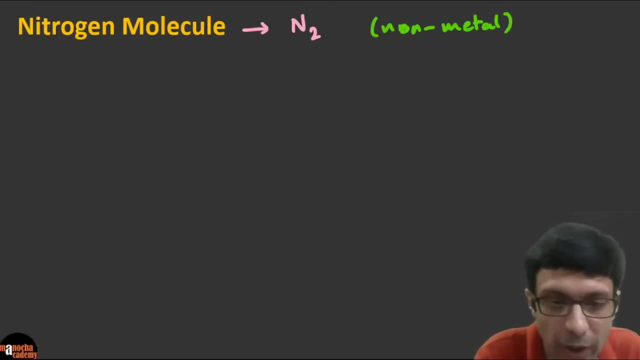 So how do we represent the simple electron dot structure? Come on, guys, let's go ahead and try. So nitrogen- basically, you know it has how many electrons. How many electrons does nitrogen have? It has seven total electrons, right? 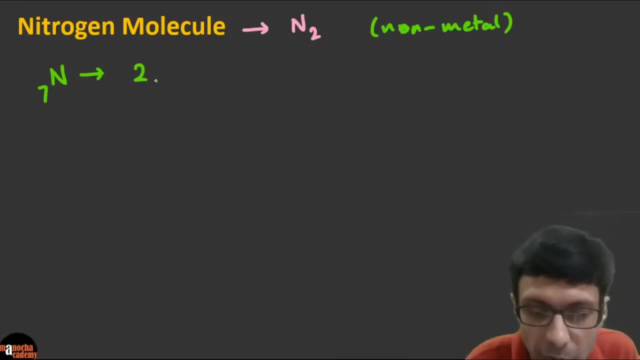 The atomic number is seven, guys, you know, And so the electron configuration is 2, 5.. Excellent, Excellent. I see a lot of you are writing 2, 5.. Great to know your atomic numbers. It really helps you in this bonding chapter. you know so that and you. 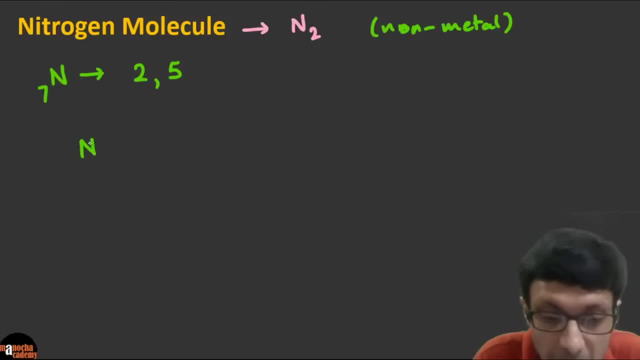 can easily derive the electron configuration based on that. So let's remember: it's important only to represent the valence electrons. Don't draw all 2, 5, because electron dot structure only the valence. you show that. that's the simplification. 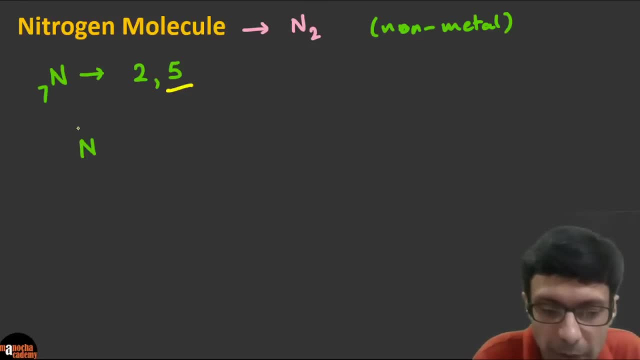 OK. so nitrogen, we know right, It's going to form this bond, So let's go ahead and draw. So 1, 2, 3, 4 and 5, right, I've represented like this. So let's say: I'm representing this thing and these are our five electrons. 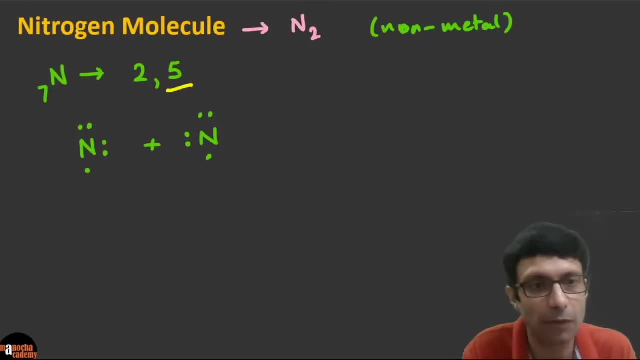 OK, but to gain stability, How many electrons does nitrogen need? Guys, can you tell me to get stability, How many does it need Each nitrogen molecule? Again, they're nonmetals. They don't want to give it away. 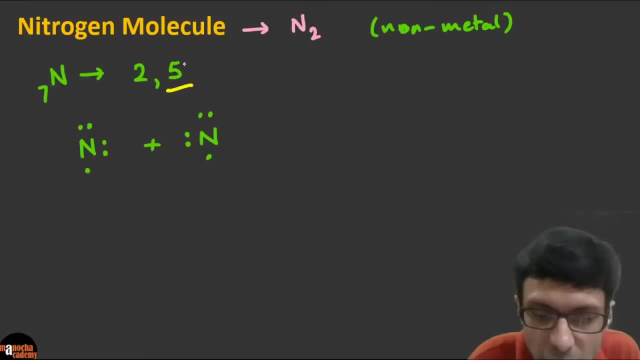 They want to share. So, to get to stability, it needs a plus three here, right? Yes, So it needs plus three over here, so that that will make it stable, Right, And that is why it wants to share three. So, rather than so, we want three electrons to be shared between the nitrogen. 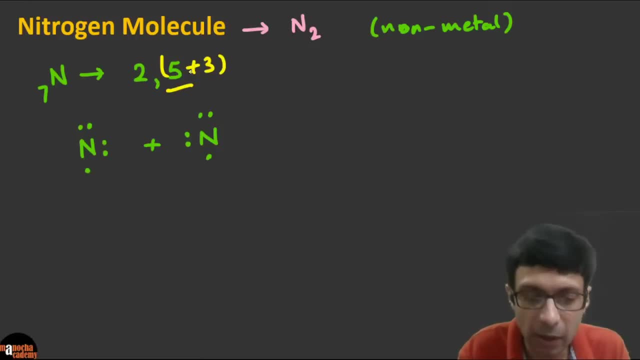 Excellent guys, A lot of you are writing three super. So please see, We are not going to represent this in this pair form. We are actually going to do some cheating here and represent it as a triplet. OK, so so that it's easy to show the sharing of these three electrons. 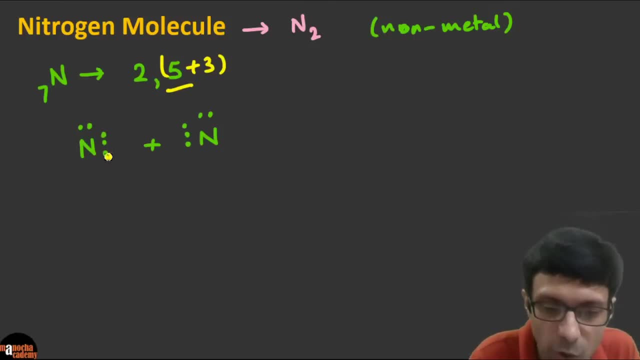 OK. so, guys, can you see I've modified my diagram and please take a look. Now I'm representing three dots here. OK, and they're using only dots because same type of atom. So the electron dot structure will look something like this: 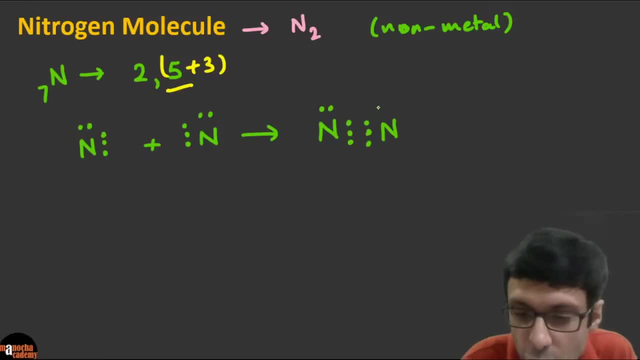 So you bring the atoms close to each other and then you're wanting to share the three electrons, So you put them in the center, three from here and three from here. And, guys, you can go ahead and draw the circles if you like that. 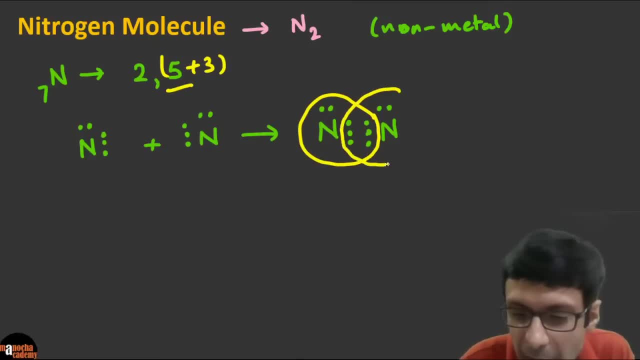 Or if your teacher asks you to do that, you please go ahead and draw that And there you can see. Can you see that each circle now has one, two, three, four, five, six, seven, eight electrons? Can you see that? Excellent guys. 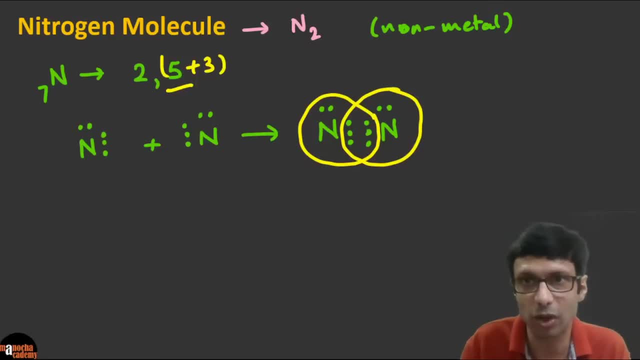 So nitrogen, this is how you represent the electron dot structure for the nitrogen molecule. Very important A lot of times this diagram comes in your test. OK, So this is basically. we can represent it as the triple bond. OK, so this is a triple bond here because there are three covalent bonds. 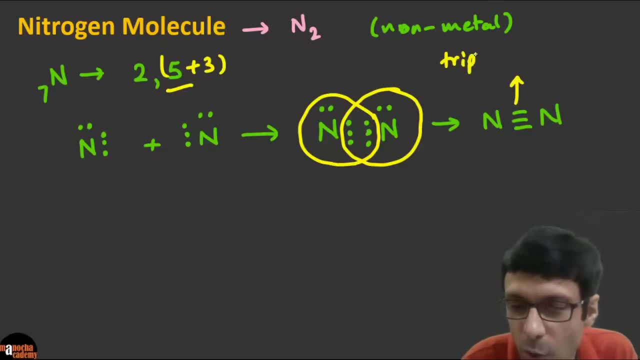 OK, so this is basically what we have here is a triple covalent bond. right, Triple covalent bond because why? There are three shared pairs, not three electrons. three shared pairs of electrons, Excellent, Chandan says triple covalent. 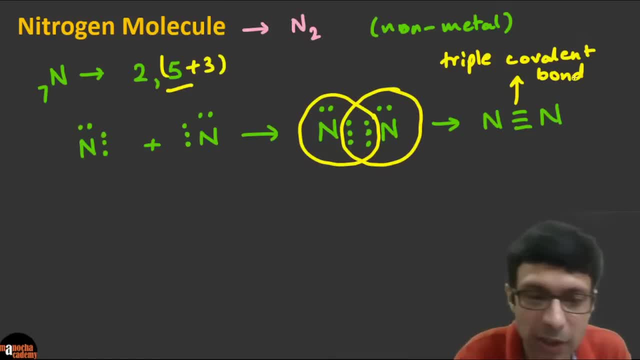 Superb guys. Vineet says that Very good, And so this is. finally we can say this is our N2 molecule. So it's good to write all the steps. in the first step, Show the atoms with the plus, you know. 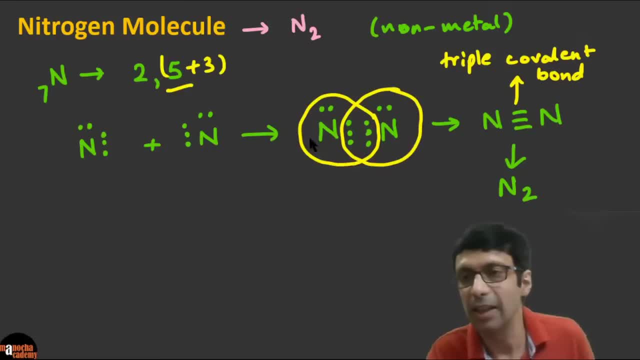 trying to join and draw only their valence electrons. in the next step, You can show them coming close to each other and drawing their the circles to show the octet rule being satisfied. And then you can go ahead and complete and finish off by showing the the triple covalent bond. 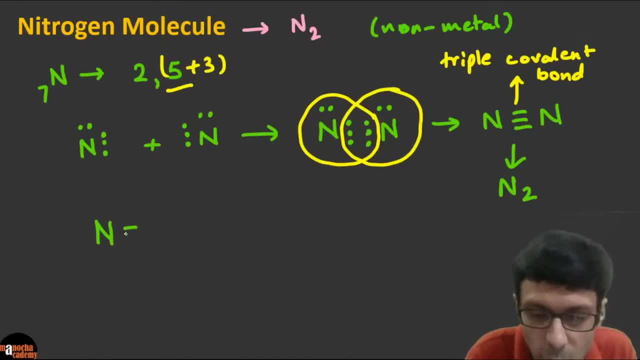 And so this is the simplification right. So when we write it like this, we are not showing all the electrons, We are just showing that nitrogen has the triple bond and clearly you can see now each one, each nitrogen atom is having the octet. 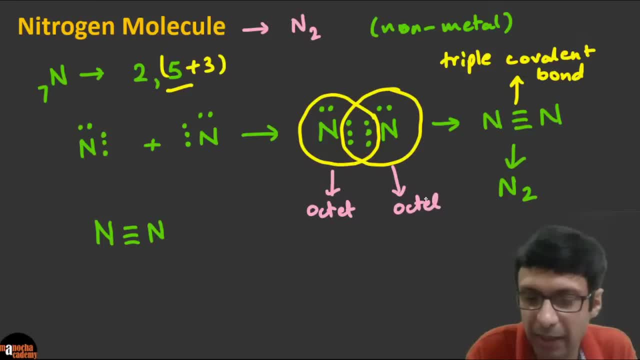 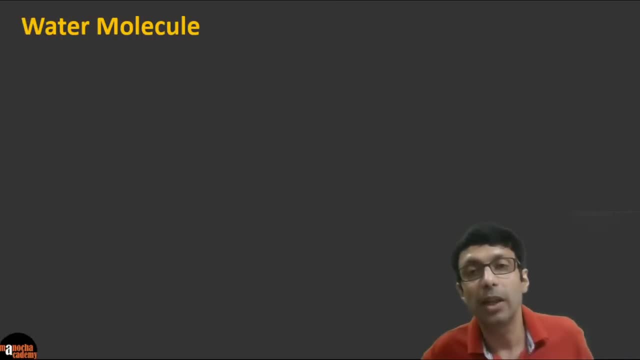 Can you see that? eight, eight, right, So each one is getting its octet here. Excellent guys, Superb. OK, and guys. now can you tell me, based on our knowledge, what is going to be the kind of bonding in a water molecule, right? 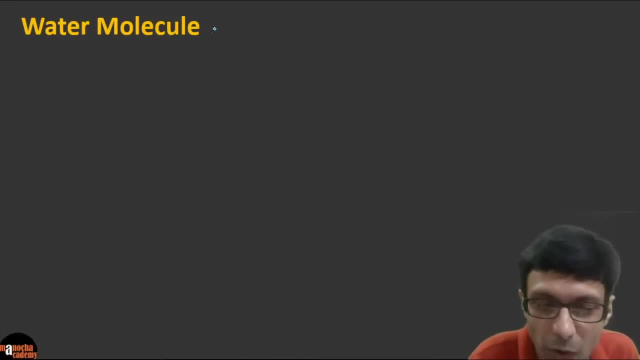 Everybody knows about water, right? So who can tell me what will be the bonding in water molecule? So here we are, talking about water, which you know is H2O. So is it going to be? So, guys, come on, be James Bond. 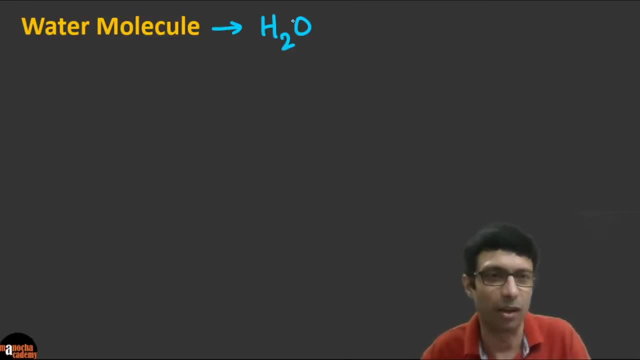 Is it? the main question is: is it ionic or covalent? All of you know the formula: water right H2O. So how do you understand? So again, don't learn it up. You know you can easily derive it because you guys, you know hydrogen. 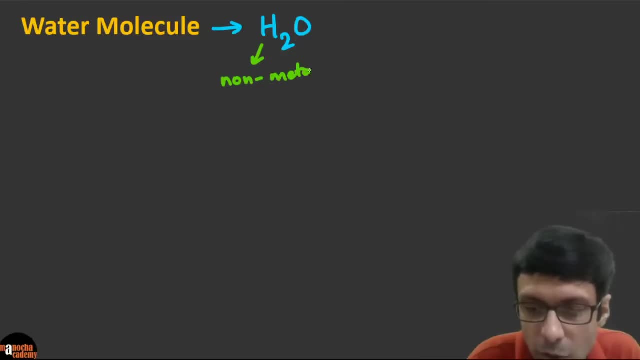 It's a gas, as we discussed, It's a nonmetal right. So hydrogen is a nonmetal. What about oxygen? Oxygen is also nonmetal right. So there's nothing to learn here, Just and all you need to know: nonmetal. 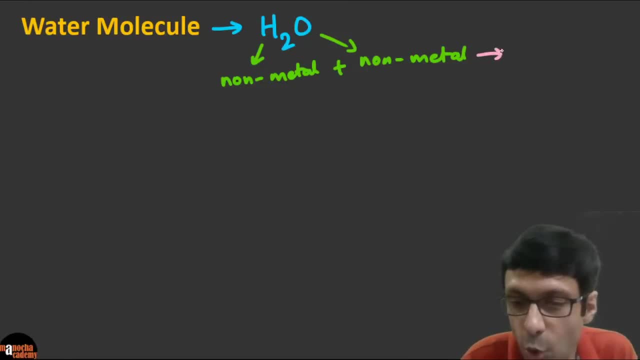 and nonmetal right. They together form a covalent bond. because you know the nonmetals, they don't want to give away the electron they want to accept. But you can't have two guys accepting right, So you cannot have a transfer here. 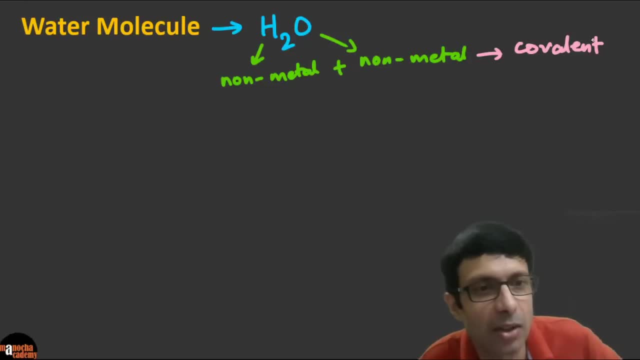 It's going to be a sharing- Excellent. I see. Gauri Bagga has the right answer, right. Rajna has the right answer, Excellent. Sumangal Chandra covalent bond- right. Excellent. guys, It is not ionic. 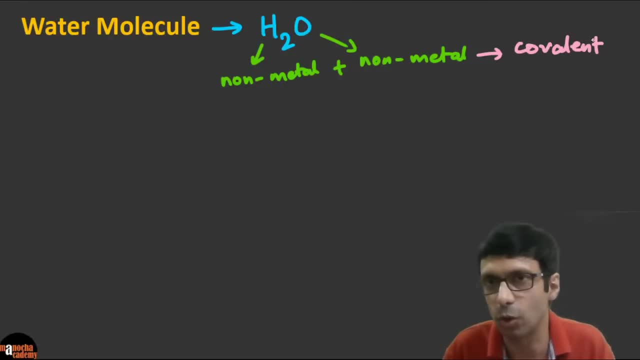 OK, why? Because hydrogen is a nonmetal. Oxygen is also a nonmetal, OK, So don't think H as H plus. OK, I know some of you are thinking you know of acids and all. Don't think of H plus. 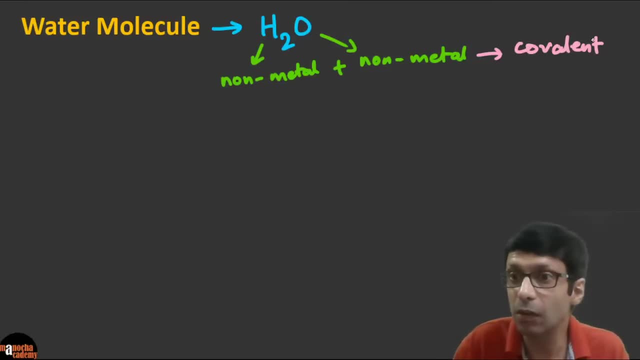 It is clearly a covalent bond. OK, and now we can see whether it's going to be single covalent, double covalent, triple covalent. Let's go ahead and try to draw the electron dot structure of this. 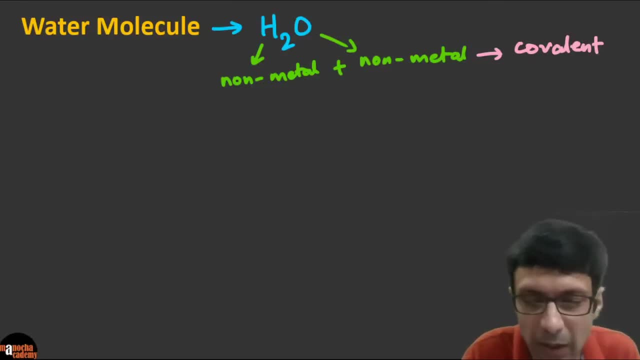 Come on, guys. So this is really exciting, right, We are analyzing the molecular structure of these, So let's go ahead and draw hydrogen and oxygen. OK, so hydrogen I'm going to represent in the pink color here, So clearly. 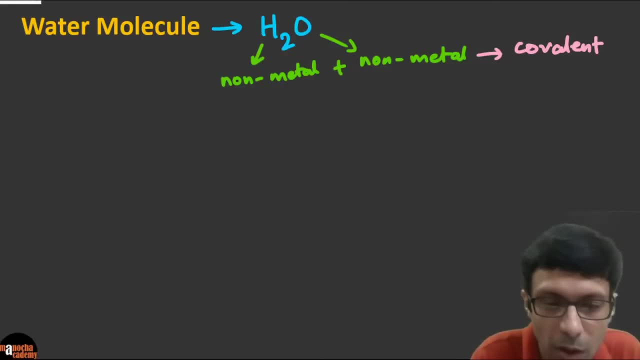 Let's put oxygen in the middle here, right? So you know the for oxygen it's going to be O, right, And here, actually, you know, let me show you a trick. Usually you can cheat rather than going ahead to draw the bonding structure. 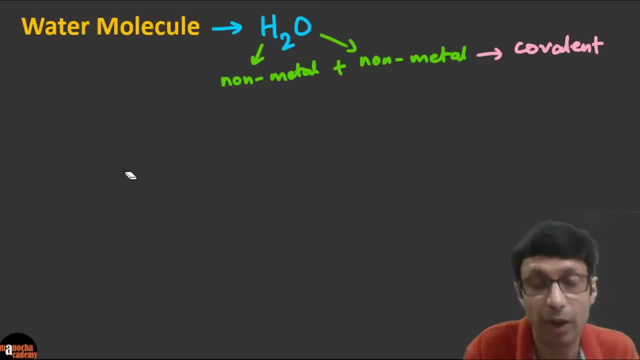 You can first think of what is going to be the type of bond. So let me tell you a very important trick for that right. So if you take a look at oxygen, right, oxygen has a valency. So why is it forming water? 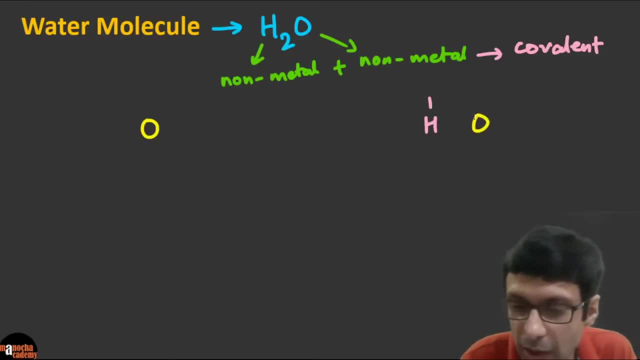 Because hydrogen, you know, has valency one and oxygen has valency two. What is the meaning of valency two? It can form two bonds right with hydrogen here. So the structure you know is going to end up something like this: 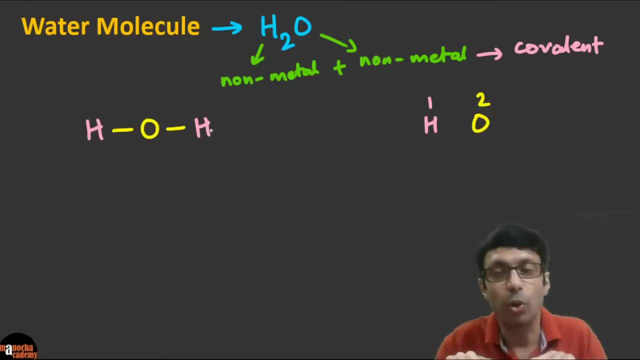 Do you guys agree? Because oxygen has valency two, So it combines with two hydrogen And if you look at these bonds you can see oxygen is having two covalent bonds, The two dashes. Why? Because valency is two Hydrogen. each hydrogen atom can have only one bond. 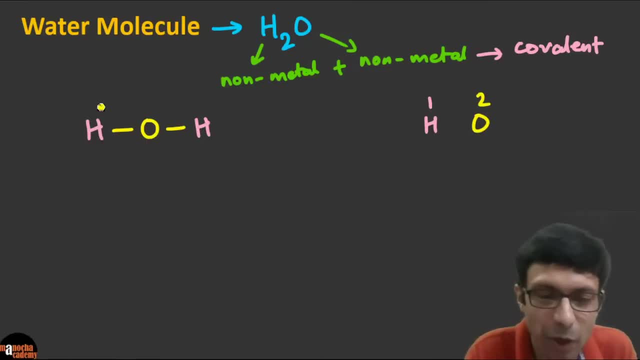 Very good, A lot of you are writing HOH with the dashes. Excellent, right, Because oxygen has valency two, So two bonds, and each hydrogen atom has only one dash because valency one. So you can actually do the reverse: First think of the structure, then you draw it. 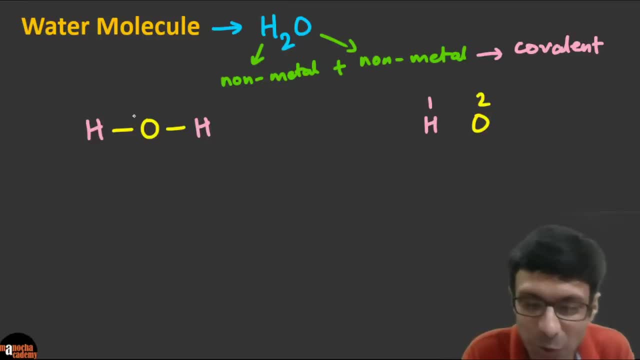 It's much easier, right, Rather than starting with the electron dots and all. So you know your answer is going to be of this form, or you know in some books you might see. you know the water molecule has a shape. 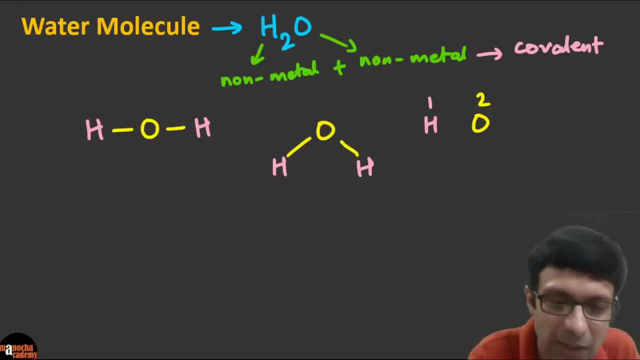 something like this: right, But here the shape is not important. So I think this is enough for this discussion, that water is a structure like this, So let's quickly go ahead and draw its electron dot structure. So basically oxygen, you know, has six. 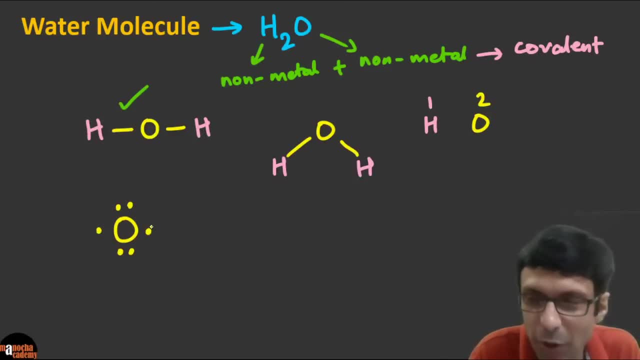 So we're going to keep one, two, three, four and one on either side, because we know it's going to share with hydrogen right, And we're going to draw hydrogen on this side And hydrogen is going to have one electron right. 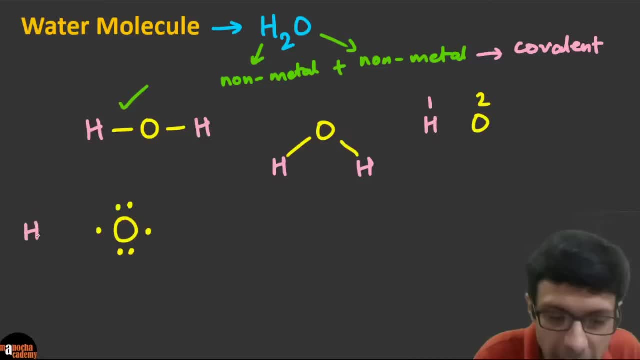 Oops, too close. So let's go ahead and draw hydrogen this side, So hydrogen, OK, And another hydrogen on this side, with a single electron, And that I've shown with the cross because it's a different atom, OK. So if we combine these, what are we going to get, guys? 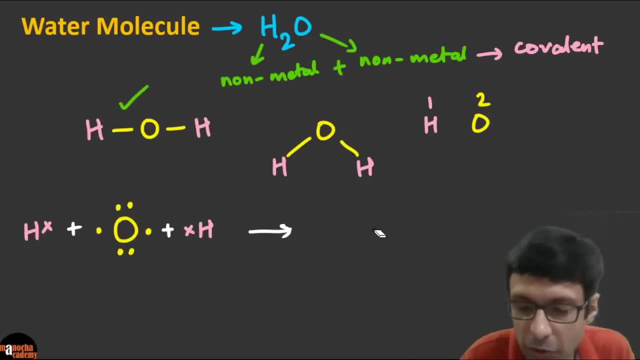 So oxygen is going to become like. so we're going to represent oxygen like this Right And with this electrons and hydrogen. you put it close to that and you're going to start with the pink color right. So hydrogen we're going to have here. 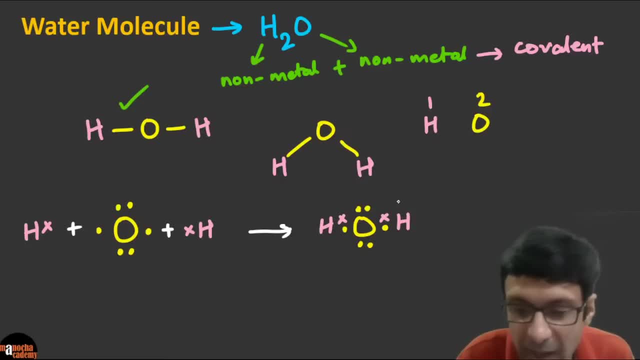 and we're going to mark its cross right, the electron with its cross, And there you can see- guys, take a careful look- Can you see that oxygen now has its octet? So if you draw the circle around oxygen, oxygen has its octet and each hydrogen guy has its duplicate. 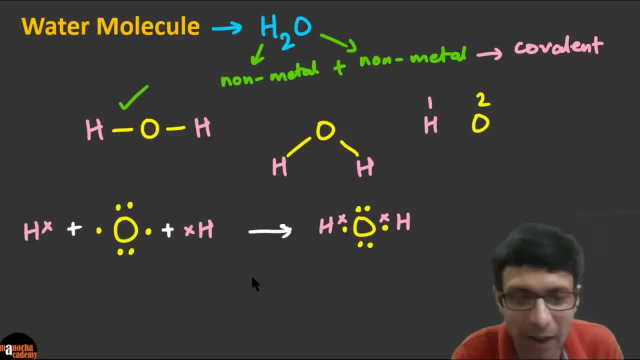 OK, it's getting really messy, I think, So let me draw that again a little more carefully. OK, so oxygen, can you see, has its octet here right, And hydrogens: each hydrogen has its duplicate. OK, you can leave it as that also, even without drawing these circles. 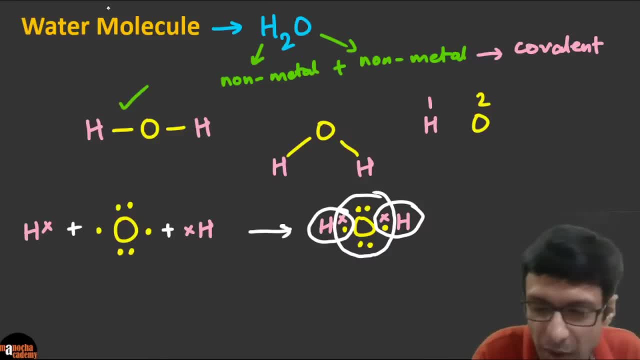 So that is the structure of water And that is why the final form is this form. right, guys, So the final form is going to be of this form. And so now can you tell me single covalent, double covalent? 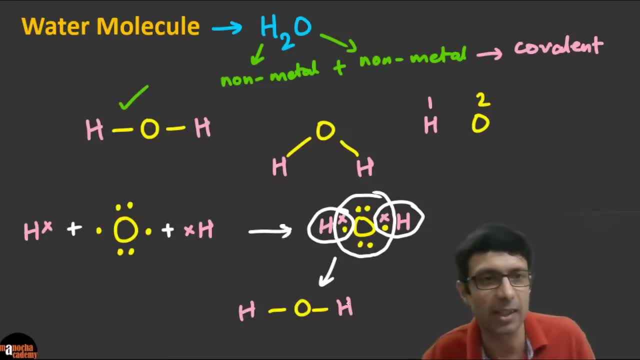 what is there? triple covalent? what is there in the water molecule? So who can tell me? guys, Come on, please try. OK, some of you are asking: is this for class 10?? It's important for class 9,, class 10.. 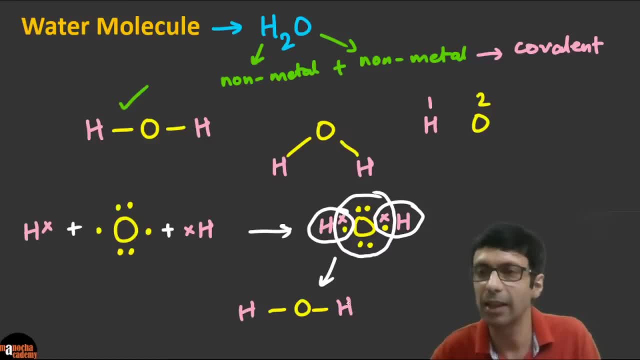 Some of you even have it in class 7 and 8.. But mostly students get this in class 9, 10, though I've seen a lot of students having this topic covered in class 7 and 8, including these electron diagrams. 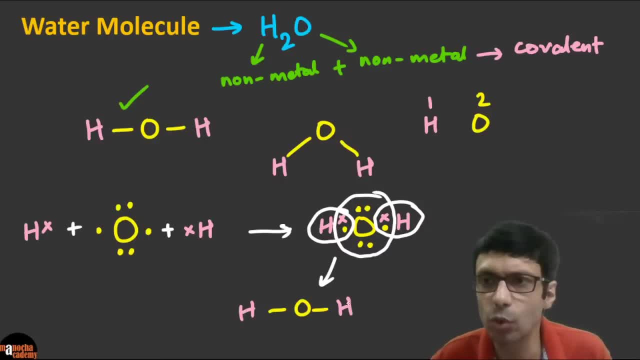 OK. so some of you are saying double covalent bond. I don't think I agree. Do you see a double covalent bonds? look something like this, guys: OK, so this is not double covalent, because double covalent should have a double bond, right. 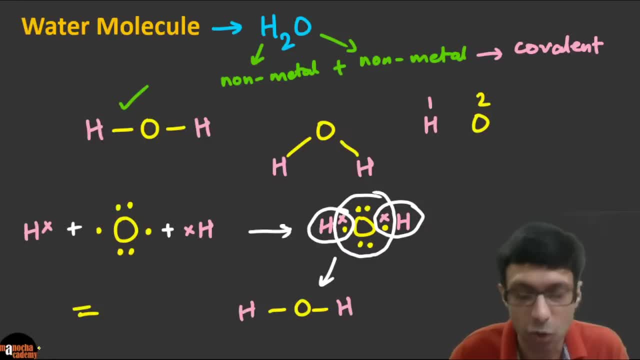 This is not a double bond. OK, this is not a triple bond. So please take a look. There are two. there are two single covalent bonds. Can you see that? Because there are only these single dashes, right? So there in this molecule, please take a careful look. 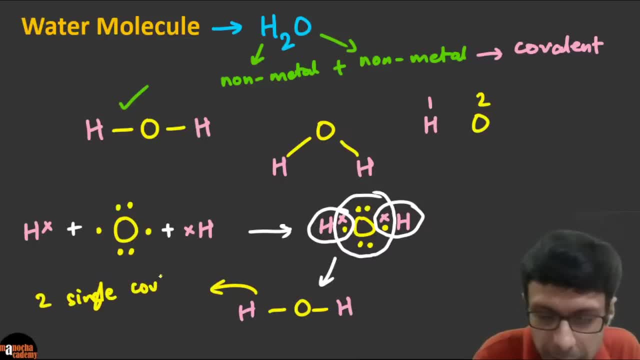 There are two single covalent bonds. Right, There are, there are two bonds, but each bond is one shared pair of electron. So this class has- sorry, this class, this molecule, has two single covalent bonds here, because can you see each one? 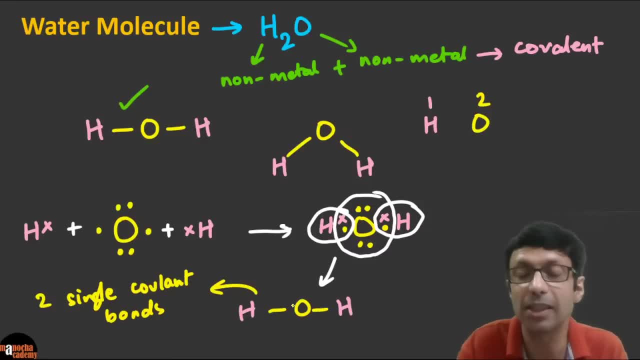 of them, right with the mark with the yellow dash, and the dash represents it's only used for covalent bonds, not for ionic bonds. It's special to these. OK guys, is that making sense to you? So this is how you draw the. 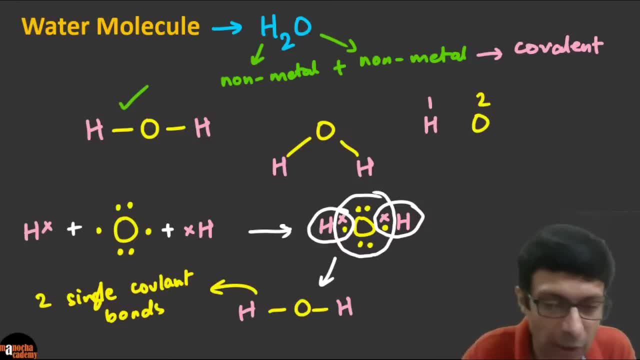 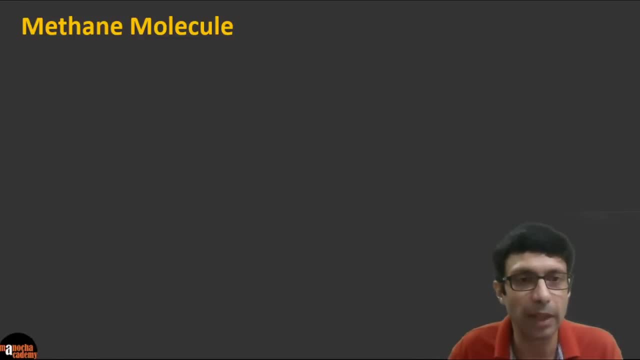 molecule of water, Excellent, Right. So two single covalent bonds. And, guys, do you know what is the formula of methane? So let's try another one, Right? So, guys, can you tell me what is the formula of methane? 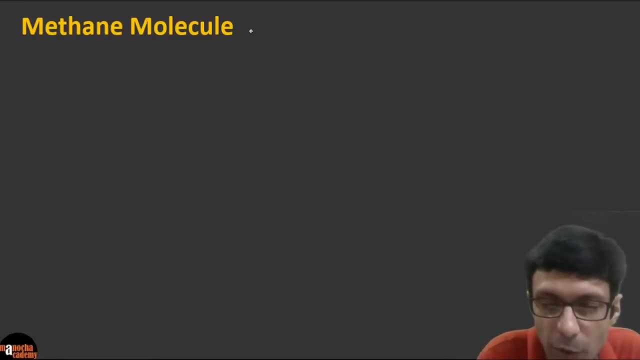 Come on, guys. So have you heard of this compound? What is methane's formula? Who can tell me here? Is this for CBSE or ICSE? It's important for both boards. The chemical bonding diagrams are there for ICSE and CBSE, right. 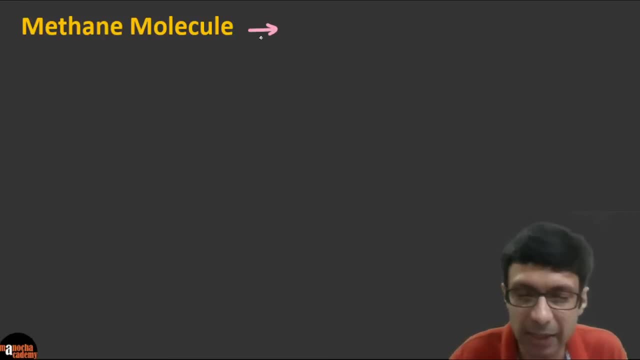 So again, it depends on your school which topic they're doing. Excellent guys, Excellent. Methane is CH4.. Superb, It's a compound of carbon and hydrogen. OK. so again the James Bond question: is it ionic or covalent? 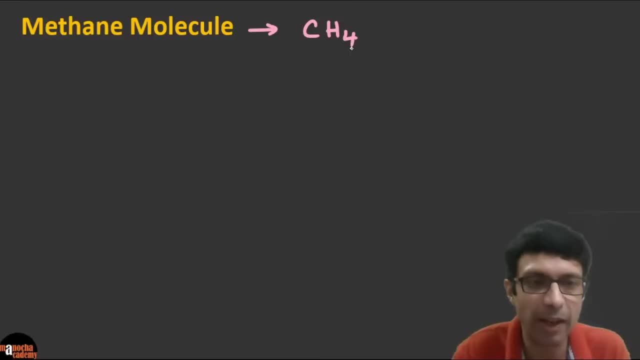 So who can tell me, is the methane molecule? is it going to be ionic or covalent? That's the key question here. right, Come on guys. So for methane molecule, is it going to be an ionic or covalent bond? 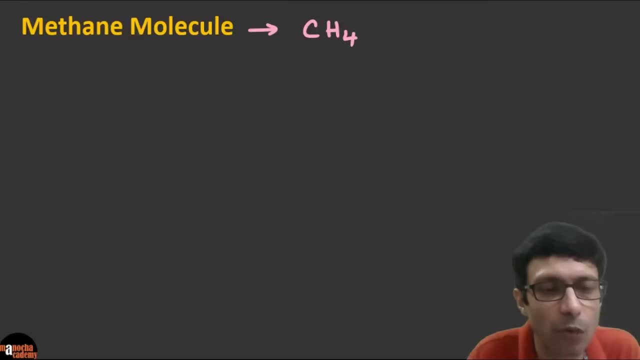 OK. Oswin says covalent right. I'm seeing some, mostly covalent. some are saying both OK. so carbon, you know, is a non-metal right. Hydrogen, as we discussed, is a non-metal right. 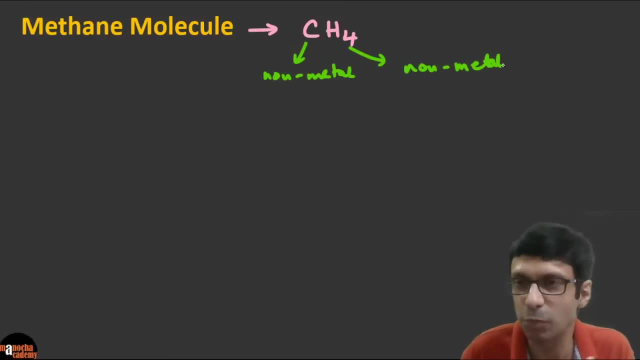 So clearly we are going to have a covalent bond. Excellent, guys, because between non-metal and non-metal this will be of a covalent bonding, So we know it's going to be sharing of electrons. Again, we can cheat here. 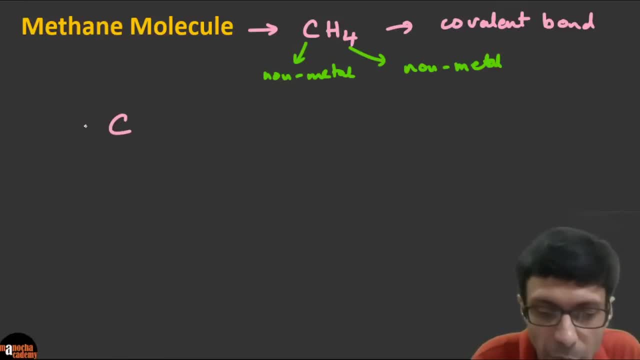 You know we can look at the structure first. So you know carbon has a valency of four right. So let's go ahead and draw the four dashes. if we call it right or sticks right, Four bonds for carbon and hydrogen has. 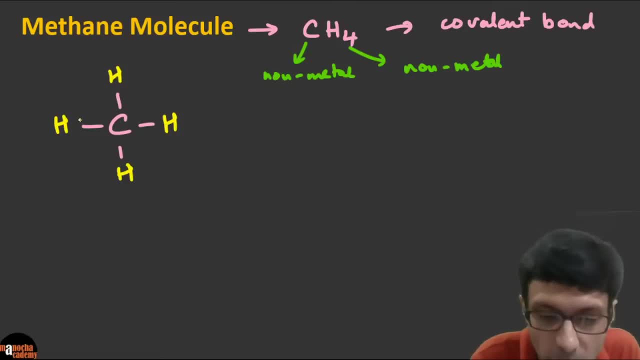 one, right? So for each hydrogen atom there's only one stick. You cannot have a situation like this. That'll be wrong. right? Because each hydrogen hydrogen has valency one. It can have only one bond, only one covalent bond- very important concept. 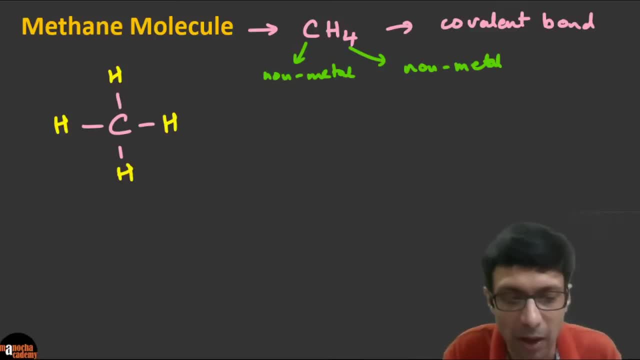 OK, so can you see this? Great guys, Great to hear you're enjoying this class. So, guys, if you haven't hit the like button, please hit it right now and do share it out with your friends so that we can have more folks on the live class. 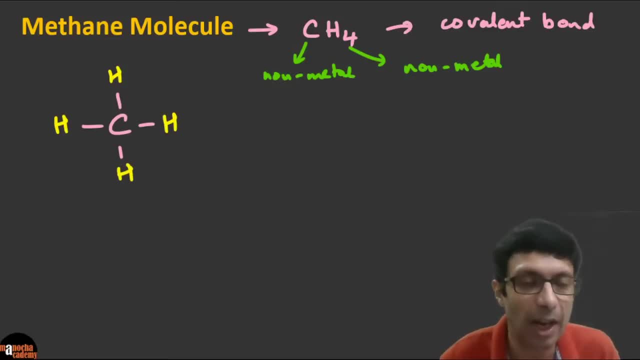 and watching our videos, and guys do check out our website, Manochacademycom. we've got awesome courses there for CBSE class nine and ten and also for ICSE class nine. So guys do check out our courses. We'll try to launch more courses as well. 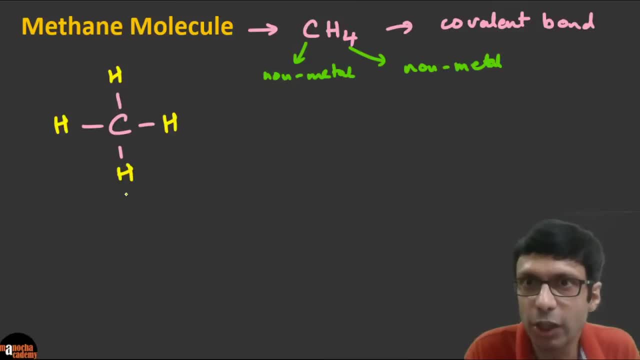 Thanks guys for the likes. So take a look here: Methane molecule, covalent bond, clearly, And can you do you agree with this structure? Carbon has valency four, So four bonds. Don't forget that Carbon valency four, tetravalent hydrogen valency one. 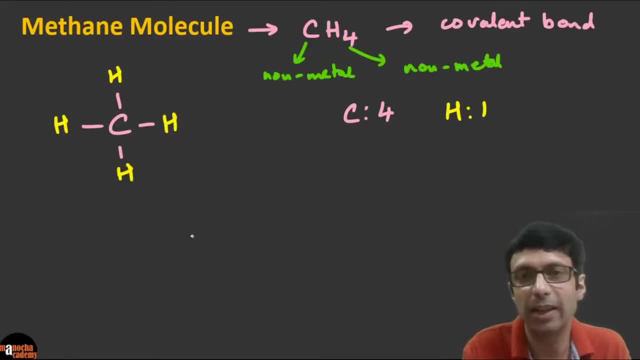 So this makes sense right Now. all we need to do, you know, translate this into its electron configuration. So carbon will have- it's going to have- four dots all around it, Right, Hydrogen: we can show with four, each with a cross. 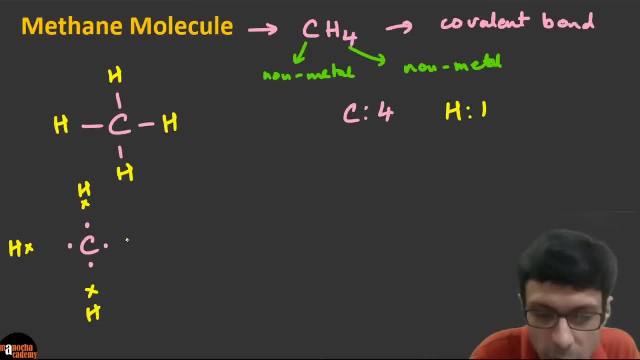 Right. So do you guys agree- And I'm going to put it on all the four sides so that they can combine nicely, And these guys are going to combine, you know, so that plus should be somewhere there, Right? OK, so the plus is here, Right? 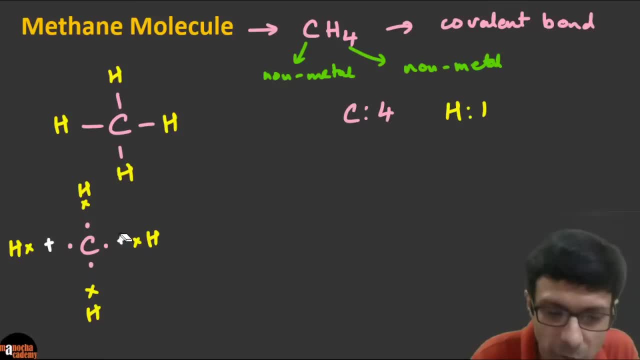 So these guys are going to combine with it, Or for now, let me leave out that plus, you know it's getting untidy, So you get the picture here and let's go ahead and draw the. let's bring them close to each other so that we can have the sharing of the electrons. 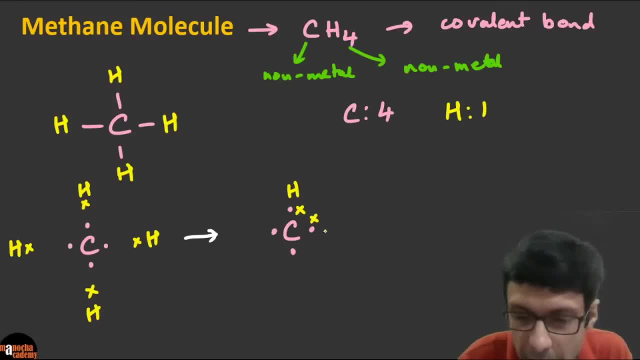 So the hydrogen atoms come here, close to the carbon and now see, like nice friends, They are sharing their electrons. Can you see that, guys? And clearly you can see carbon now I'm not going to draw the circle. Can you see? carbon has now eight electrons. 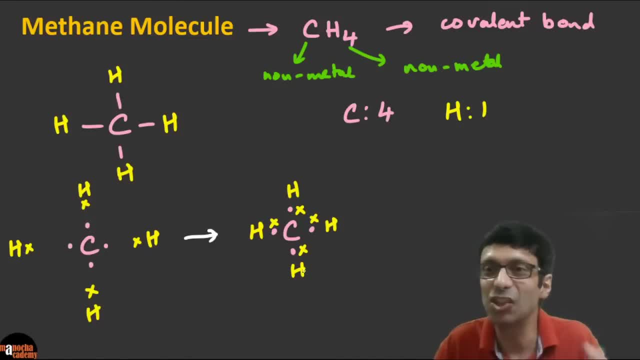 the four pink dots and the four yellow crosses. OK, and each hydrogen has two electrons. So you can see, hydrogen is now got to its duplicate. Each hydrogen atom has its duplicate state, Right? Oops, Not good, I've been writing, Let's write it again. 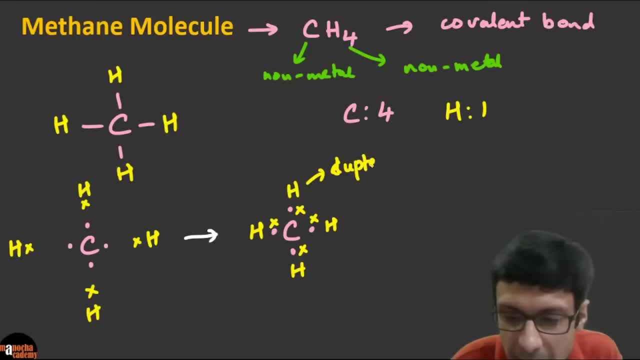 Each hydrogen atom is in its duplicate state, and the carbon is in the octet state Right. It has eight electrons. So see, that's why they've gained stability through sharing of electrons, And so the final structure is going to look like what we had drawn earlier. 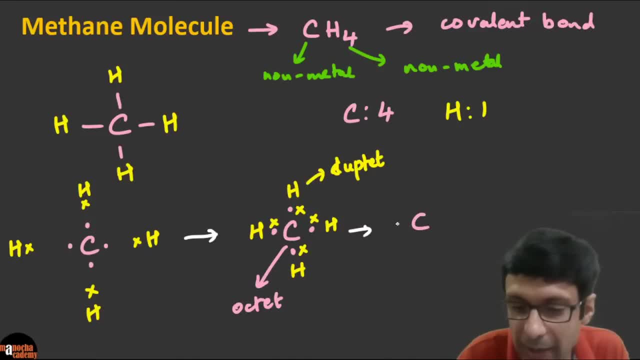 As I said, you guys can, you know, use the cheating or the back technique to first think of what is the structure, Then you draw the electrons. That's absolutely fine and recommended. So we have this and please take a look, Each of those dashes. 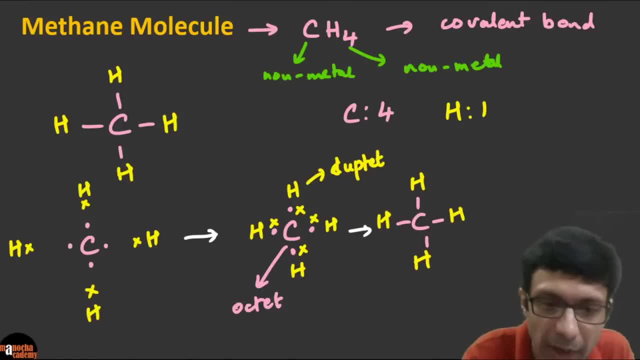 The sticks is representing a shared pair, Right, And so finally we have CH4.. Right, So you must write the last step. Also, we write the formula of the compound. So, very important, This is the formula of the methane molecule. 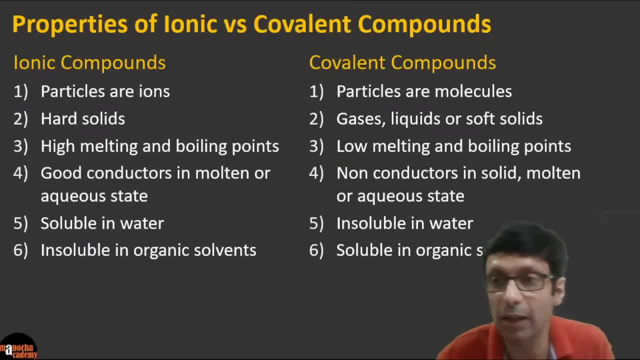 Excellent guys, Clear. Now let's talk about. we talked about the electron dot structure, Very important to discuss the properties of ionic versus covalent compounds. We've looked at these bonds and how to draw the structures So as we know that in ionic compounds, 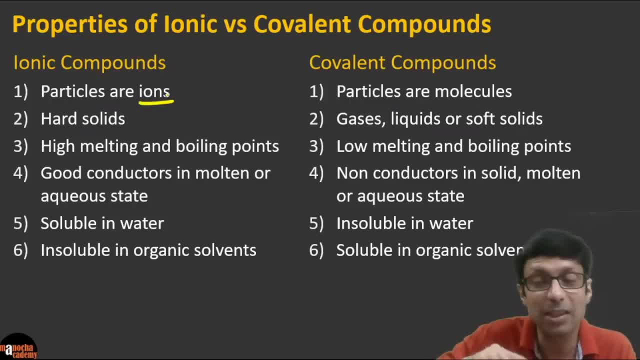 you know, the key point is the particles are ions. Remember there's a transfer of electron, So you have a cation and anion, OK. and the particles in covalent compounds are molecules, for example hydrogen molecule, H2O, water molecule. 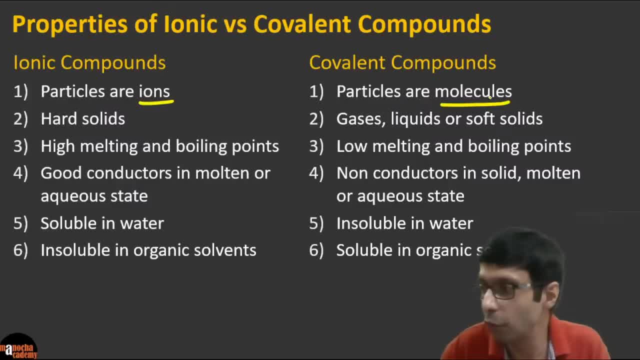 Right, OK, Then you have. So, for example, guys, I have this glass of water here with me, Right? So this glass of water, it contains water molecules in this glass of water, Right? What is a covalent compound? 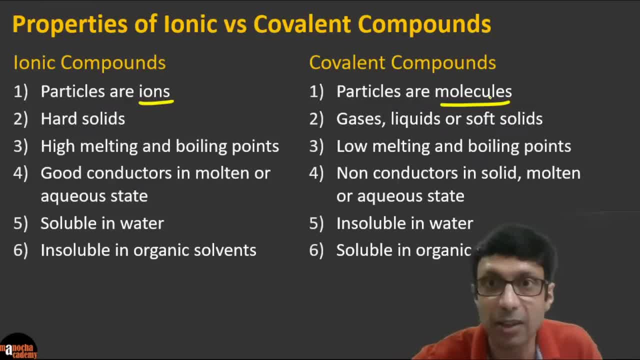 So it's having water Molecules present in it. The particles are not ions, They're water molecules. Right? What about this thing? The other properties- The other second point- is ionic compounds- are hard solids. Why? Because the strong electrostatic force. 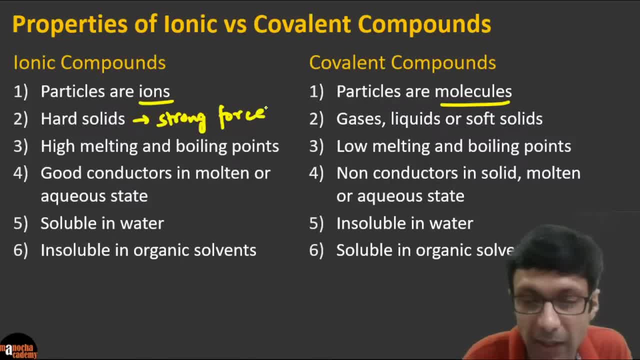 Right. So strong electrostatic force between the ions and these make them hard solids. like you know, sodium chloride is a hard solid, right, The salt. And if you take a look at covalent compounds, because these bonds are relatively weak, so these bonds are weaker bonds, right. 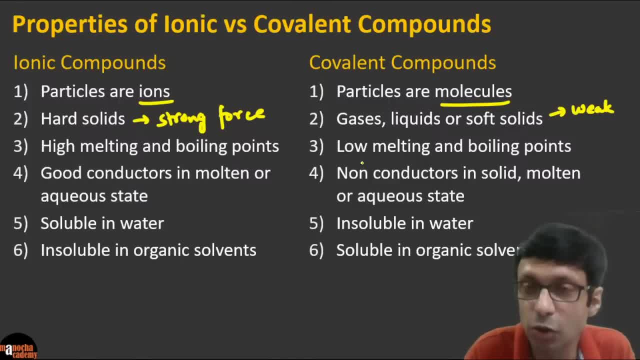 So very important property. because the bond is weaker, So it tends to form gases, liquids or soft solids. OK, can you see that? OK, let's take a look at the third point. because the bond is strong, Obviously they have high melting and boiling point. because you need a lot. 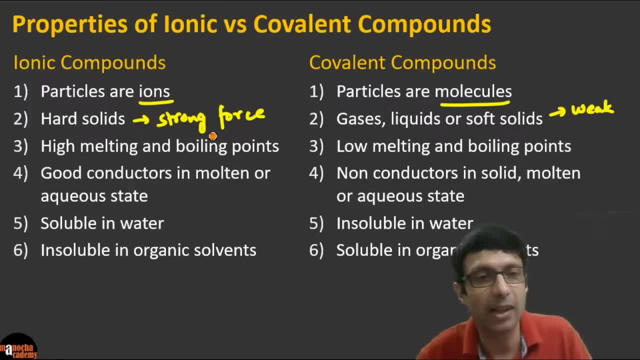 of energy, a lot of temperature to break down the bond, to melt it or to boil it. OK. And the next one? it has low melting and boiling point. If you take a look at covalent, on the other hand, it's the opposite, because weak bonds 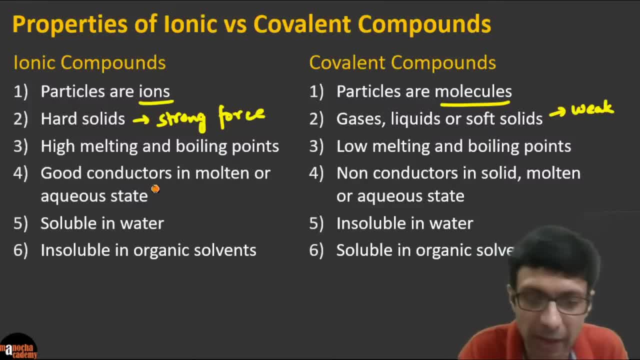 So they have low melting and low boiling points. OK, the next one, the ionic compounds. they're good conductors in molten or aqua state, because you know that when you take sodium chloride. So if you as a solid, they're not good conductors. 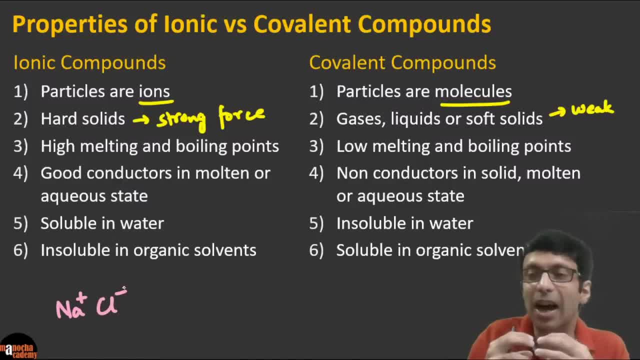 So it contains Na plus and Cl minus. right, Because the ions are tightly attached to each other, So they're not free to move, because for good conductors you want the ions to move, But when you have it in molten, OK, molten means in a. 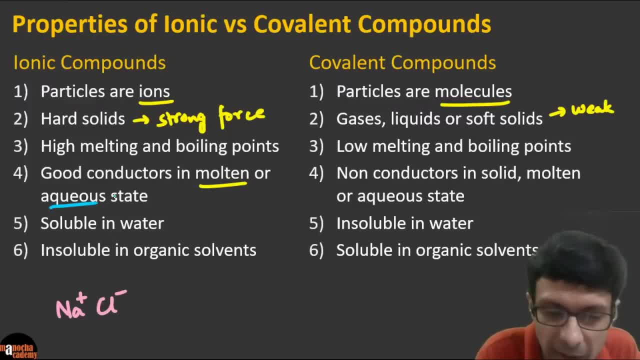 liquid state, when you heat sodium chloride enough, or in an aqua state, then these ions they break down. OK, and the ions become mobile, They're free to move And that is why they are good conductors. OK, the ions can move. 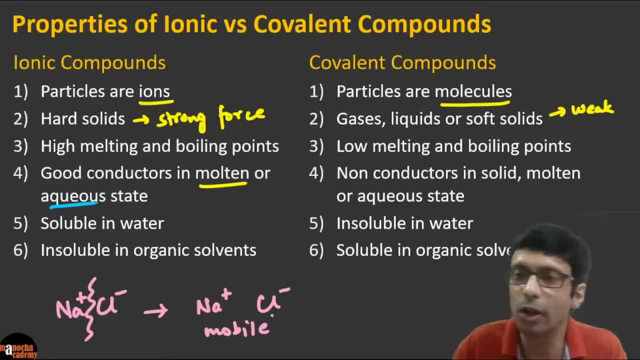 So that's the point. And then in covalent, these are non conductors in solid, molten or aqueous. Why? Because look at the first point, They are consisting of molecules. You know, you want ions charged particles for being good conductors. 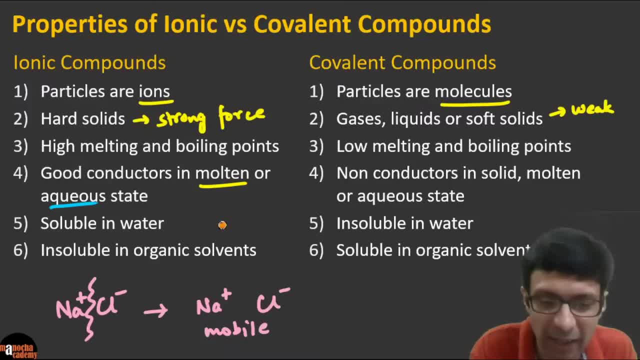 They are very important points to see. using common sense, You can get these ideas and you know you can remember the next point with an example: sodium chloride. It's an ionic compound and it's soluble in water. you know from the experience. 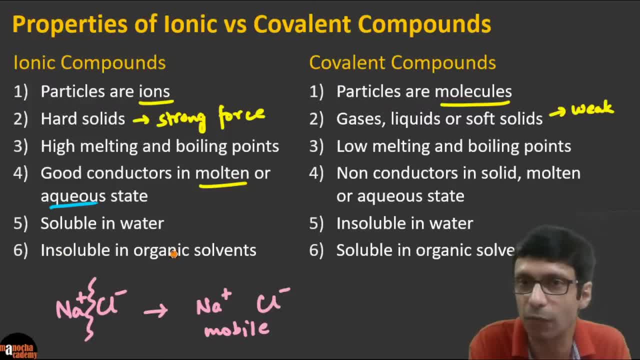 Right. So it's soluble in water, but they are insoluble organic solvents like alcohol or acetone- And usually again there may be exceptions, Right- And covalent compounds: it's the opposite: They are insoluble in water, but they're soluble in organic solvents. 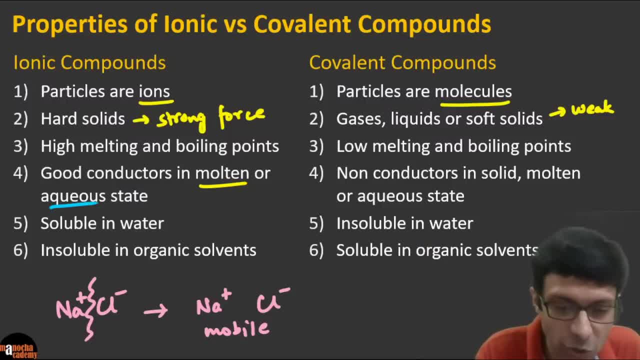 like alcohol or other organic solvents here. So this is very, very important And a lot of times you know, in the test they ask you to compare the properties And, as I suggested, read through the properties and think why. 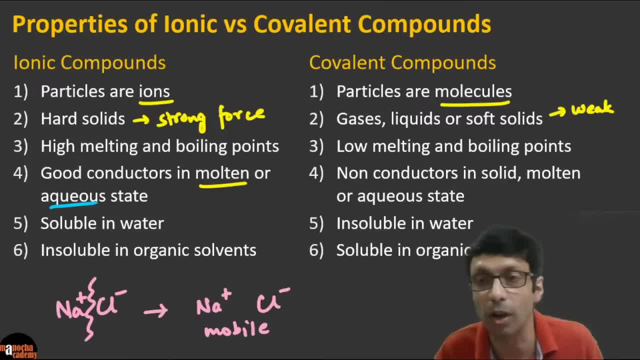 Why does it have a high melting point? Why high boiling point? Why is it soluble? Because of that strong bond, or because it has the particles contain ions? OK, And one very important thing. Remember ionic compounds, what we learn. it's formed between a metal and non metal. 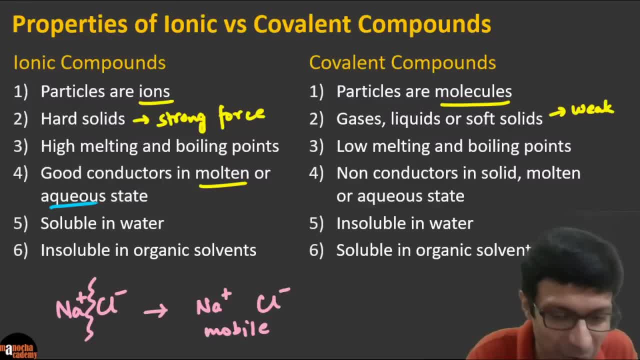 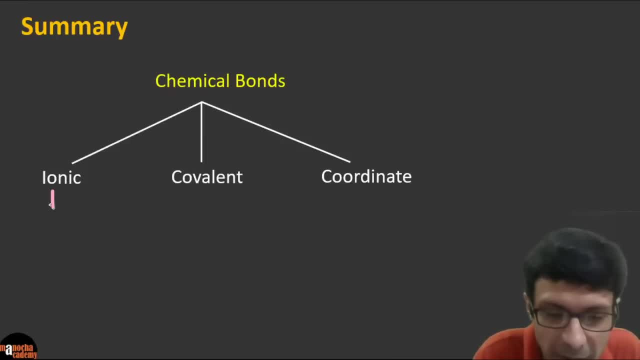 Covalent is formed between non metal and non metal, Right guys? So here's a summary of what we learned today. So ionic or electrovalent bond, what is the key point? This is due to transfer of electrons. OK, 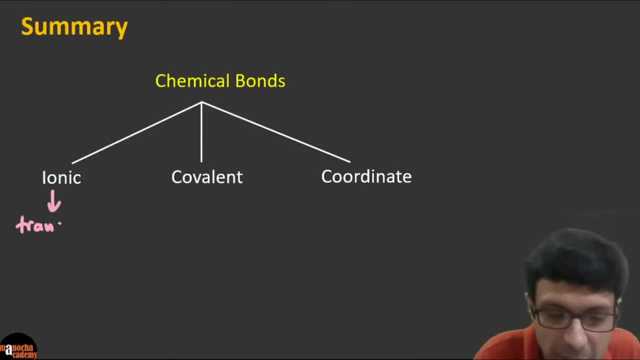 So it is. these bonds are formed by the transfer of electrons- Very important point, OK, And transfer of electrons. And it is formed between a metal and a non metal. OK, Please remember that. this is the key takeaway. And what about covalent compounds? Right? 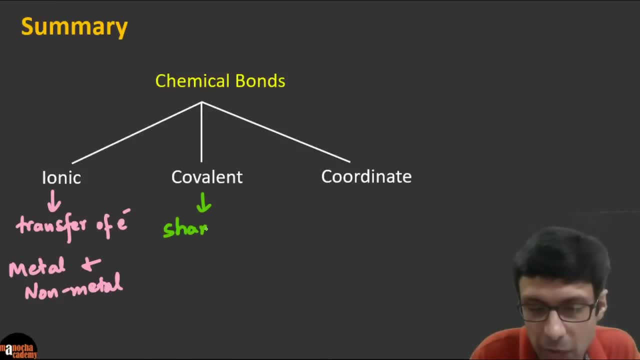 So, covalent compounds, you know, they are formed by sharing- sharing of electrons, OK, And this is formed between the sharing of electrons, Right, And formed between non metal and non metal. OK, So that was metal and non metal. 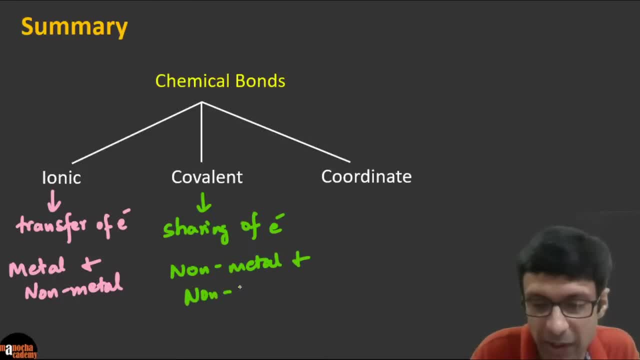 Here you need non metal and non metal. OK, It's for covalent bonds and coordinate, which we didn't talk about today. OK, We are out of time and I knew we wanted to do ionic and covalent in detail. 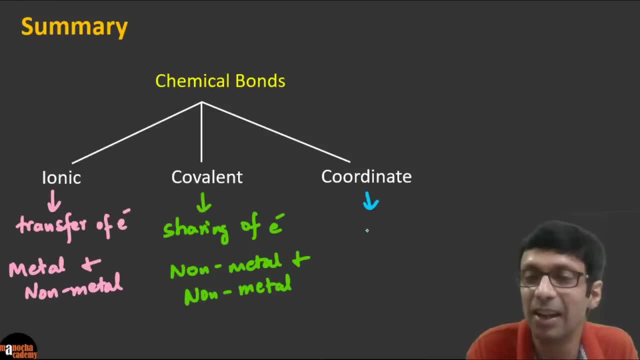 So covalent in coordinate bond or data bond is again, you know, sharing of electrons, But the shared pair comes from one Atom only. so shared pair of electrons from one atom, only one atom, only Right. And there are examples like, for example, the ammonium ion. 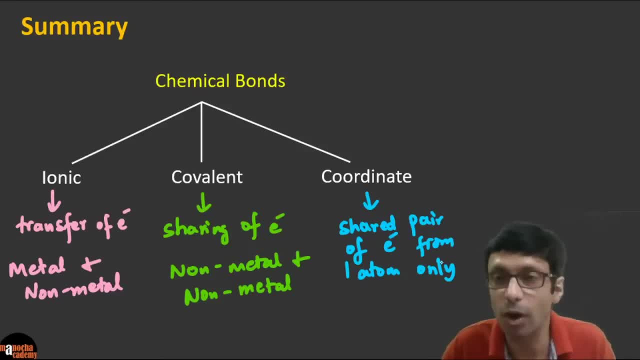 OK, so you can explore that on your own. So here's a summary of what are the three important things And, as you saw in the class, we talked about the first, the most two important: ionic and covalent bond. OK, And guys, I have a question for you. 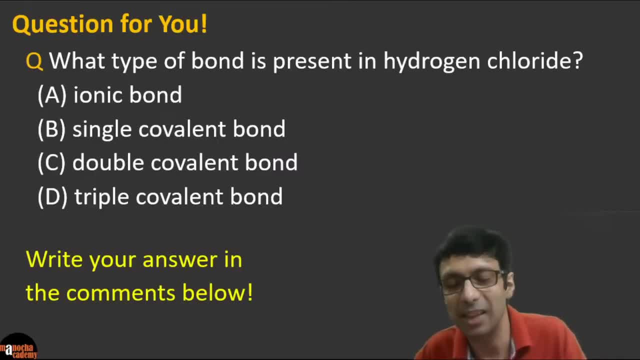 So for all of you to try what type of bond is present in hydrogen? And again I would tell you guys, the hint is be James Bond. Think carefully, Right, Think of the rule that we learned today and do let me know your answer by putting. 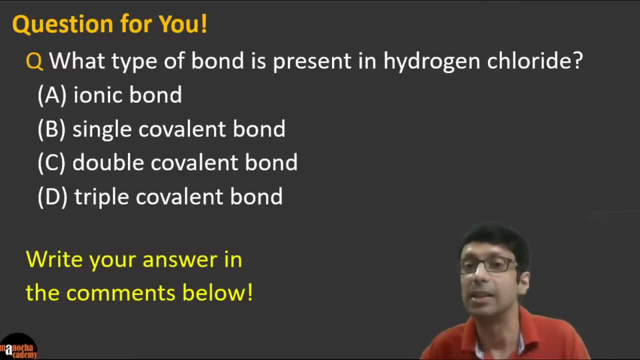 it in the comments below. So is hydrogen chloride an ionic bond, a single covalent bond, a double covalent or a triple covalent? And, guys, I look forward to reading your comments. So, guys, please do write it. 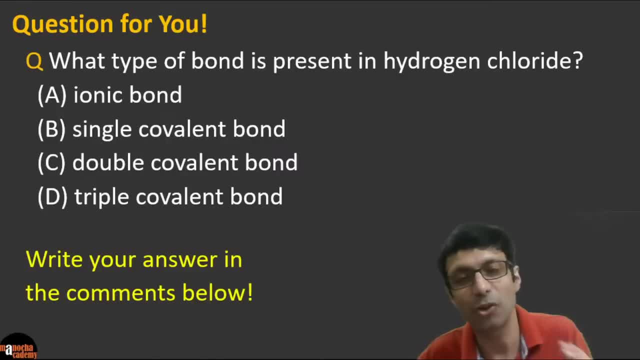 in the comments below and some of you write it really fast And I'll try to respond to you guys as soon as possible. It's great to see the response And you guys were awesome in today's class. Great to see so many likes and such excellent participation. 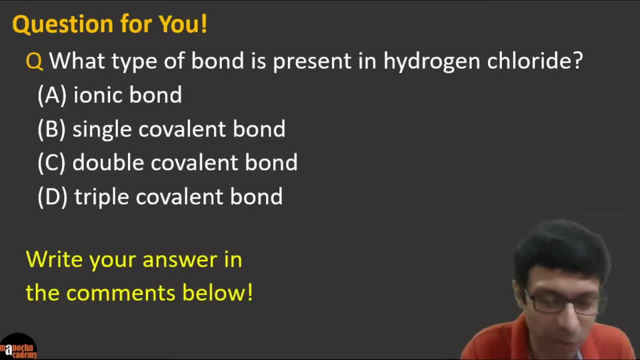 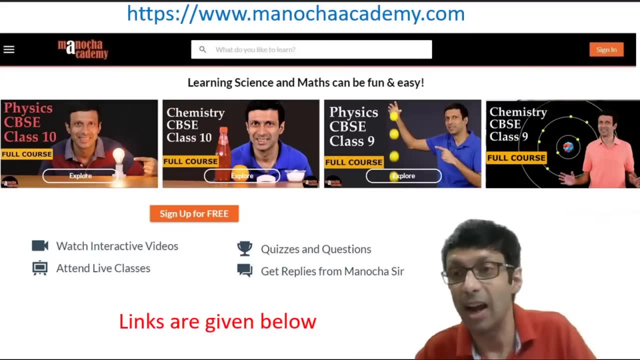 I know a lot of you requested this chemical bonding topic, So here I am with that topic And, guys, if you haven't checked out our website, do check it out: Manochacademycom. A lot of people have taken the course and I'd like more of you to take it, because 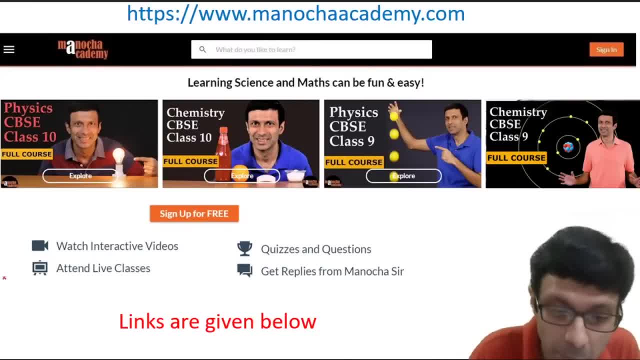 these courses will really help you in your preparation. We have- I take- more live classes on our website, So if you're excited about these live classes, come and join us. These courses are at a very discounted price. You know. we've not kept it at a high. 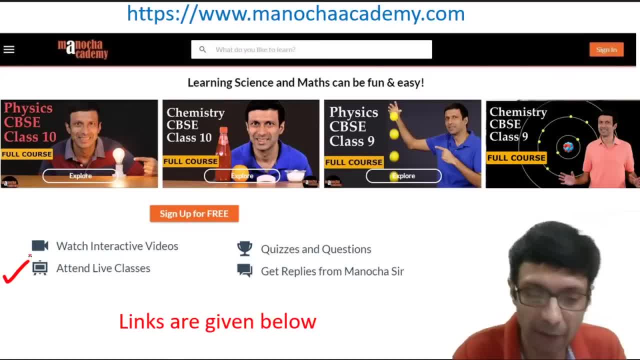 price so that everybody can avail of these courses, and they have interactive videos. We have more live classes where we discuss more detailed concepts. I show you the tips and tricks on how to solve the questions. You know we have quizzes and questions and then you get your replies to the doubts from me. 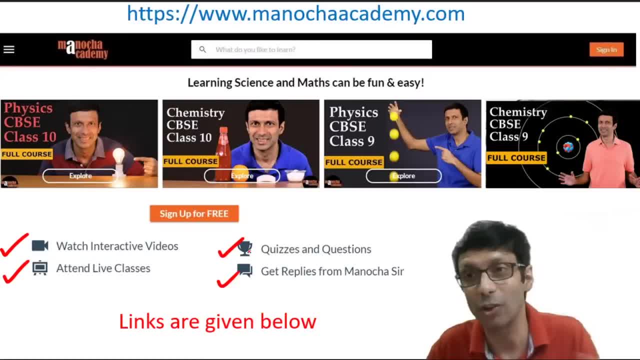 So guys do check it out on physics, chemistry and maths and we'll try to launch more courses because we've been getting more requests. So thanks a lot for your support, guys, And to share out our channel with your friends. 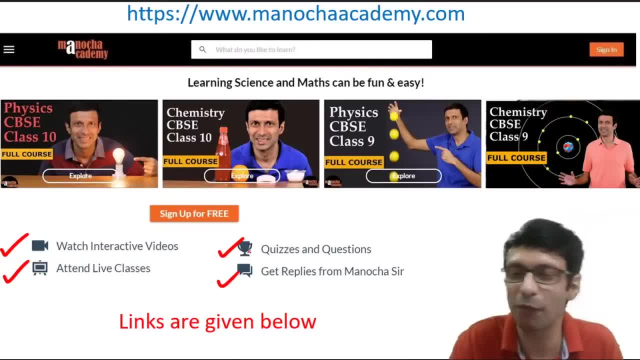 And if you Haven't hit the subscribe button, please hit it right now. Click on the notification bell so that you don't miss a single live class that we have on YouTube or any of the videos that we upload. So, guys, do check it out. 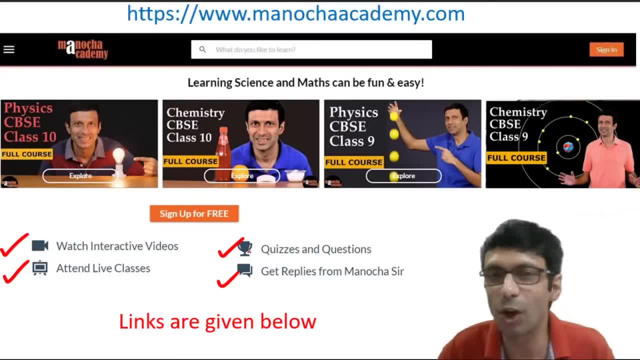 And, as I said, if you want more live classes, please go to Manochacademycom. The sign up is free. We have some free samples out there, So do check it out And if you like it, you can take the course.